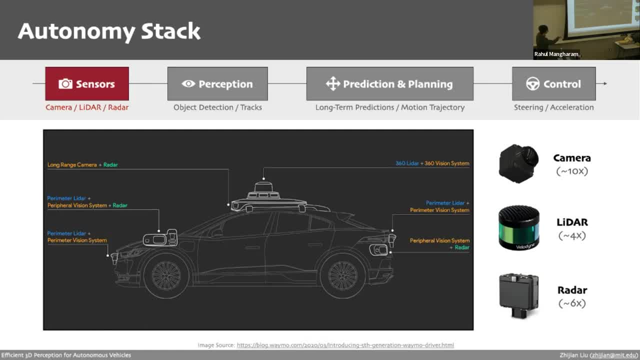 there are like 360 LiDAR and vision systems And also there are radar sensors like all around the car and also their primary vision system and the LiDAR system as well. So on the Waymo driver, there are in total four LiDAR sensors. 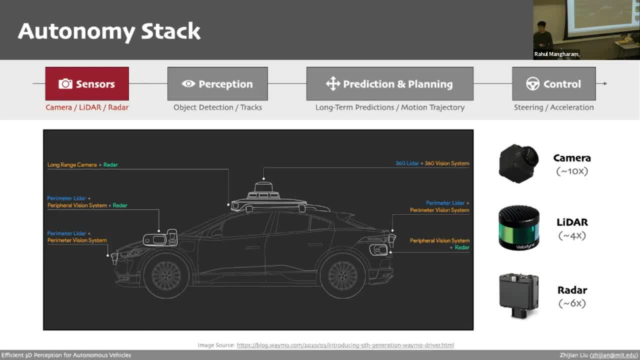 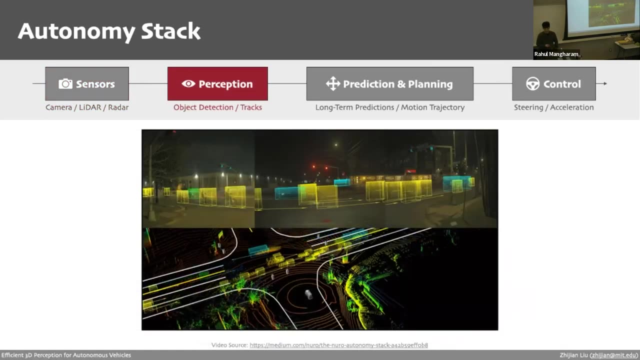 10 camera sensors and six radar sensors, So that's a lot. These sensors can actually provide different kinds of information, and the different sensors of the same kind can also provide a better coverage of the surrounding of the car. So, after collecting the information from the sensors, 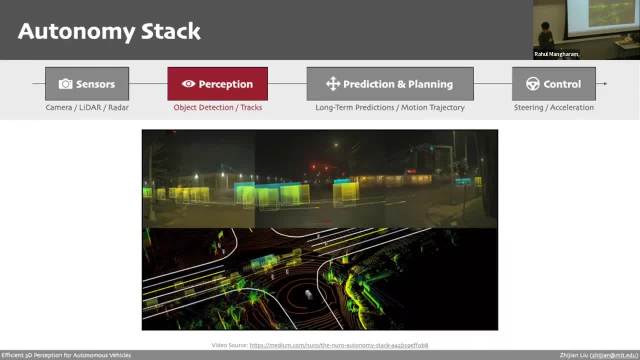 the system then goes to the perception module. So here it has to understand like what's going on around the car, for example, to recognize all the other cars and people and understanding the layout of the scene. So it's actually a very challenging part. 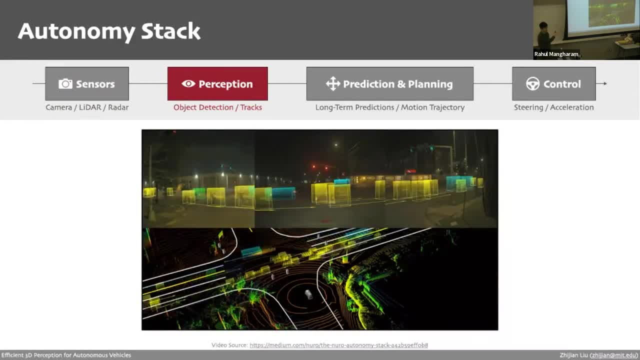 because you can see, for example, here there are a lot of moving cars that are actually very far away from the Eagle car And also it's very hard to recognize them because of the low light condition here. And that's your perception of the system. 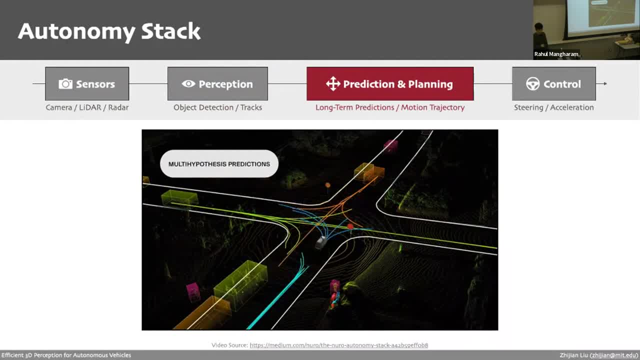 moves forward to the prediction and the planning module. So, based on how other objects have moved in the past few seconds, the prediction module will estimate how they will move in the near future, let's say, like in the next 10 seconds. And it's actually also very challenging. 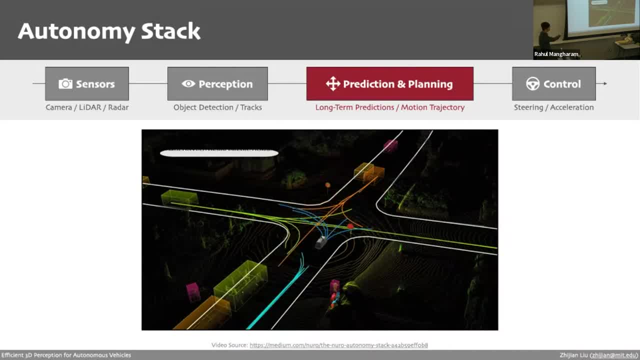 because the future can be uncertain. For example, like very closely intersection, the car can actually either go straight or actually turn left or turn right. So the planning module has to take all these possibilities into consideration and then plan the movement accordingly in order to drive safely. 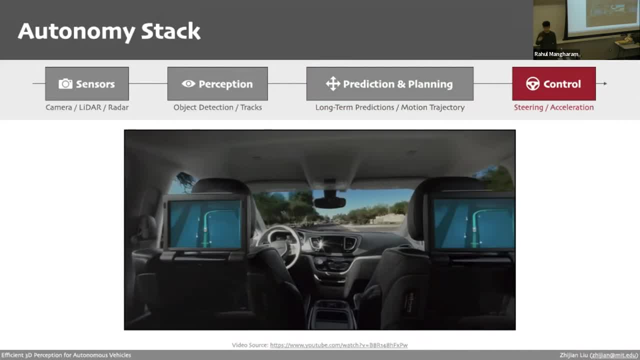 And the final step is the control modules. So it basically takes the plan trajectory and maps it into the action by actually controlling the steering wheels and acceleration. So I hope this gives you a very quick glance of how autonomous vehicles work. So in this lecture 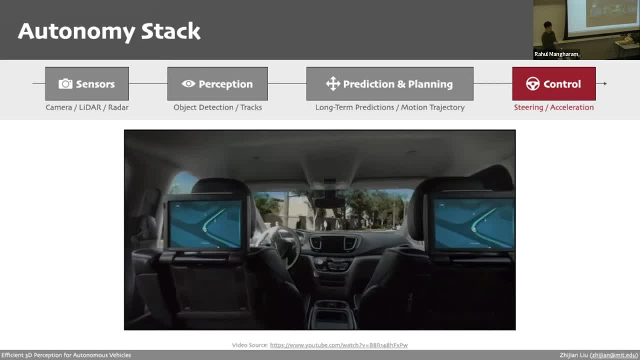 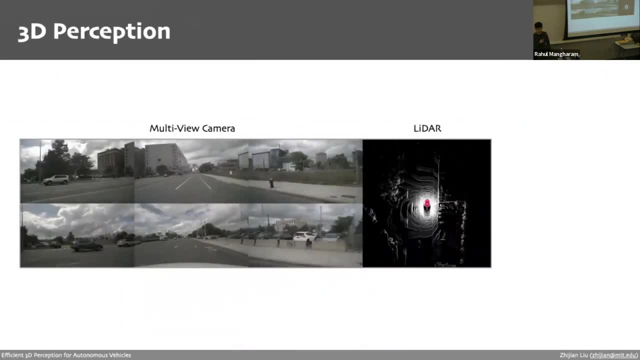 we'll be mainly focusing on the second component here, the perception. So we're more precisely, we'll be focusing on the 3D perception. So what is 3D perception? The input to the 3D perception is the sensory data. 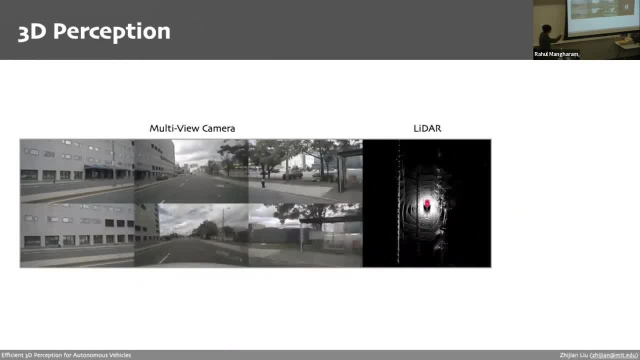 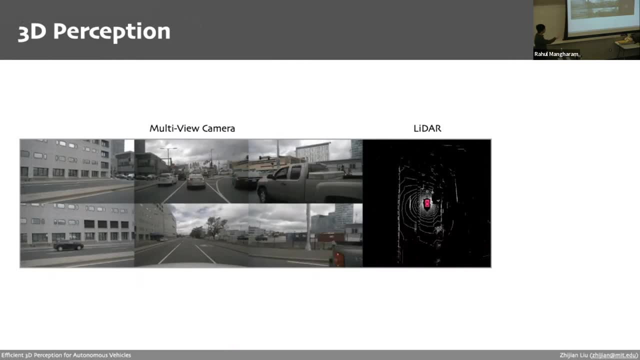 For example, here we have the multi-view camera, images from multi-view cameras here and each having different orientations, for example, some of them heading front and some of them heading back and left and right. We also have the light of point out here. 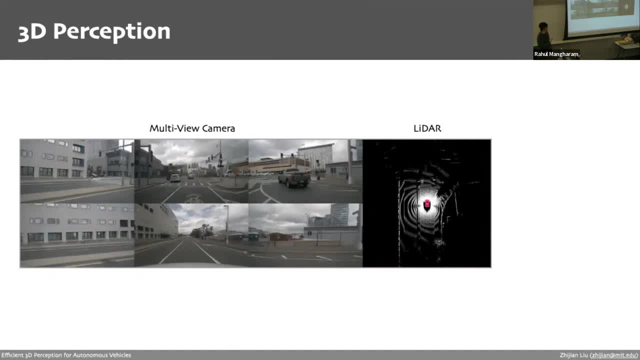 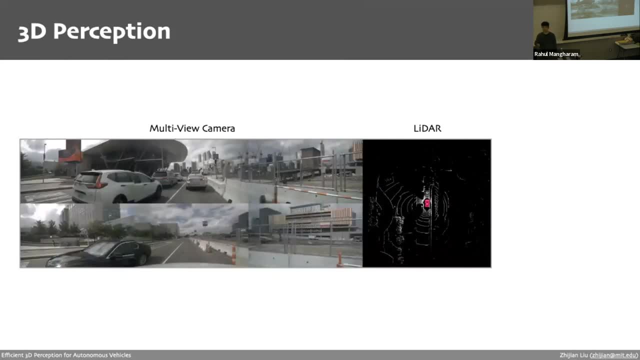 So here I projected into the top-down bird's eye view for visualization purposes. So, based on these inputs, the goal of the 3D perception is to understand the surrounding environment, For example, to do the theory of the detection to protect all the other objects. 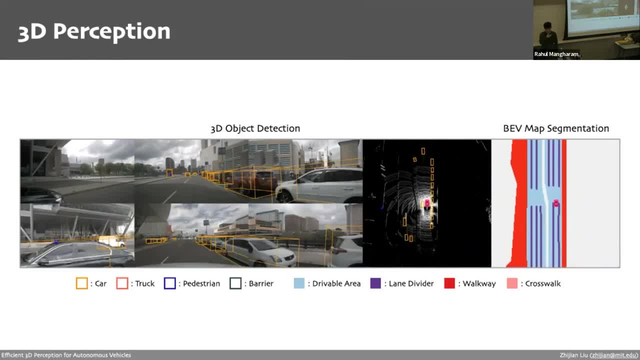 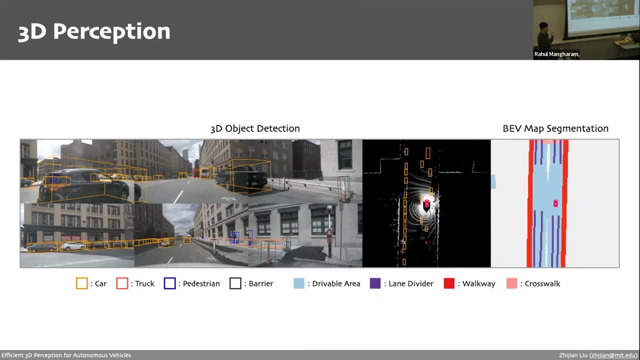 in the scene, such as the cars, cars, pedestrians here. So these detections have to happen in a 3D space, because we care not only about these objects where they are, in the 2D images. also we want to understand how far away 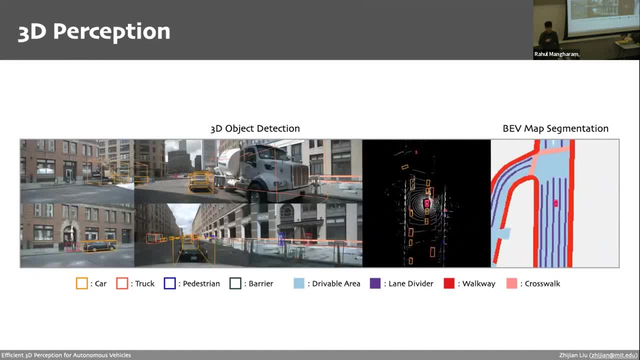 are they from the eagle car? And in addition to detecting these dynamic objects in some places where we don't have the high definition map, we also want to like pause the semantic layout based on the perception data. So that's probably a map. second patient: 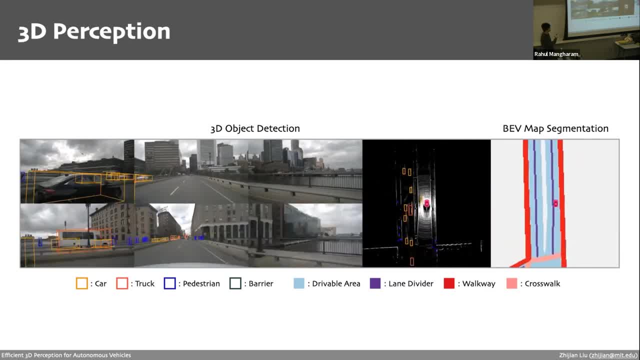 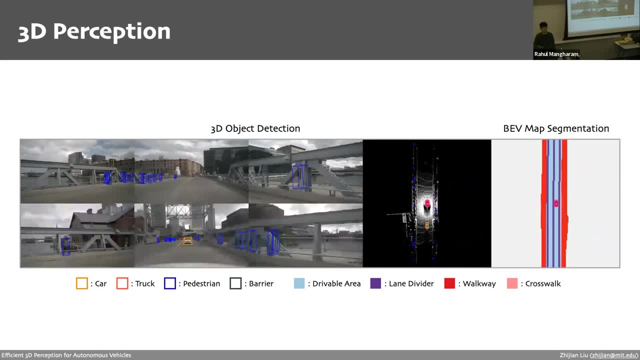 So here we need to pause to travel area, the link divider, and the other like semantic causes as well. So how can we achieve the 3D perception? So nowadays all the 3D perception systems are mostly based on like a neuron. that was deep learning. 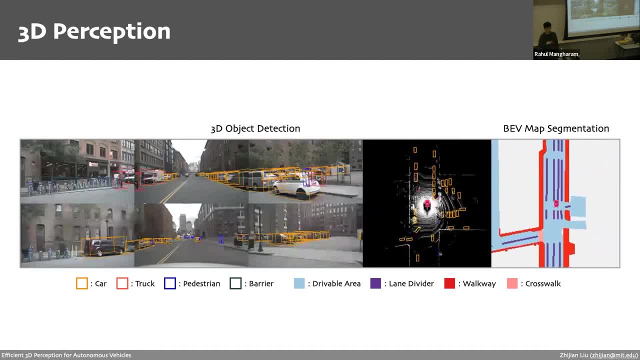 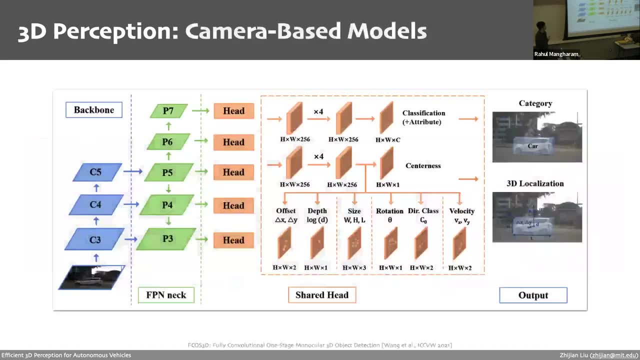 So I will first briefly go over two of the very classic 3D perception models. One is a camera-based model, this one is a light-up based models. So first let's take a look at the camera-based 3D perception model. here it's called FCO in 3D. 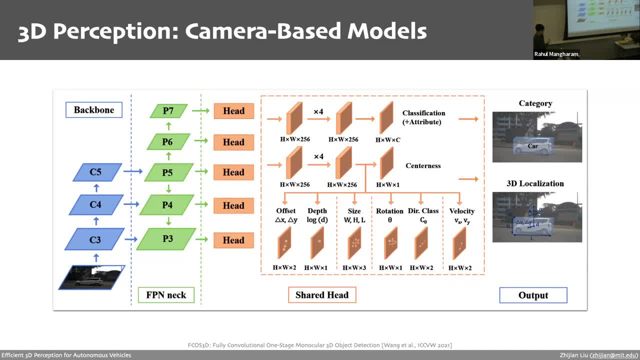 So you can see the overall structure is actually very similar to the 2D detection models. For example, we have the image backbones at the very beginning and then we have the feature pyramid network to extract the multi-scale features to cover objects with different sizes. 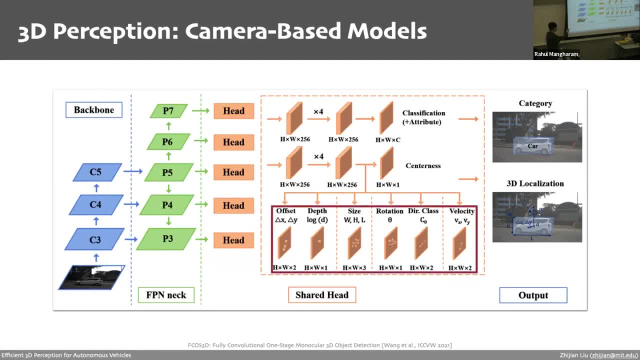 The major difference here from the 2D detection is actually at the hat. You can see, here we're only care about the 2D offset, the 2D locations of the car. You also want to request the tabs, the 3D dimensions of the box and also, like you know, 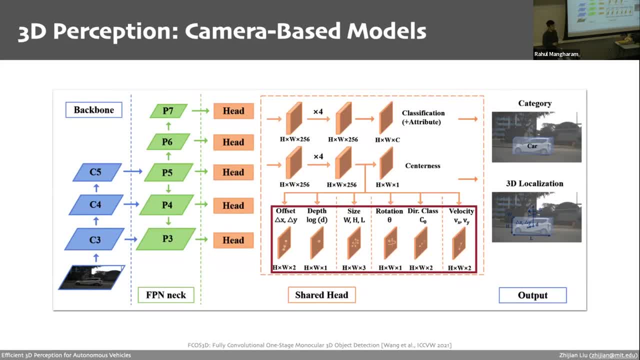 the 3D dimensions of the car, The orientations and finally the velocity. So velocity is actually very important because it's used in the motion prediction stage to help the system understand, like the movement of the car. And then this is the light-up 3D perception model. 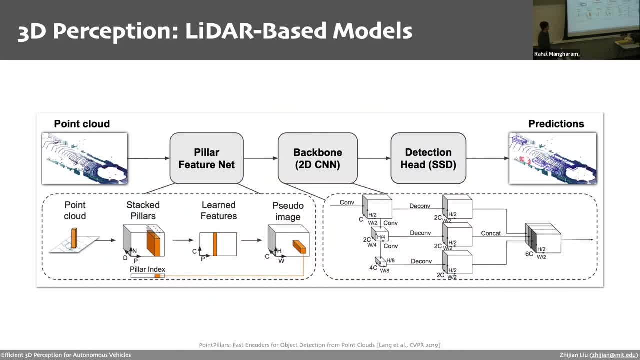 it's called point pillars. I think it's actually covered in the previous lecture. So most of the 3D perception model follows basically the same paradigm. So we will first use a 3D encoder here to extract the 3D features. 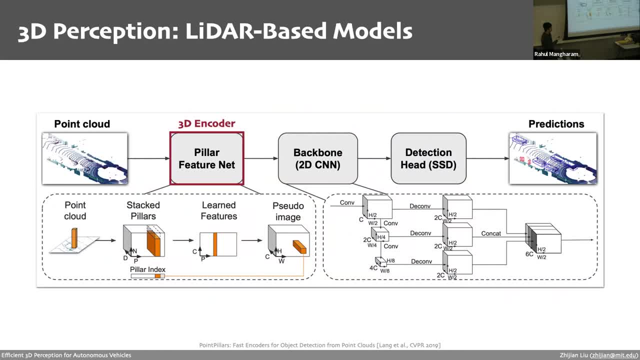 And then you will project the 3D features onto the first-eye view- a 2D map. So oh, by the way, here the 3D encoder they're using is very similar to a point map. It's less powerful than the sparse convolutional models. 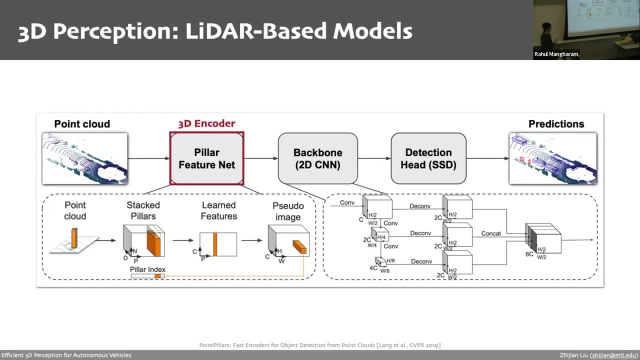 I will introduce later, but it's actually like more friendly for the deployment So they can be easily deployed using TensorFlow, RT and other acceleration libraries, And then for the BAB feature map, because this is in 2D so you can use any 2D platforms. 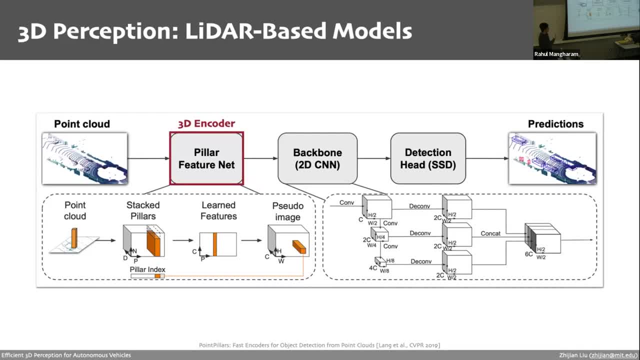 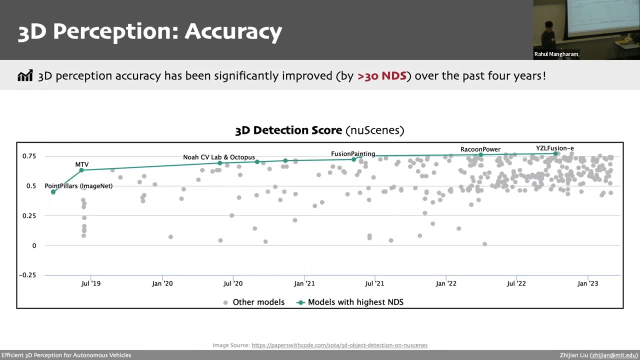 and detection hats to process it. For example, here they're using a multi-scale backbone and also using SSP as your detection hat. So with the development of the deep learning and neural networks, we have actually observed a huge improvement in accuracy of the 3D perception model. 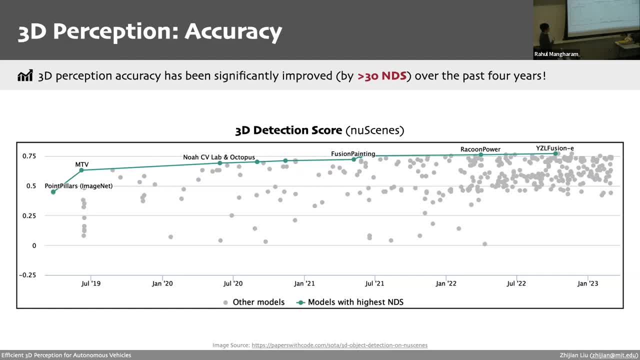 So here is the trend of the 3D detection score. from the new things leaderboard We can see that the very first method here actually is 0.2. as we just introduced, It only achieves around 45%. like new things detection score. 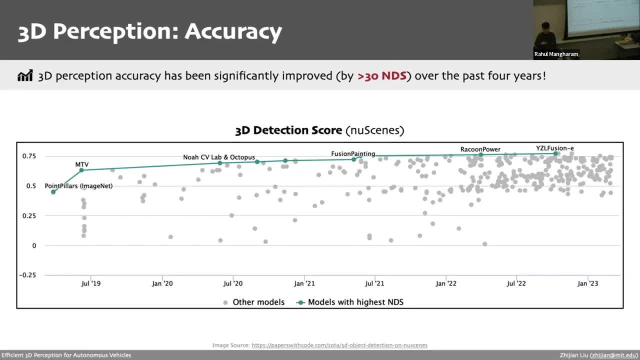 Over the past four years the detection accuracy has improved from 45% to about 75% here, So that's 30% absolutely improved. We are also witnessing more and more methods on the coming on each week actually on the leaderboard. 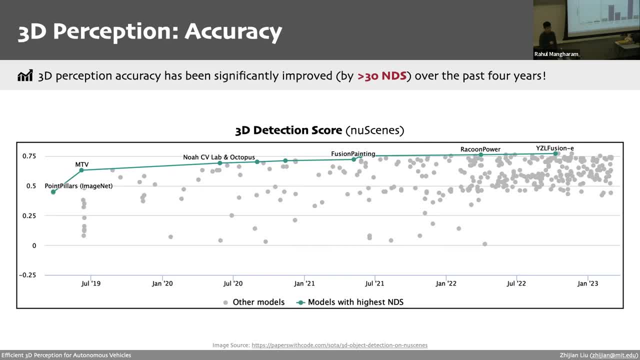 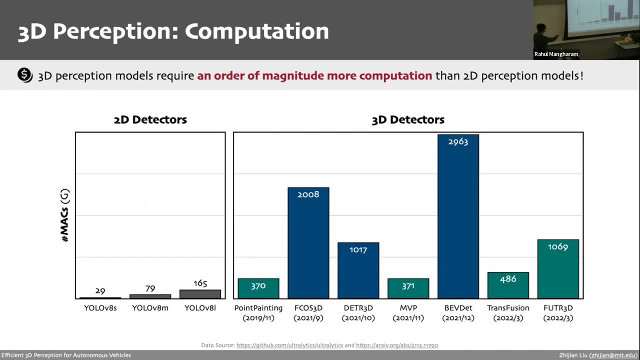 It's a very fast evolving direction. However, the improved accuracy comes at a cost of increased computation. So on the left-hand side we have the latest YOLO V8 series, So that's a very popular, efficient 2D detection models. 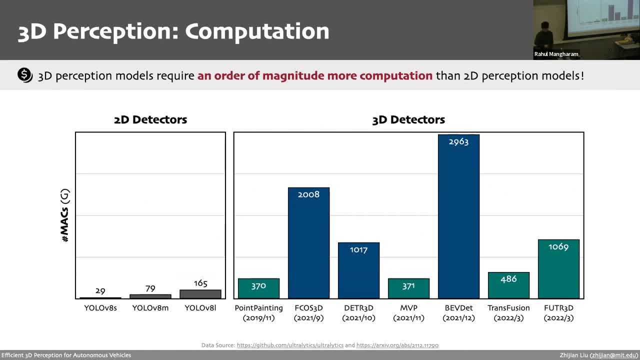 targeting real-time deployment, So you can see they're actually very efficient. While on the right-hand side I listed a few representative 3D detection models in the chronological order, For example, the point-painting, FCOS and the latest transfusion and filter 3D. 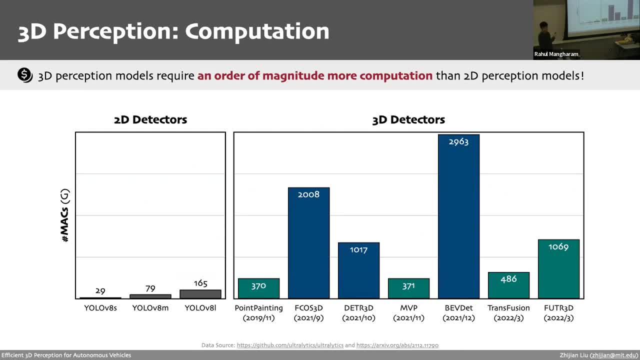 So we can see a clear gap in the computation between the 2D and 3D detectors here. The 2D detectors consume around 200 Gmax, while for some camera-based 3D detection models like DVTAD, they're actually taking like 3T max. 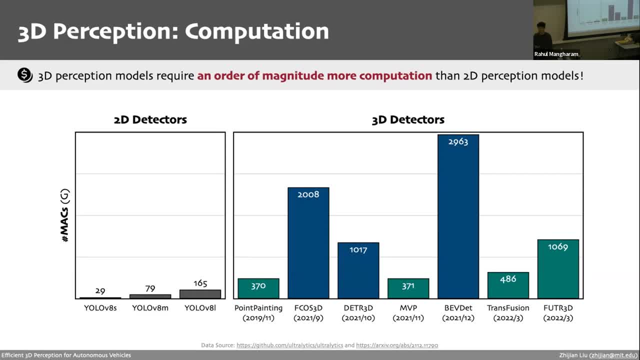 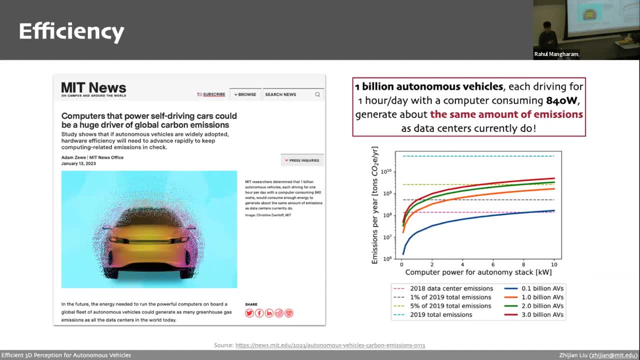 So that raises a huge challenge on the efficiency side of the 3D detection models. So that comes to the third key word of this lecture: efficiency. So one reason why we care about efficiency is also like the computer is powering the cell. 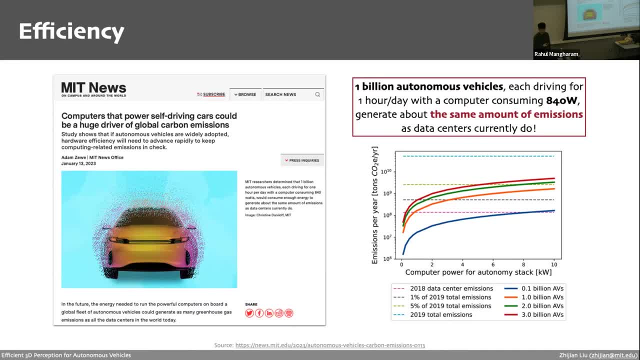 and the self-driving cars could be a huge source of the carbon emission, So that's why we care about its efficiency. But this is the latest article from the MIT News, So a group of MIT researchers identified that the computers. so if we have like 1 billion autonomous vehicles, 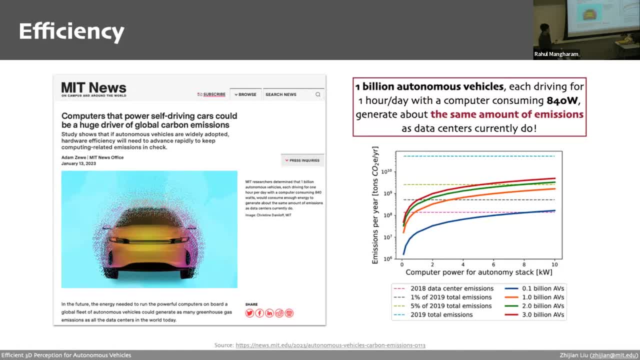 and each drives for like one hour per day, and if it's mounted with a computer consuming like 840 watts of like energy, you can see its carbon emission is around the same as the data center currently do. So you can also see from the curves here. 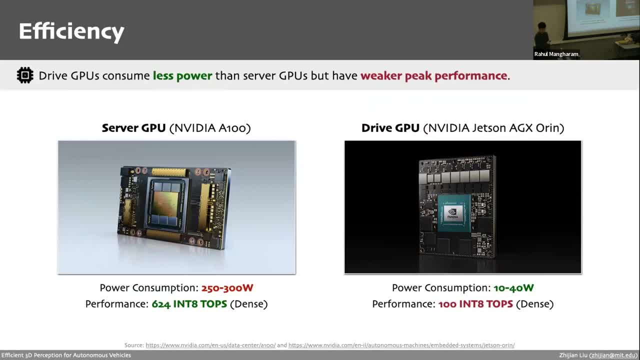 So because of this, the drive GPUs are actually usually more energy efficient than the server GPUs. For instance, a popular drive GPU here, the NVIDIA Justin AGX-R. it consumes only 40 watts of energy, So it's around seven times lower. 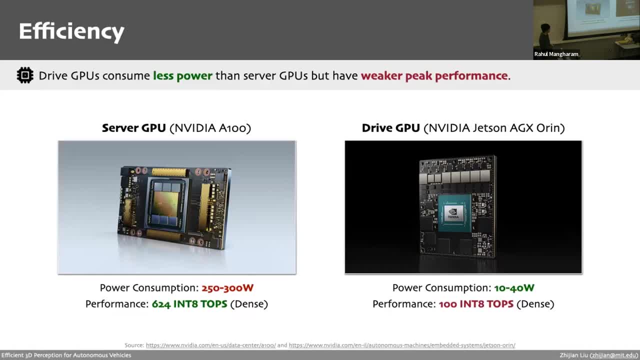 than the server side GPU of the NVIDIA A1 engine, But it also comes at a cost right, So its peak performance is also weaker than the server side GPU. For example, its peak performance is only 100 into 80 ops, while the server GPU A100 is like six times more than that. 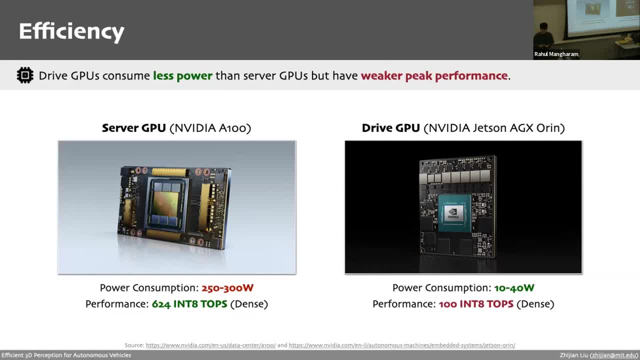 So, like the limited computational resources we have on the car, also motivates us to design more efficient 3D perception algorithms. So that's actually the focus of this lecture. So for the rest of the lecture, I will start by introducing the BV Fusion. 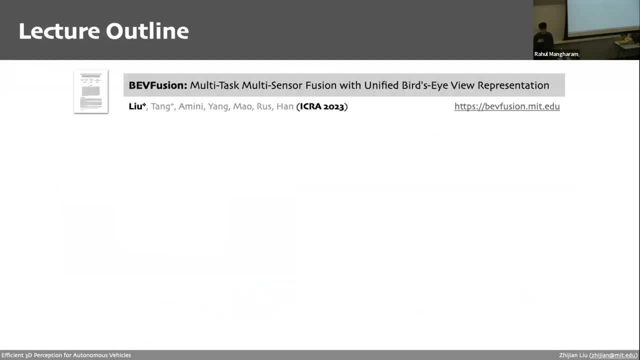 So it's a 3D perception framework that can efficiently, you know, be used in the future. So it's a 3D perception framework that can efficiently, you know, be used in the future. It supports multiple sensors and handle multiple different 3D perception tasks. 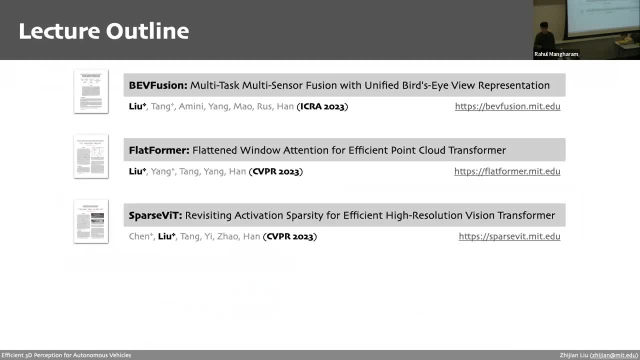 And next I will give you a brief overview of our latest works: Platformer and SparseVIT, So they're accelerating the LiDAR and camera encoders in the 3D perception models. And lastly, I will demonstrate how we have deployed 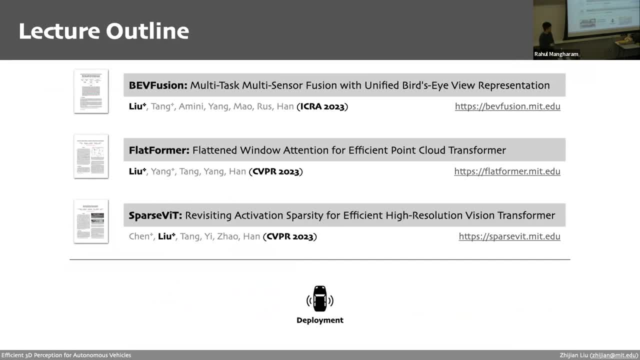 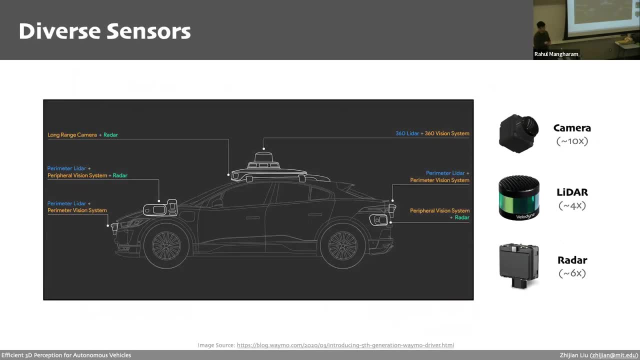 our work in autonomous racing vehicle and also on a full-scale autonomous car. So let's begin with the BV Fusion, As I had mentioned earlier. like self-driving cars are equipped with numerous sensors, each with distinct types and also distinct orientations. So the three most commonly used sensors are the LiDAR. 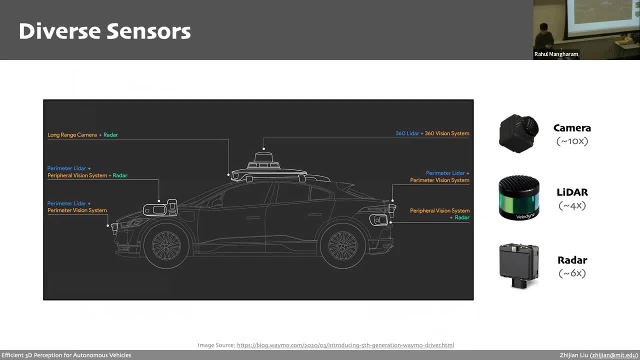 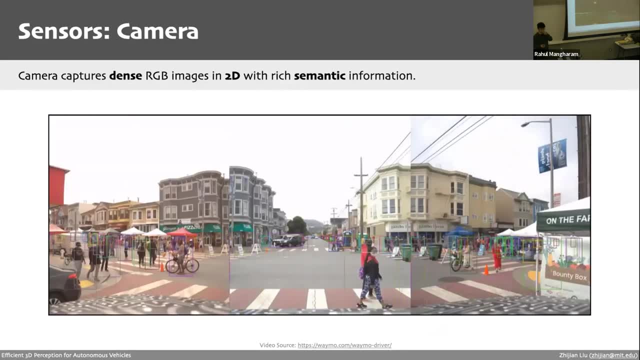 camera and radar, So we'll first go over each one of them. So cameras are probably the most familiar sensors to all of us because we are using them on a daily basis. So they capture the dense RGB images in the 2D space. 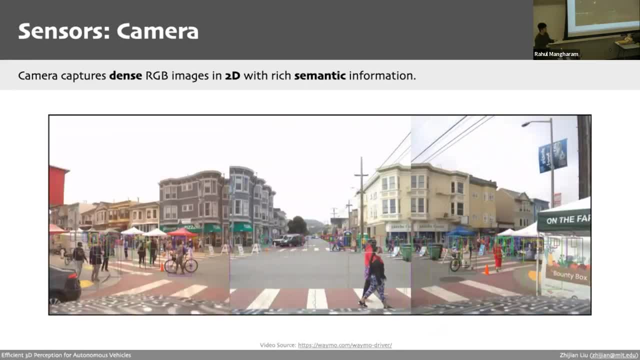 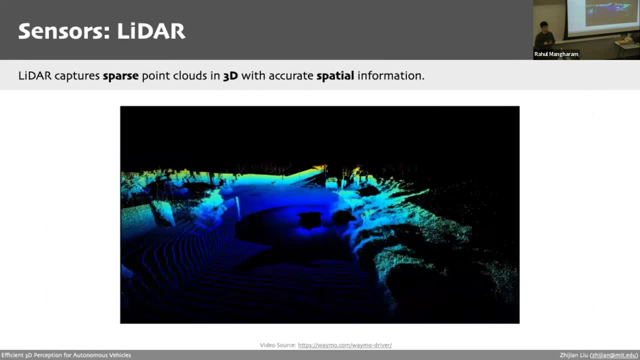 which can capture rich semantic information, for example, the color and texture of the environment and the other cars. LiDARs, on the other hand, capture data in the form of a sparse 3D point cloud which essentially is a set of points- XYZ coordinates. 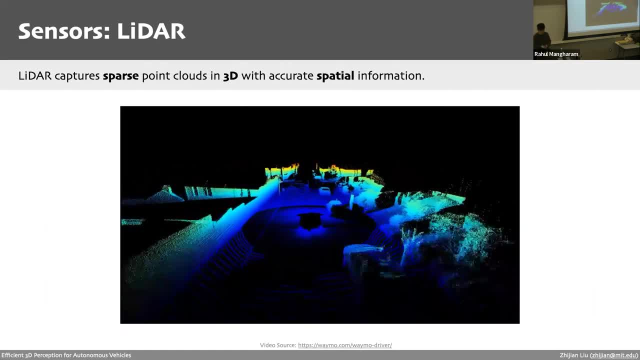 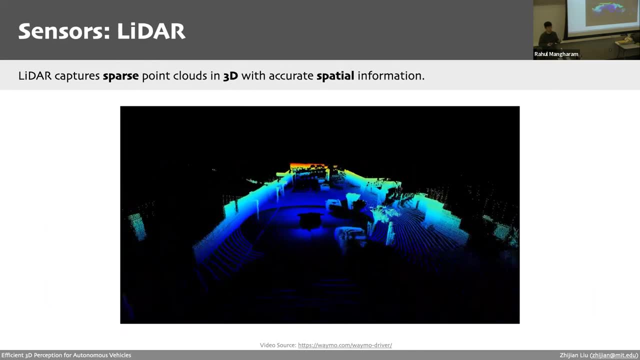 and sometimes they also have some other features like intensities. So, as the data is in 3D, the LiDARs can provide very accurate spatial information about the distance of each point to the ego part, which can be crucial for the 3D detection task. 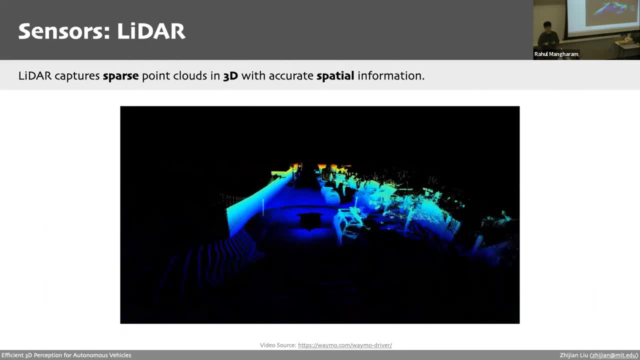 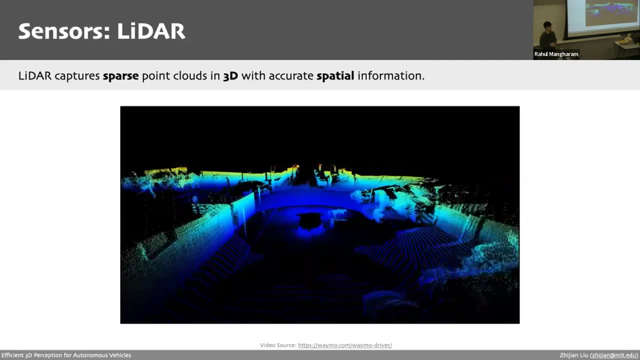 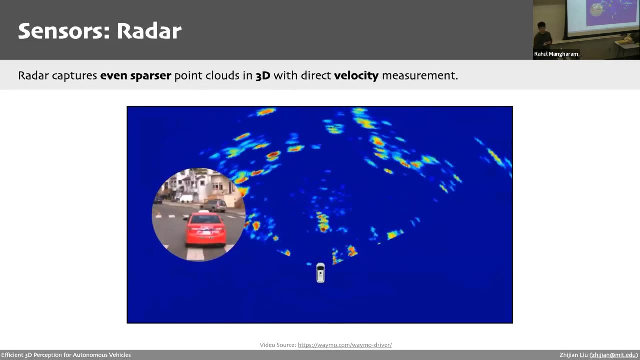 And this type of sensor has also become more accessible in the past few years. For example, the latest generations of the iPhone Pro actually has also equipped with the LiDAR scanners, which is underneath the camera sensors, And finally, the radars are kind of similar to the LiDARs. 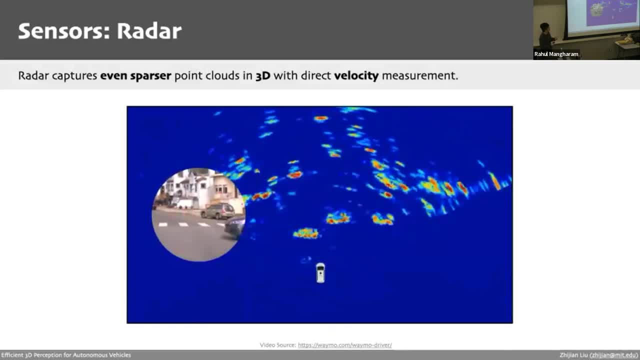 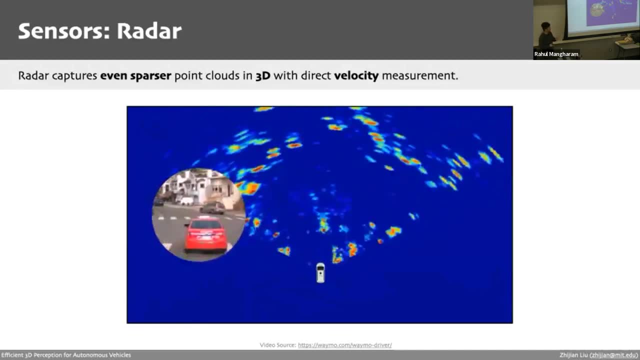 in some ways They are also capturing the data in the sparse point cloud format, in the 3D or in the bird's eye view space. So there are two main difference between the LiDAR and radar data collected. The first one is the data collected is much sparser. 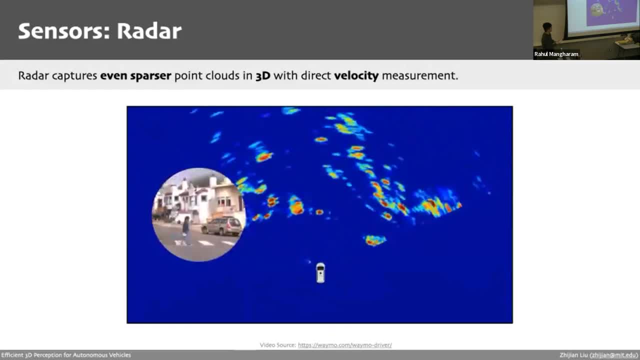 than the LiDAR point cloud and also it's much noisier. And also another thing is that the radar can directly measure the velocity of the other objects. That could be very useful if you are going to estimate the velocity of the other moving objects. 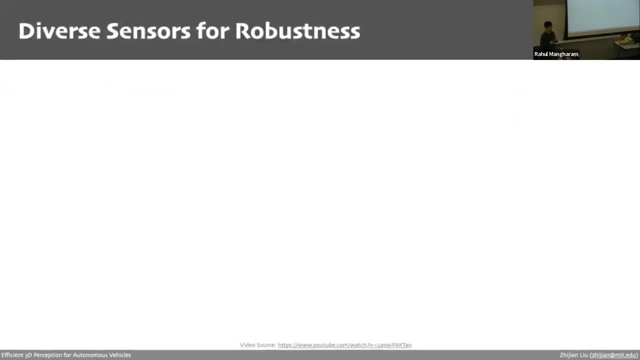 So different sensors have distinct properties. Some of them are like focusing on capturing magnetic information, Some of them are capturing like spatial, spatial information and some capturing motion. So using a variety of sensors can also improve the robustness of the screen detection system. 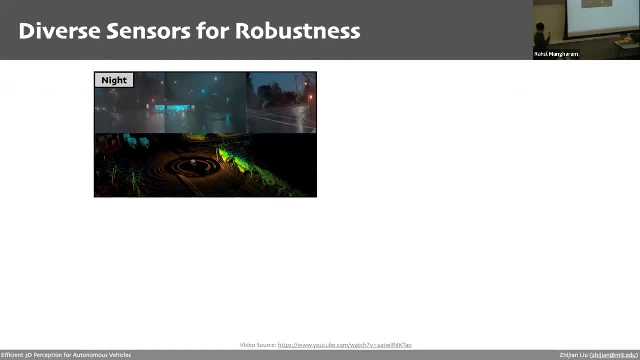 For example, the camera sensors are not very robust in lighting condition. You can see from this visualization here: during the nighttime the camera sensor can barely provide much useful information, While during the daytime the direct sunlight can also cause overexposure. 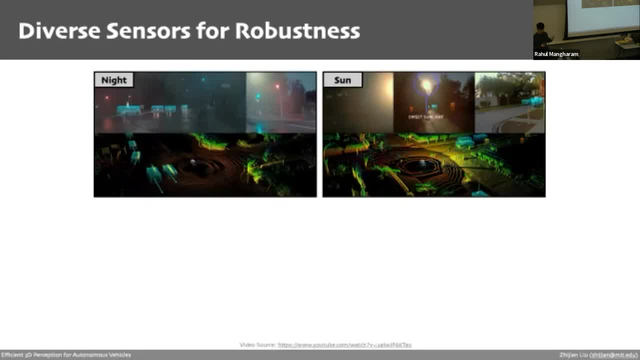 which also makes it very challenging for the camera sensor to capture anything. LiDAR sensors, as you can see on the bottom of the two visualizations, are less effective. to try the lighting conditions, However, the LiDAR sensors are not very robust. 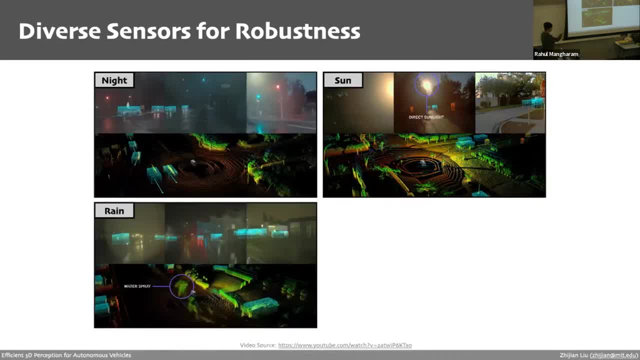 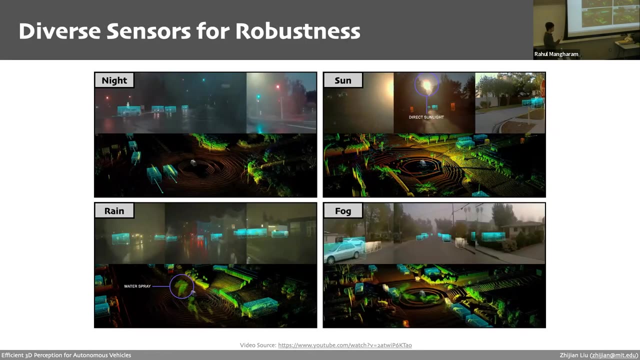 in some weather conditions, For example here you can see, in the rainy days- the LiDAR sensors will capture the water sprays in the beta as well, which might actually confuse the three perception systems and generate some positive predictions, And the same applies to the foggy days. 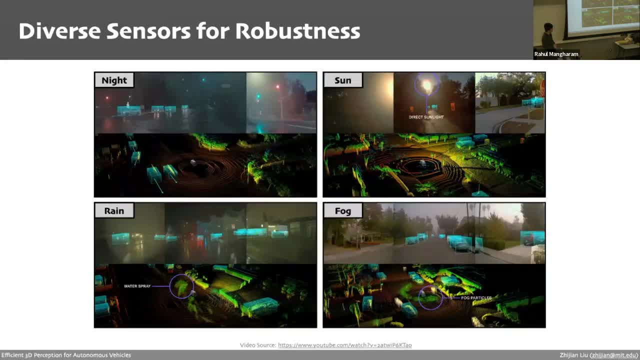 You can see that the fog particles can also generate some noise in the beta, But in these two cases the camera sensors are kind of less effective and radar is actually very robust in different weather conditions. So therefore fusing information from diverse sensors can help us avoid a single point failure. 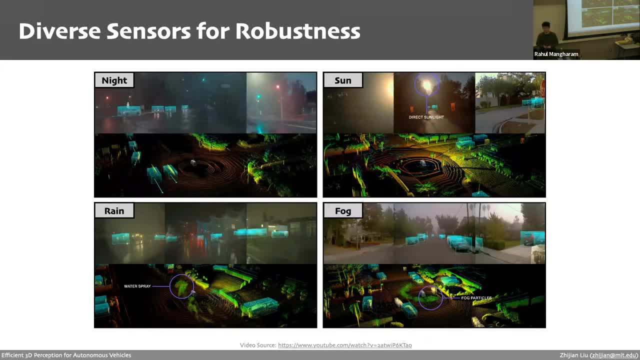 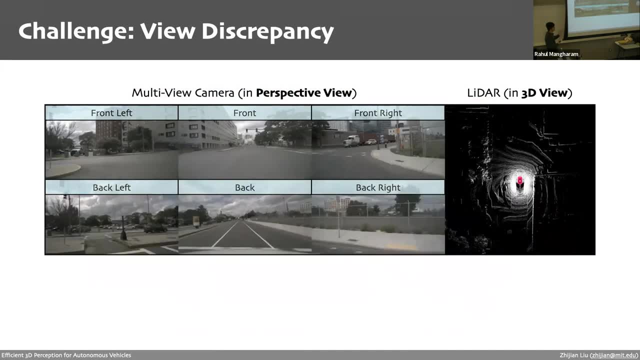 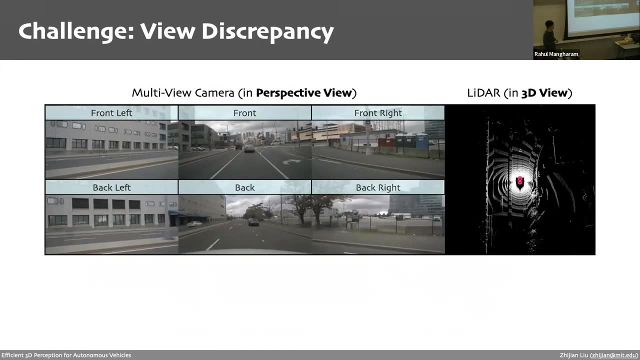 from a single sensor and make the 3D perception system more robust. So one of the significant challenge in the sensor fusion is the view discrepancy. So that means different sensory data are in a different format in a different space. So, for example, here we have the camera data. 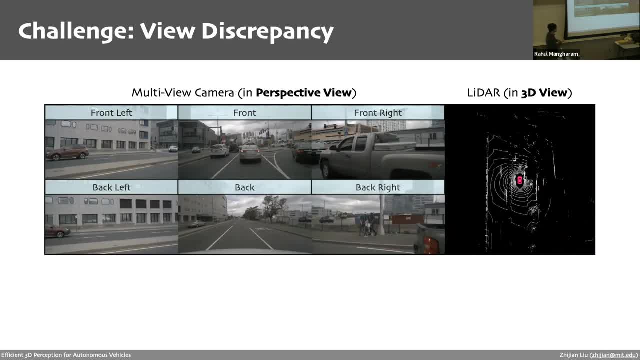 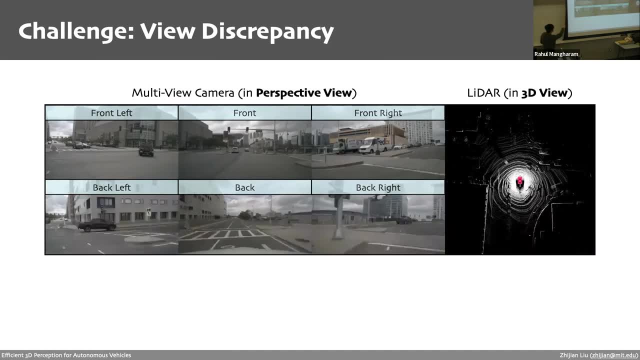 So they're in a perspective view and we have the LiDAR data is in a 3D view And also you can see actually different camera data as they're having different orientations. So that means if you're considering the top left corner of each camera sensor, 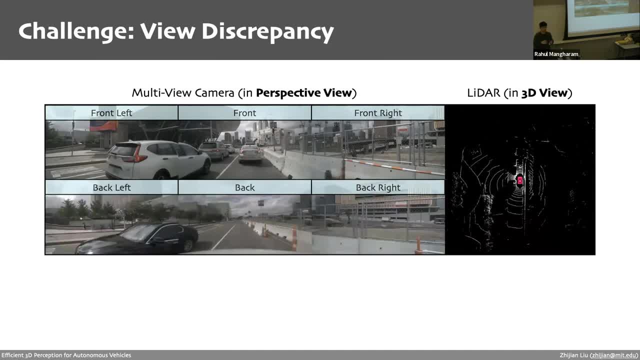 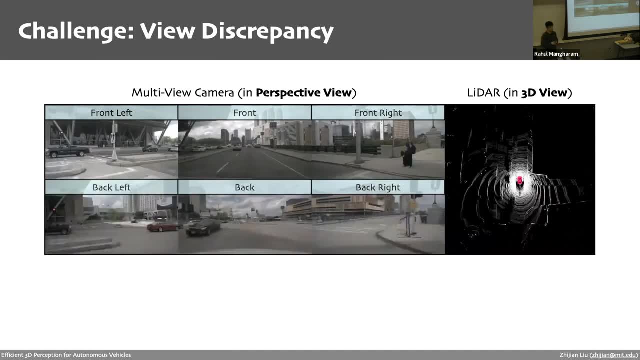 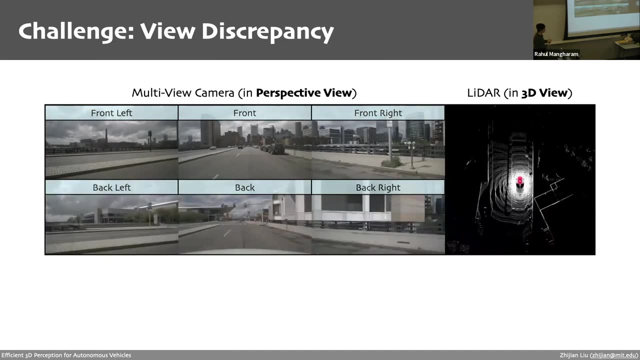 they are not actually corresponding to the same spatial location. You want to understand, like, the spatial relationship between different pixels across different camera sensors. you actually need to know how the cameras are mounted and using some calibration to understand like the locations. So that means we can not like naively. 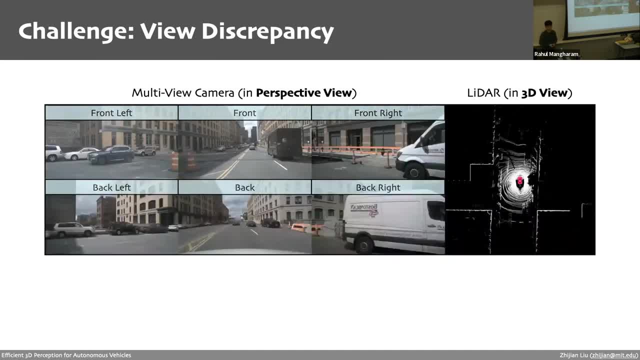 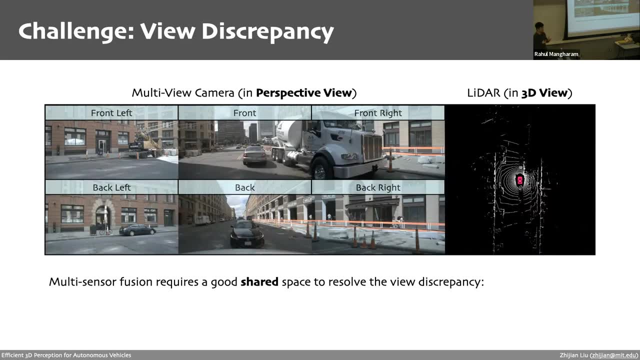 just adding these features together and fuse them together, right, Because they are not actually responding to the same spatial location. So the goal of the multi-sensor fusion is actually to find a good shared space to resolve the view discrepancy issue. So there are two requirements here. 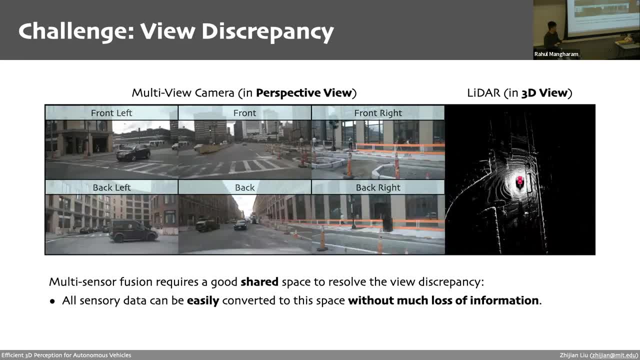 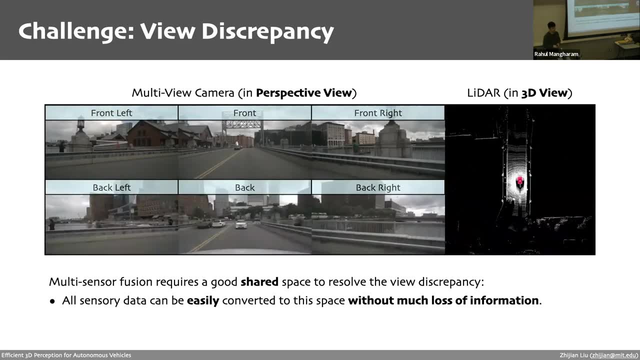 First, the sensor data needs to be easily converted to this space without much of the lots of information. But here the conversion has to be implemented can be implemented very efficiently and in a very easy manner, And also the information loss is another thing. 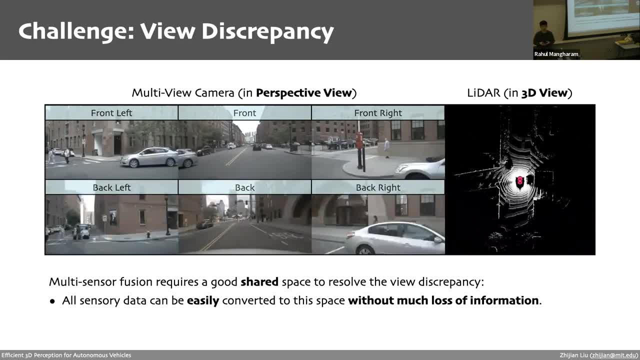 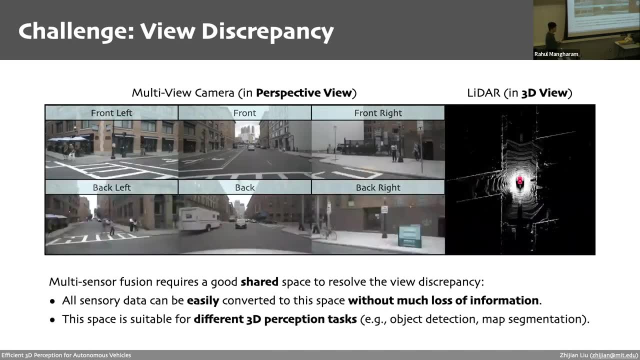 we need to consider, because different sensors are giving us different information. we want to preserve this information as much as possible. And the second requirement is this space has to be suitable for different 3D perception tasks, Because in reality, we care not only about the 3D object detection. 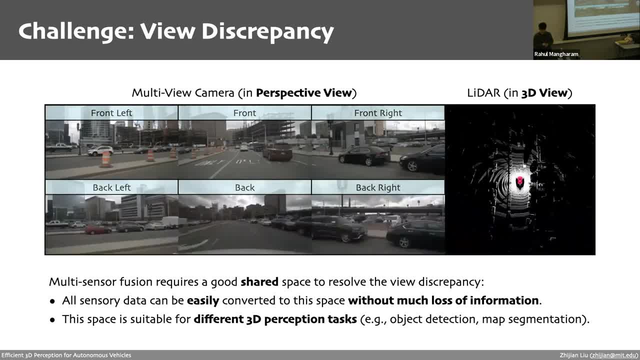 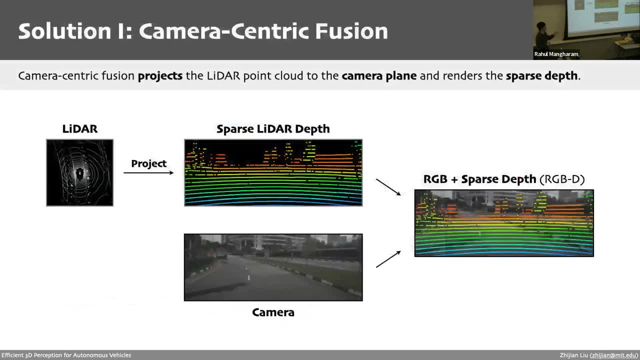 we also care about some other semantic tasks, like the matching. So now let's take a look at a few existing solutions. So the first solution is called camera-centric fusion. It's actually motivated by the RGBP data. So the basic idea is: we can just project. 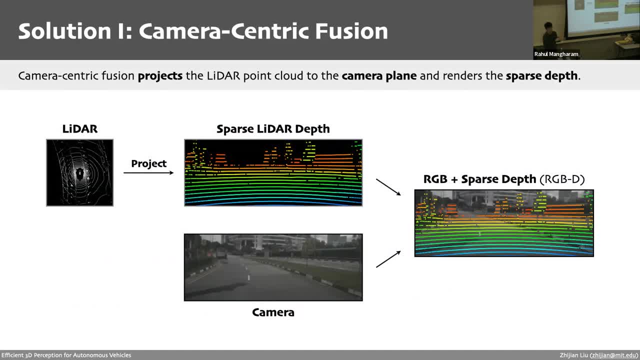 the light-up point cloud onto the camera thing using the camera's light-up transformator And then you can see this is the sparse light-up that we'll get. It's kind of different from the light-up that the DAPs will have on RGBP, since it's much smaller. 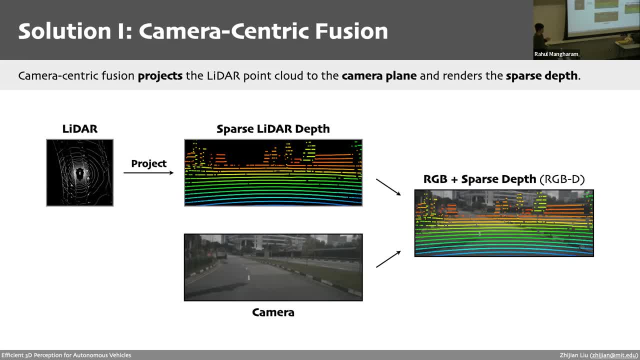 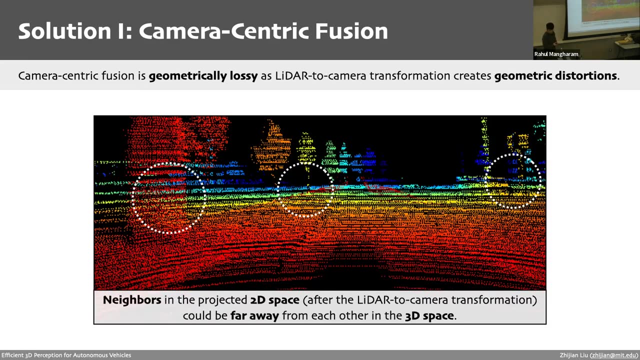 which is the sparser here, And actually we can just concatenate them together and we can process it using, like any camera based 3D detection model, the FTO model I just mentioned. So what's the problem of this approach? So let's take a closer look at the light-up. 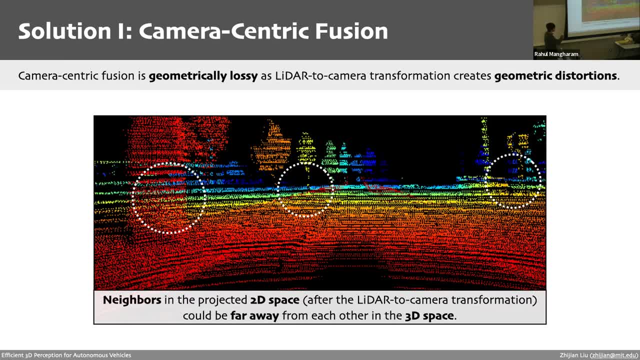 that's projected to the camera thing. So I circled out a few regions here. You can see that within each circle right there are clearly some points which, like there is kind of there is- I'm not saying that- some of the Light-Up points. 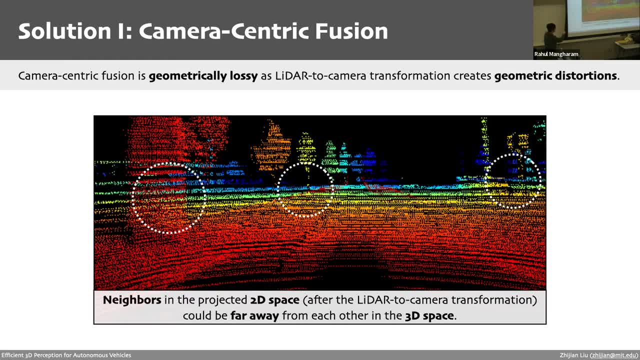 with like very different colors. So for some of the points the depth is actually very small and for some of them I can have a very large depth. So there's a discontinuity in the depth convergence. The reason for that is the projecting. 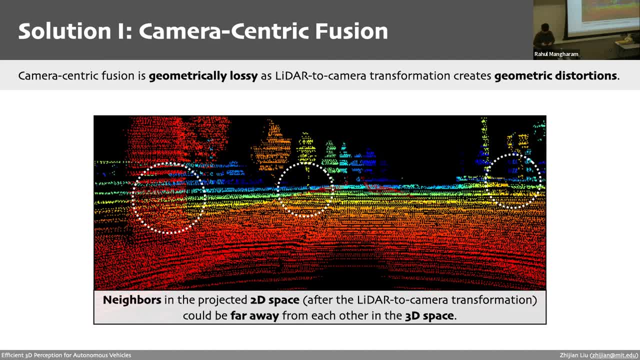 when we are projecting the LiDAR point out to the camera point. but that's back of each pixel. it's actually determined by the closest LiDAR like point to the pixel. Therefore, like neighboring pixels can have different depths as long as they're close to the 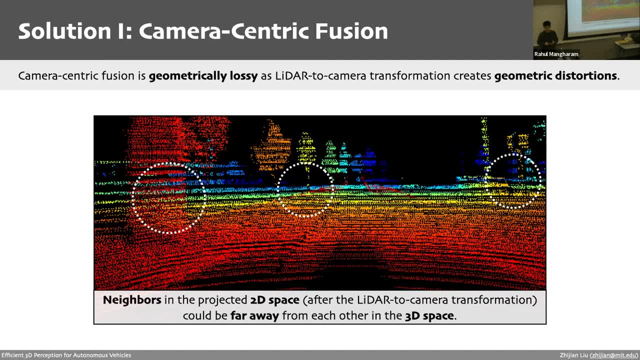 closest to a different LiDAR point. So this will result in a loss of information about the true 3D structure of the scene and the object, making it very hard to accurately detect and localize the 3D objects, And this could be an issue for a 3D detection process. 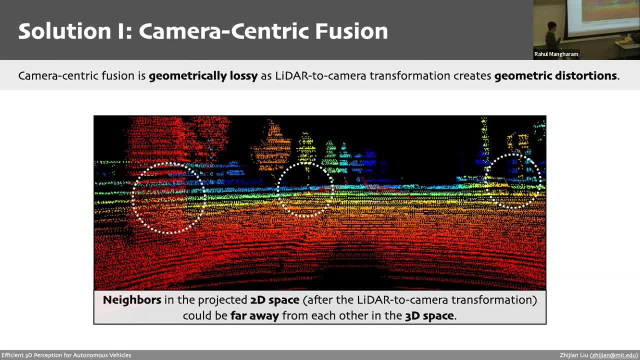 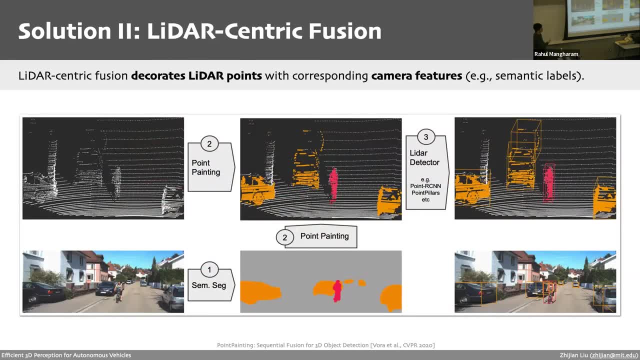 So that's why actually most of the leading like multi-sensor fusion 3D detection models don't really follow this approach. They're using a different approach called LiDAR-centric fusion. So the idea is that we want to project the camera information. 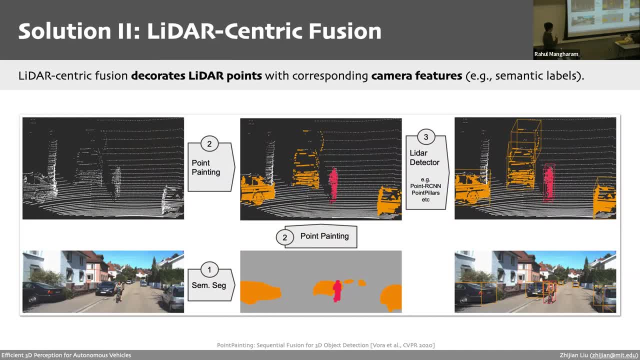 to the LiDAR space. So here is a very representative work called point painting. It's actually from the same group as the point pillars. So the first step is to run the 2D semantic sanitation to get the semantic labels for each pixel. 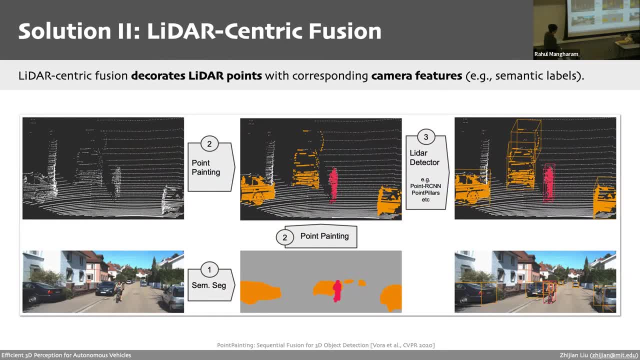 For example, here we have the cars, we have the cyclists here, And after that we paint the semantic labels to the LiDAR point out, So it would be a color point out afterwards, And then we can just use any LiDAR detectors to process it. 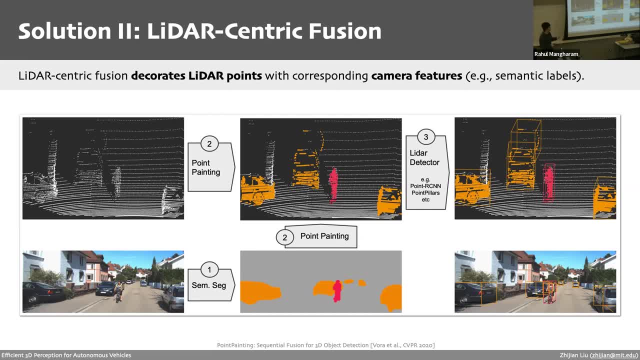 For example, we can use the point pillars. We can use like sparse cone, like point RCNM to process it. So what's the issue of this approach? So the camera to LiDAR projection is actually very lousy in the semantics. 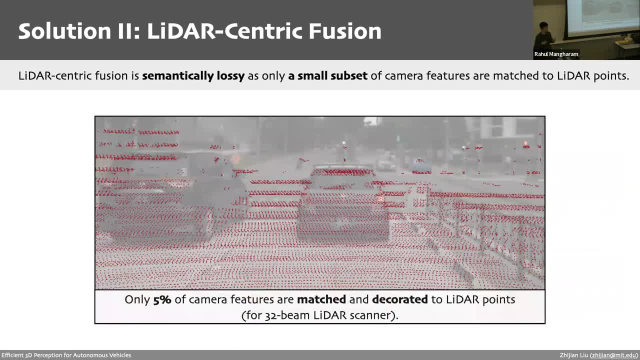 So the camera and LiDAR feature, because the camera and LiDAR data have drastically different densities. So here you can see, all these red dots are the LiDAR points projected onto the camera. So only 5% of the camera features are actually covered. 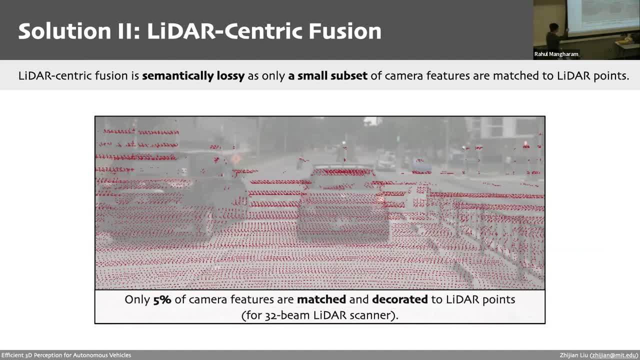 by one of them. That means all the other points, as long as they're not visualized in red here, they're actually dropped directly during the decoration, the painting process. This is actually not optimal because, you can see, the semantic information is very important. 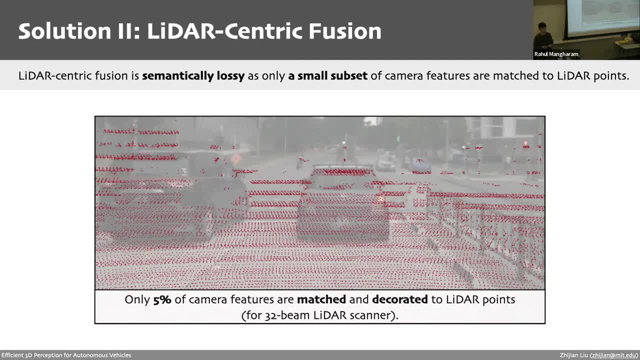 For some classes. for example, if you want to understand the layout of the screen, that's definitely unnecessary information you need to use. And also another thing we can notice here is the top right corner of this image is barely covered, So the reason for that is the LiDAR. 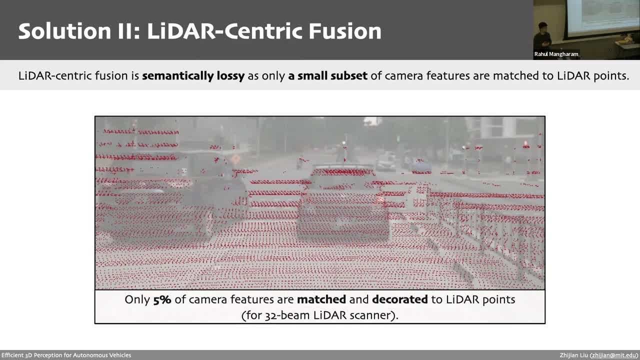 has a limited coverage in the range, for example, like plus minus 50 meters, while the camera can actually capture objects that are very far away from the legal part. So if you're doing the fusion in this manner, if we project the camera, decorate the camera features. 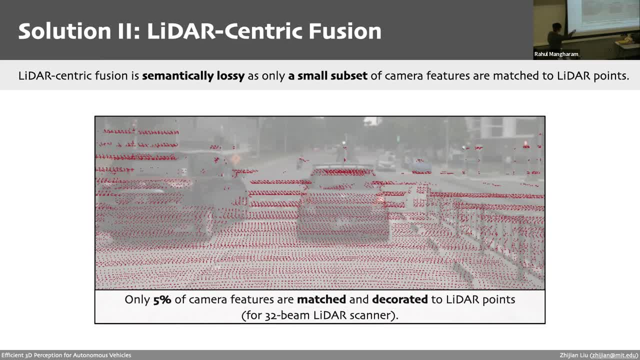 to the LiDAR data. all these image features, camera features, will be directly discarded. That's also not optimal. So now we have talked about the limitations of both camera-centric fusion and the LiDAR-centric fusion. Oh, OK, I just had a question. 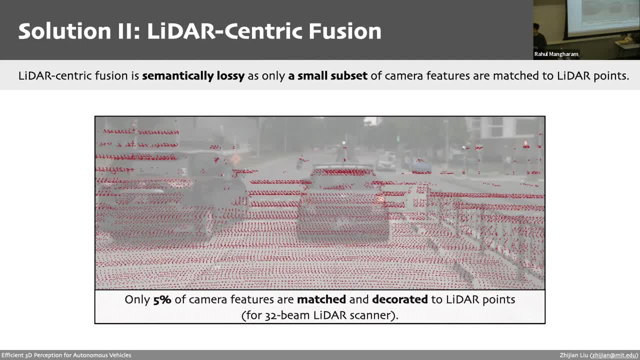 Have you used or have you seen anything in the literature about using intensity images or reflectivity images to do these kinds of fusions between? I'm also projecting a LiDAR to a camera, Sorry. So are you also projecting a LiDAR data to a camera using? 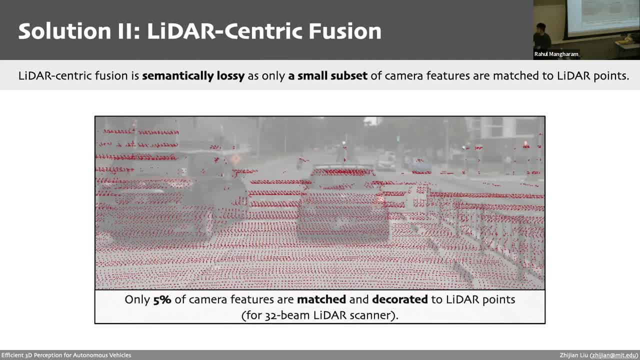 the Yes. yes, This is actually very similar to the camera-centric fusion. So I haven't really I haven't seen a lot of papers doing that- for the object detection, specifically because the camera-based detection model, the accuracy actually lags far. 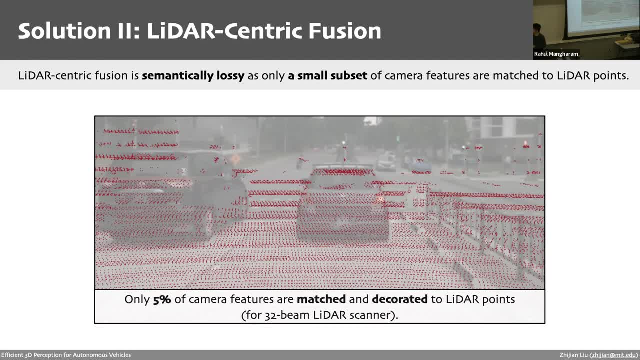 behind the LiDAR-based detection. So most people have decided to do that in the LiDAR space. But I think that's actually a very interesting idea because nowadays actually the camera-based detection catch up in the accuracy a lot. 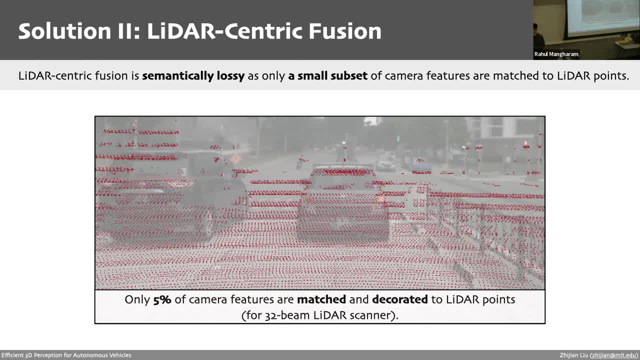 So that approach could be an interesting direction. Yeah, so we have talked about the limitations of both LiDAR-centric fusion And the camera-centric fusion. So here comes the first small quiz. So what other options do we have? How can we fuse the information better? 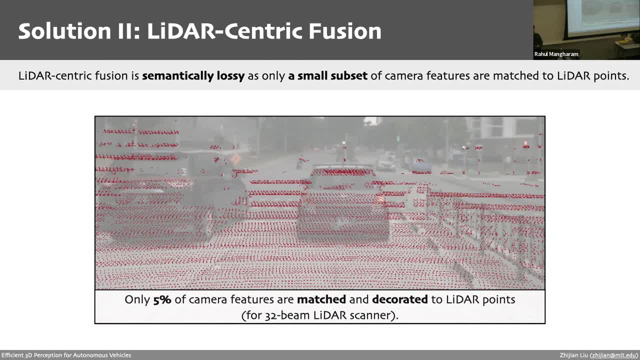 We have the camera, We have the LiDAR. Is there a better solution for the fusion? You could object space, Object space, So technically space. Yeah, that's actually a very interesting idea. So some papers actually have explored that. 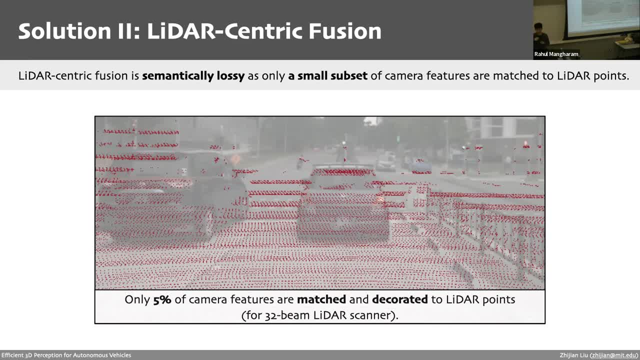 So they use some sort of latent object queries And then they project. They project it onto either camera and LiDAR. That's actually a very interesting idea. It's actually very effective in the detection three detection models. But if you think about it, if we care about the map segmentation, 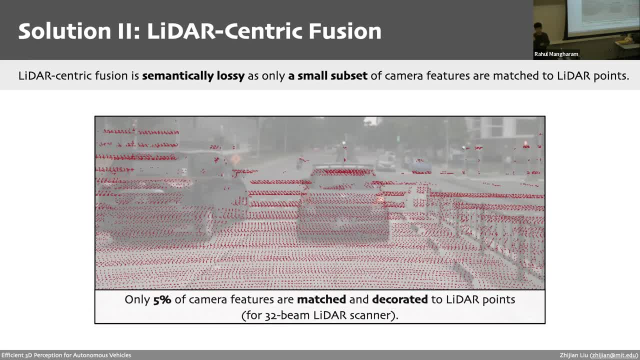 that could be very challenging if you only care about those objects, using the objects to query the different sensors, Like in feature space, In the feature space. So what kind of feature space? So you have a feature extractor for the LiDAR and another feature. 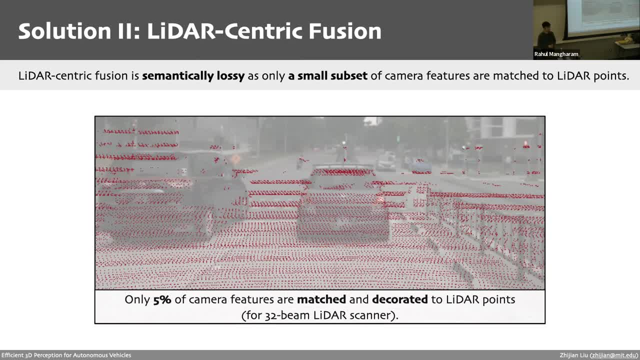 extractor for the image And you directly use the output like a latent space for both. You directly use those numbers as your combined feature. So that means that you have the camera features, LiDAR features and then you do some spatial pooling. 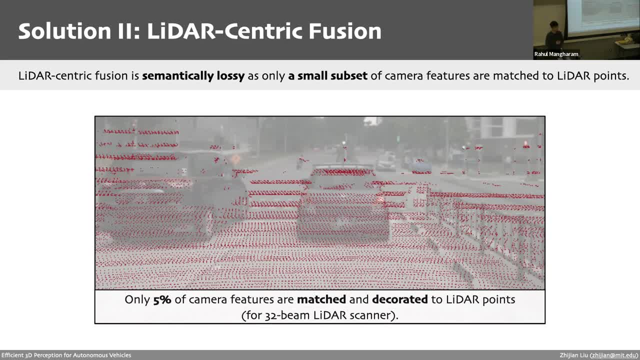 You just directly use the, so you put two. You can put two. You can put two Compactly. it's the output from two different feature extractors. I see, I see, So it fights in the features from different sensors. 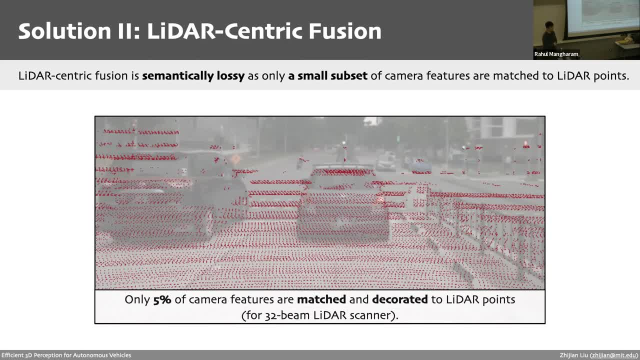 Yes, And then use that as a fusion feature. I think that could be an interesting idea. I think, yeah. So some people will do something a little bit more complicated, do something like pause the tension between the hidden features. That's actually a very interesting solution as well. 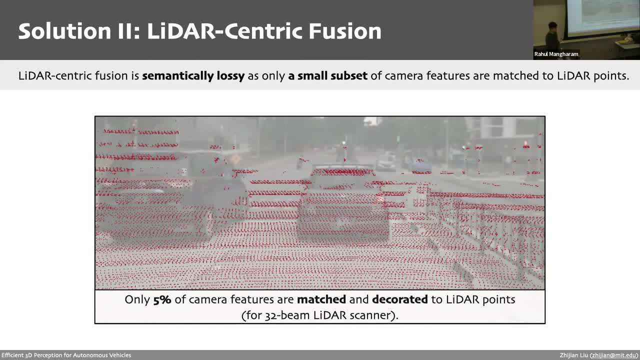 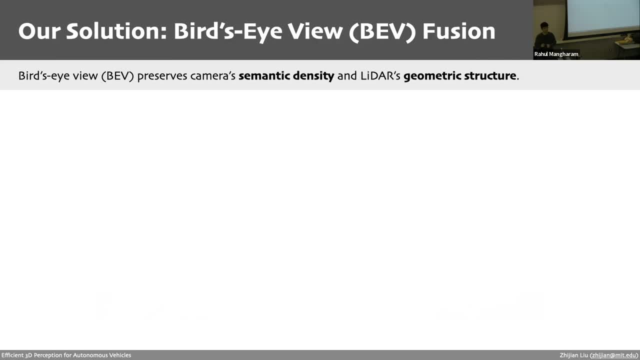 So actually our approach is already in the name of the, the paper It's called. So basically we're choosing the first idea: space. There are definitely other options, of course. Obviously, object theory, the feature space, latent space. 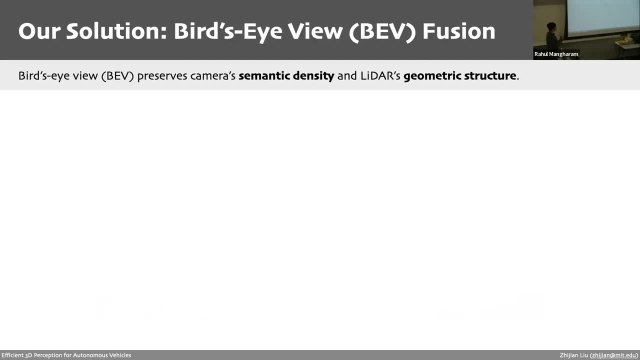 could be a good alternative as well. But the reason we chose this space is, first, most of the 3D perception paths in the first idea space, Because they are mostly extracting features attaching heads in the first idea space. So let's take a look at how we can transform the features. 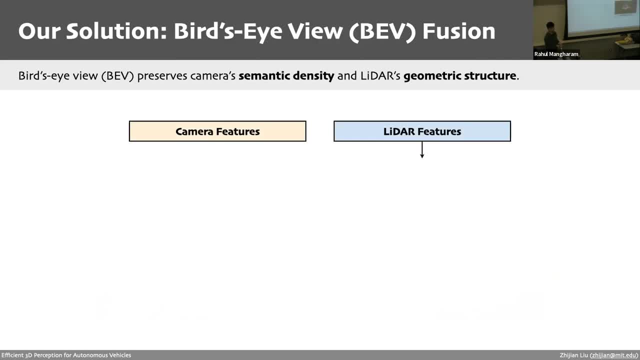 to the first idea In a high level. So features: it's actually very simple Because it's already in the 3D space Projecting. to the first idea: space is just discarding the z-axis right And you can see it's kind of preserving. 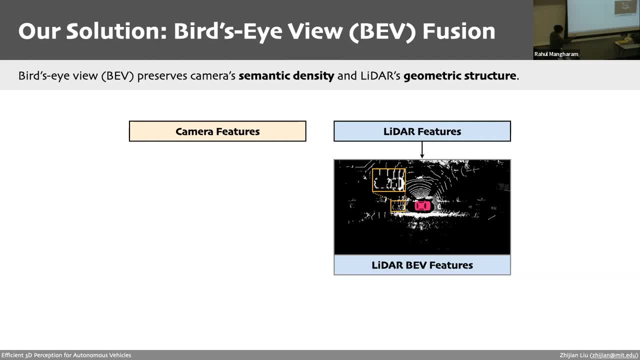 the geometric structure of the LiDAR, Because you can still see that this is a car right Even after projecting the height dimension. But in reality we don't really discard the directly discard the height dimension. We'll do some feature aggregation on the height dimension. 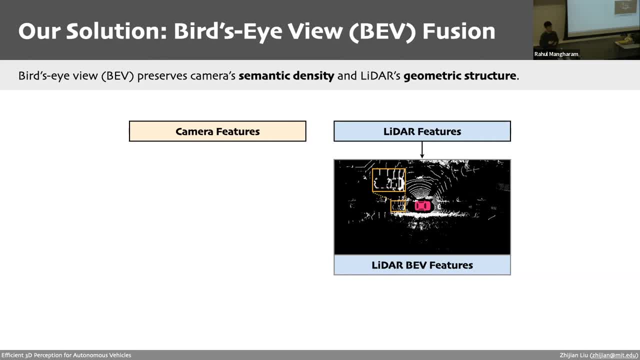 to invite it to the channel dimension. So in this way the z, The information of the z, is kind of still preserved. Well, the camera is a little bit more complicated. I will detail in next few slides, But the overall idea is we have multiple cameras. 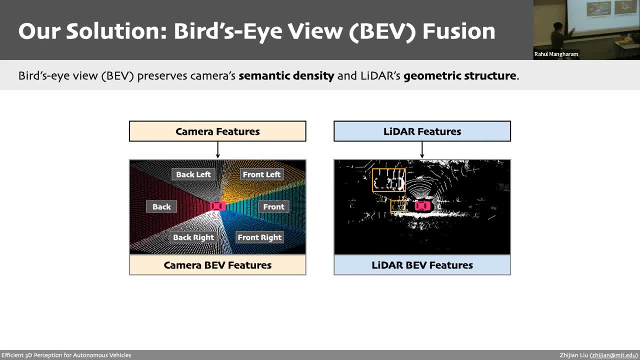 that are having different orientations. We want to project it onto this shared bird's eye view space Here- front camera, back camera and the other cameras as well. So from this visualization you can have a very intuitive sense that it's also very dense, semantically dense. 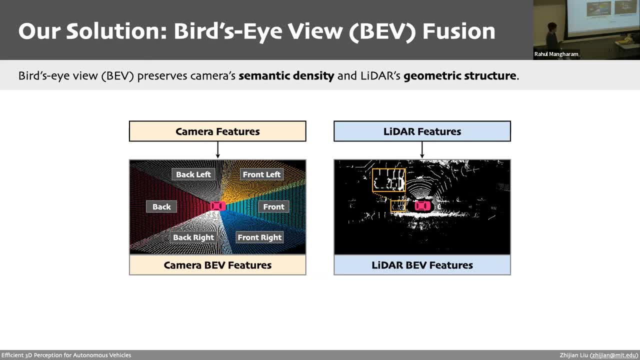 So preserving the density of the camera features. So, after all, the features are capturing the bird's eye view. we can easily use them together, using them, using some like animalized operation. So let's take a look at how we implement this. So, given different sensory data, for example, 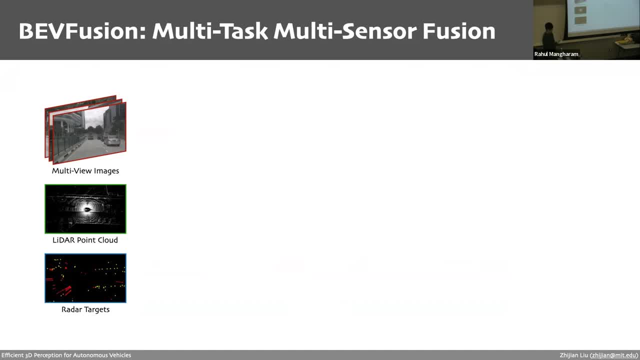 we have the multi-view images. LiDAR point out the radar targets. We'll first use the modality specific encoders to extract your features. For example, here we are using like Swin Transformer using ResNet as our camera encoders using VoxelNet. 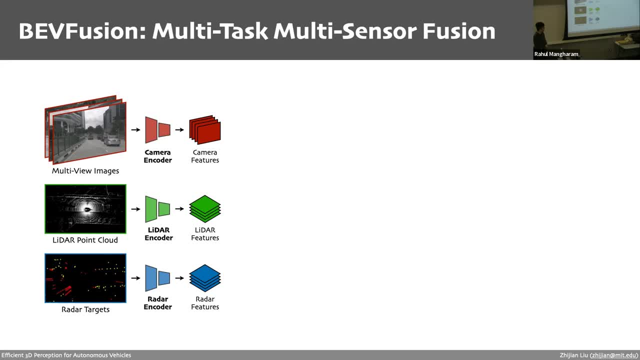 as our LiDAR encoder and the point field is our radar encoder. So, after this encoding step, the camera's features are still in the perspective view, while the LiDAR and radar features are still in the 3D space, And that's where I transform all these features. 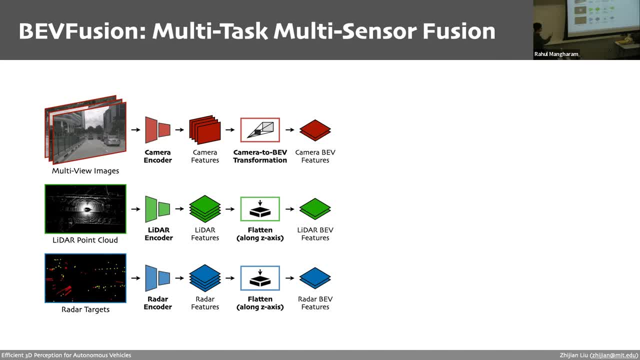 in a unified bird's eye view space. So, as I mentioned, the transformation process for the camera to bird's eye view is a little bit more complicated, So I will show you from the next slide If LiDAR or radar is very simple, we just flatten it. 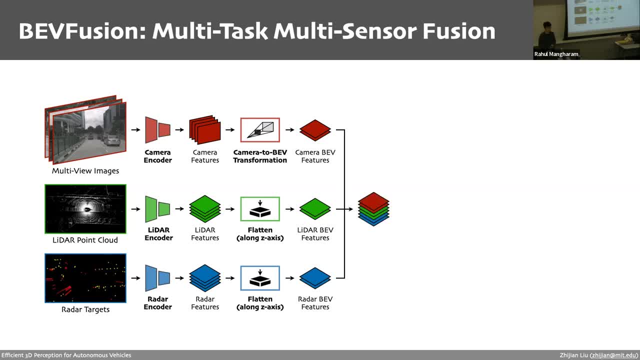 So once all the features have been converted to the bird's eye view, we can just simply stack them together and then apply a BIM encoder to fuse the features together. And finally, we can apply multiple tasks, specific tasks. For example, we can attach some detection. 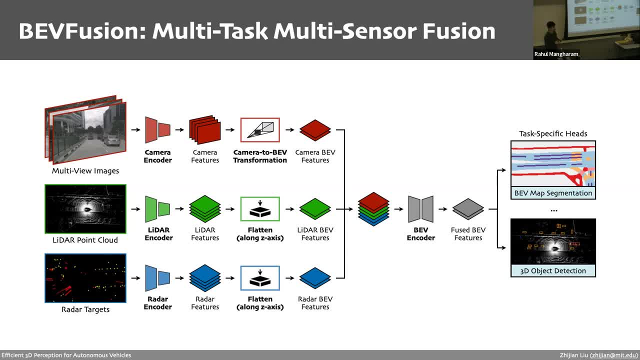 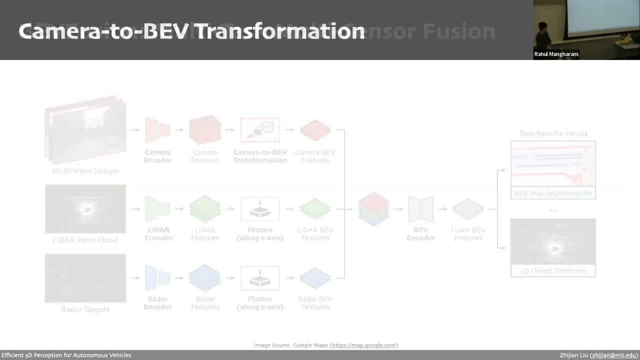 like sensor-based detection, have three: object detection and some segmentation. have for the BIM map segmentation. So now let's focus on the camera to bird's eye view and then the BIM encoder. So this process can be a little bit abstract, so I will first provide you with an intuitive idea. 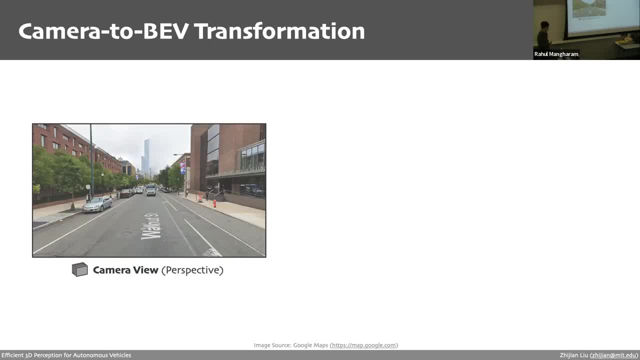 of how the process works. So to illustrate this transformation, so consider this street view image right of the School of Engineering here. I found online. So this image is captured in a camera. from the camera we can see. it's in the perspective view. 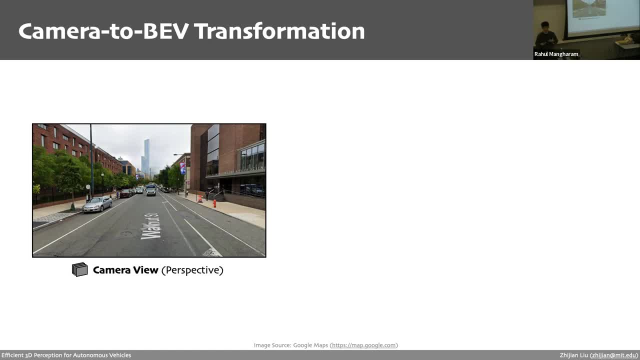 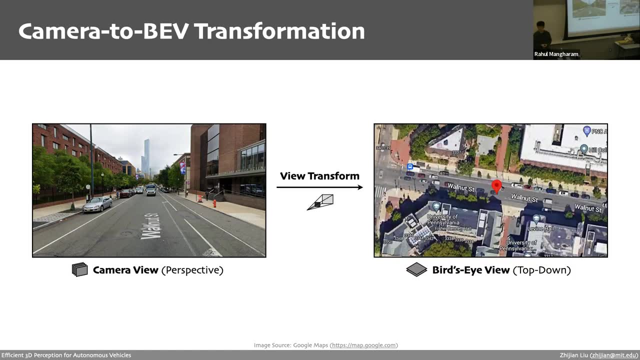 So the goal of the view transformation is actually to convert this perspective view image to a top-down back view image. It's very similar to the like the satellite image you can see here. So how can we achieve this? So the first step is we want to understand the depth. 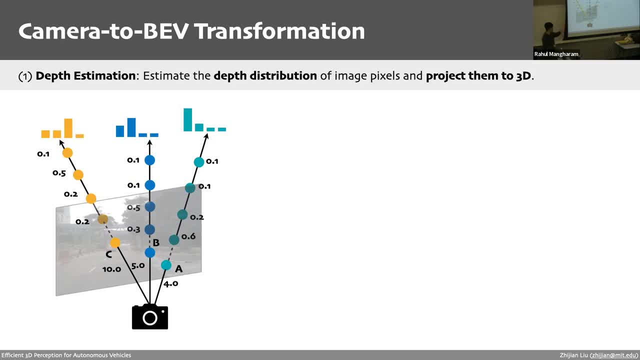 of each image pixel. This is actually a very challenging task for the camera data because camera doesn't really provide such information. So we followed the previous work to explicitly detect, predict the depth distribution of each pixel. For example, you can see here like for the pixel A. 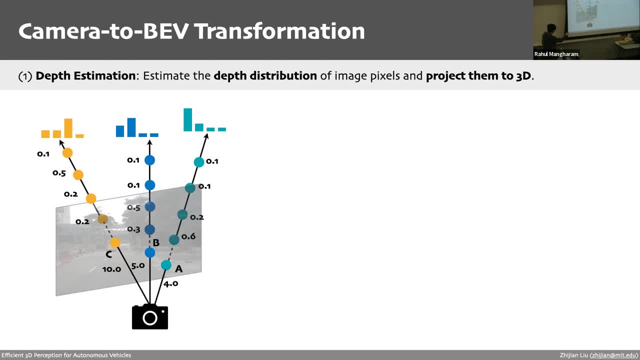 it has a large depth probability either a smaller depth. So the basic training at this point is probably very close to the camera, While for the pixel C, here it has a large probability value at a larger depth, So it's probably very far away from the top. 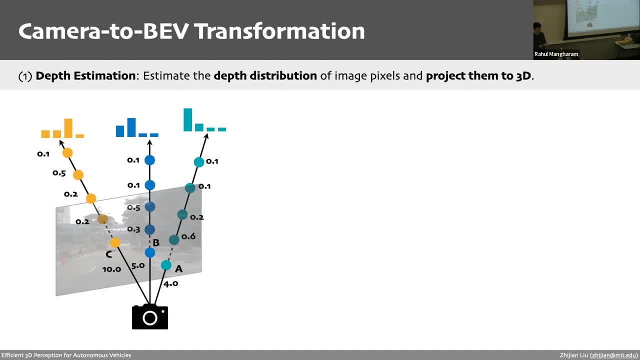 So this step is essentially a depth estimation process. So we can achieve this by just applying a few convolution layers to the image features. And next we want to scatter each of the image pixel to a few distributed points, For example here, like we: 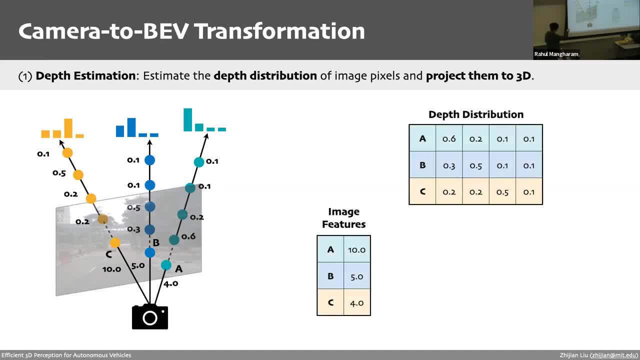 for each of the ABC, these three pixel. we want to scatter four points here, So in total we'll have 12 points after the scattering process. So the feature of the scatter point will be depending depends on the two factors. One is the original image features here. 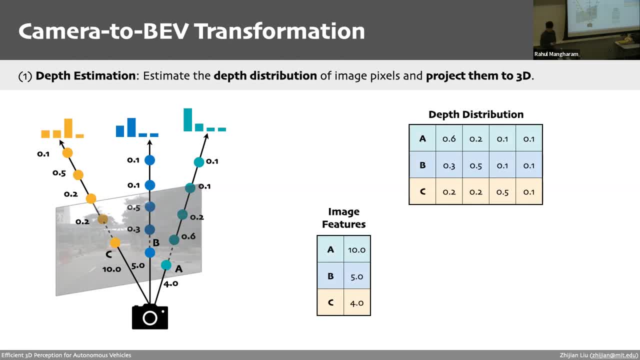 and the other one is the best distribution which is predicted. So the basic idea here is we just simply multiply these two factors together. For example, you can see the highlighted box here. the 2.5 is obtained by just multiplying the corresponding image feature here. 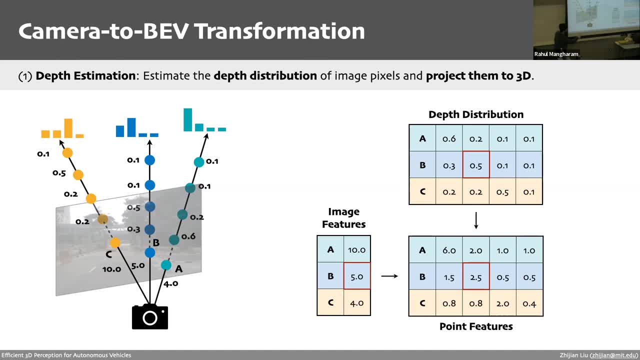 which is 5.0, and the best distribution here, which is the 2.5.. So this resulting, so this completes the first step of the like BV2, camera to BV transformation. So, in practice, after the bound sampling. 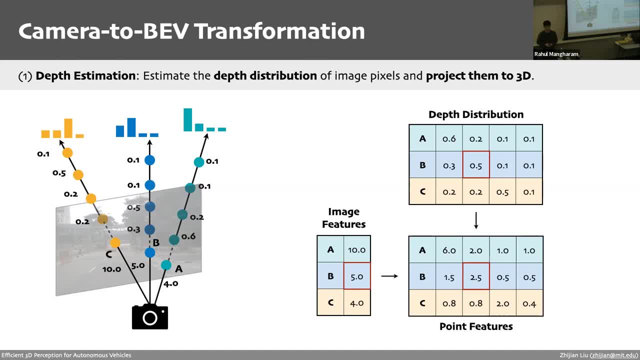 so here we'll have around 3000 image pixels And for each of them we'll generate around 100 points, And because we have six cameras in total, so that means we'll generate a super dense point of health- around 2 million points. 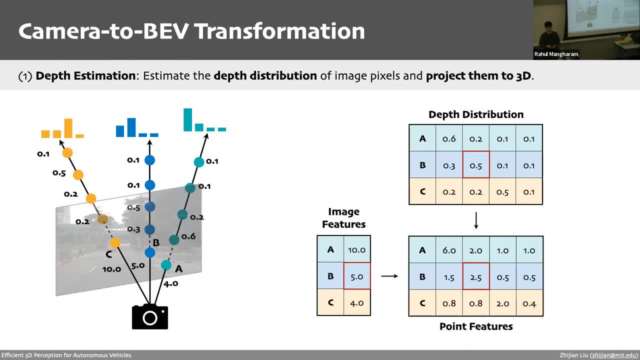 So that's actually like two others of magnitude, denser than the light of health. So we need to keep that in mind in the next few steps because that could be an overhead. So the best distribution you get it from a monochrome. that's asking. 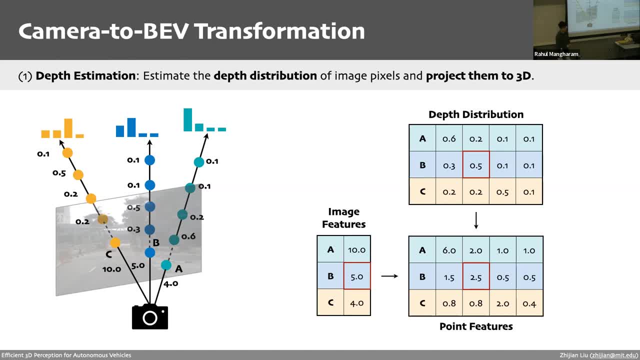 Yep, that's a monocular. sorry, Which one did you use? So basically, like after the feature extraction, we just apply a few convolution layers together, because we don't really need a very accurate depth system for this. Okay, you're not using an existing word? 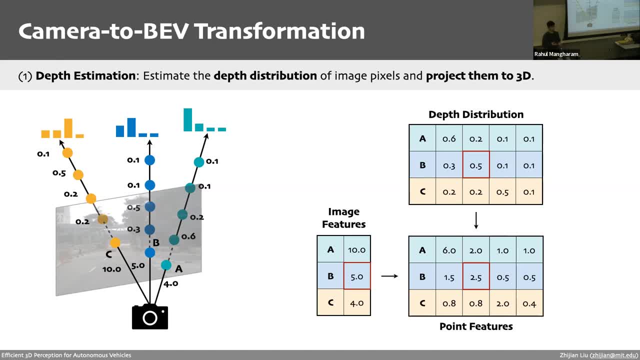 It's part of the pipeline. We want to blend that into the original camera encoder, If we want to, if we use a separate like that's estimation model actually to give us a huge overhead to the other side. Are there any other questions? 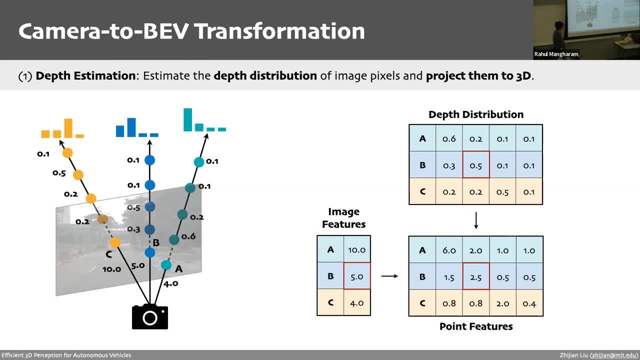 How do you get the number of image features? Oh, we use a camera encoder, for example, there's a rest net to extract the features And then we have, like the, you know, you can get the number of white features for all of them. 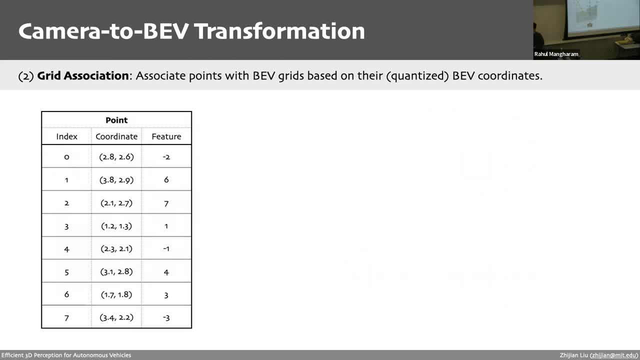 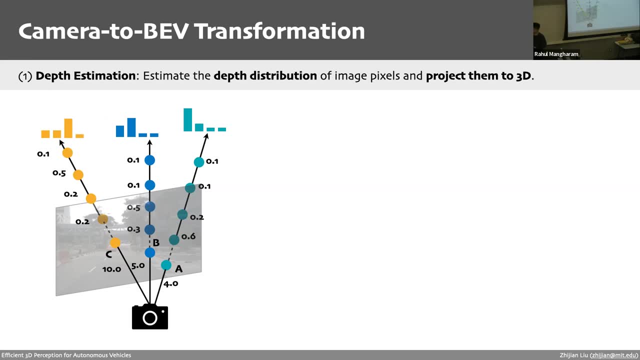 Right. So okay, How did you get the number of white features Instead of The number of point features? you mean, like, how many points we scattered, right? That's actually a determined fixed number, For example, for each pixel. 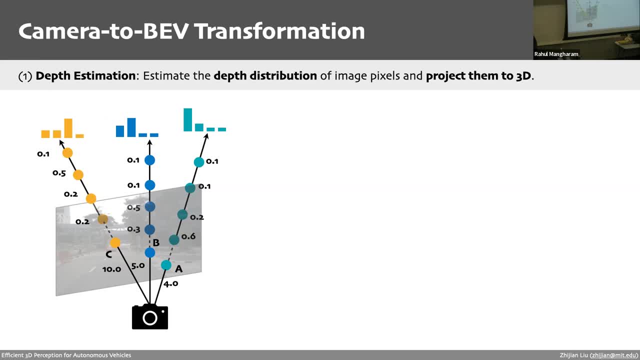 we'll generate one point for each depth value. For example, like 0.5 meters, one meters all the way to a 16 inch, Okay, So like there are like a lot of stuff, So you can get 120 points per pixel. 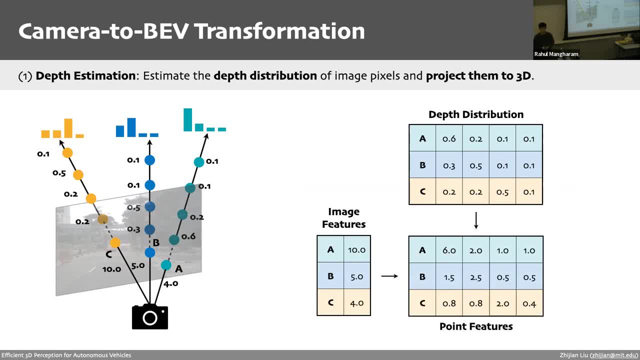 What happens when you end up with two points at the same position? Yeah, that's exactly what we're going to handle in the next step. We want to pool, like do some pooling right, Like for all the features actually in the same grid. 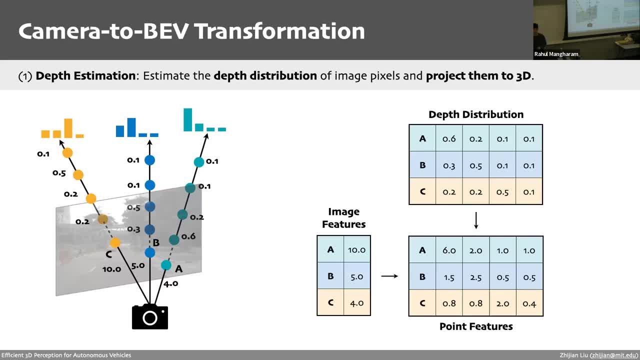 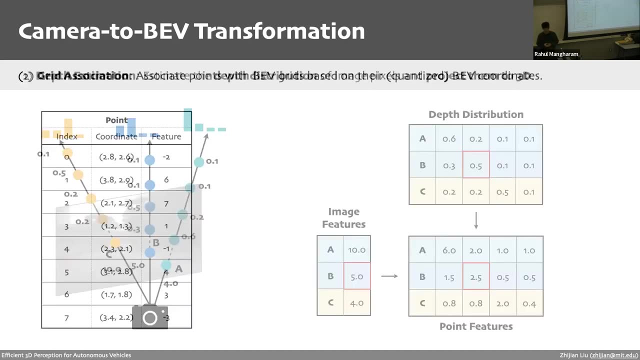 So it's not necessarily there having the exactly the same 3D coordinates, but as long as they're close to each other, we want to kind of like aggregate your features together into one feature. Yeah, So actually before that we want to first understand, like the association. 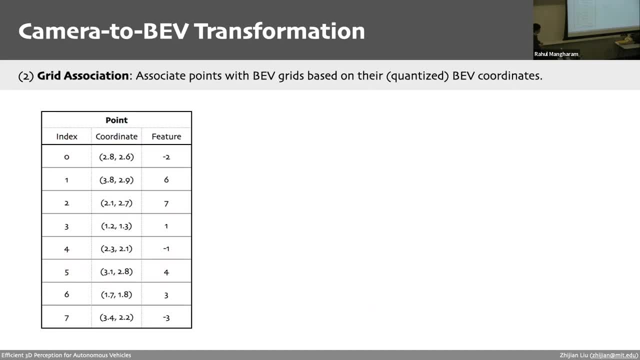 or actually like which are the points that are actually close to each other. So we did a grid association here. So this is an example of the point cloud generated after the scattering step. So for each point we have a, B and E coordinates here. 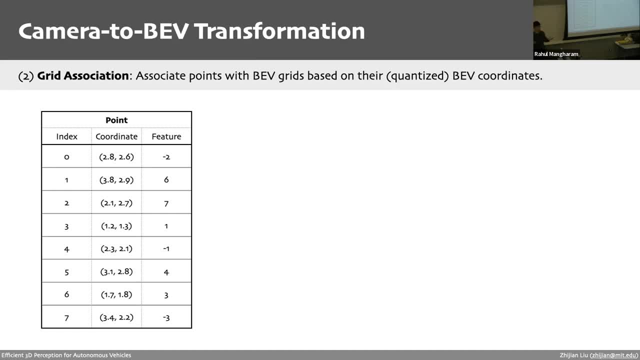 And also we have a feature corresponding to that. So the way we generate features, it's just multi-clining in the image features and depth values. So for example, let's consider, like the first point here, with index zero, this coordinate is 2.8, 2.6.. 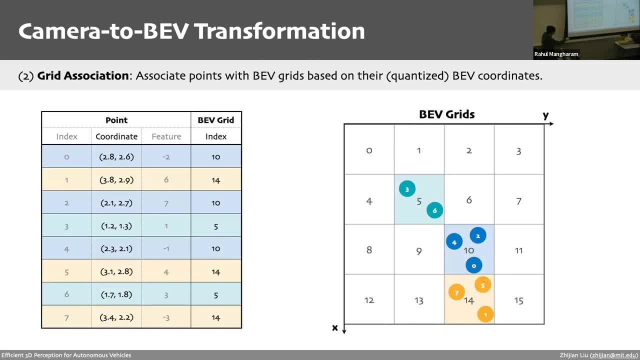 So that means it falls into, like this blue grid, So it's a tense grid. So you've got a BV grid index of 10, and the same applies to this one. The coordinate is like 3.8, 2.9.. 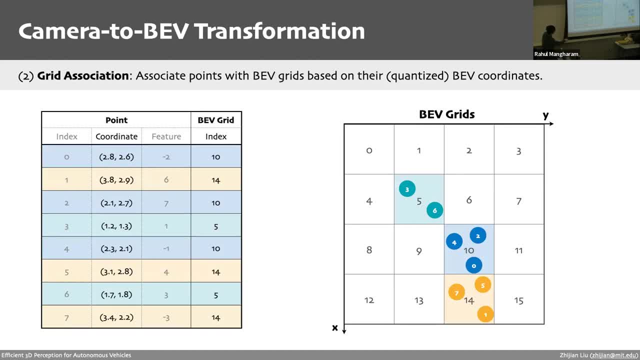 So it's actually in the yellow grid here, So you can do the same for the other points and get a good index here. So this can be. and then we want to reorder like all the entries in this table So that like all those points. 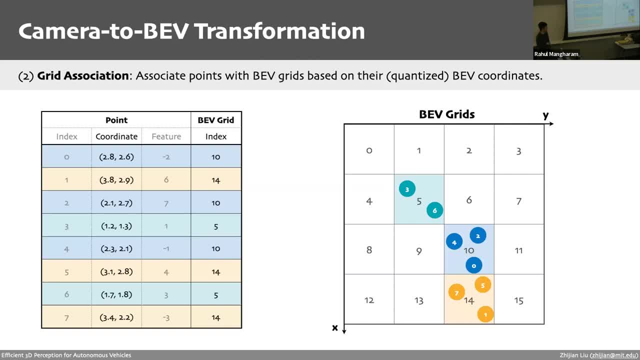 with the same BV grid index will be consecutive with each other. So this stuff can be achieved by like doing arguments for it based on the BV grid index And then we'll just reorder all the entries based on the sorted rank. So this is the table after the sorting, and see here. 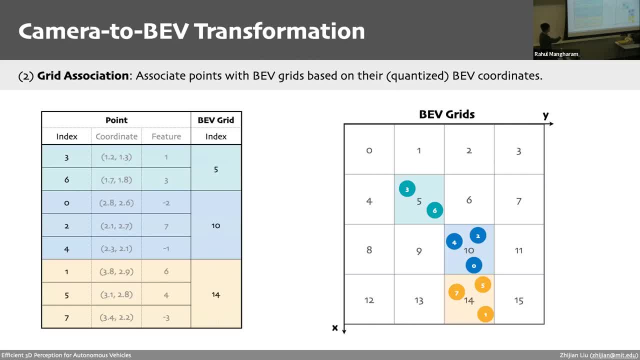 the point index is no longer consecutive anymore. This is basically the rank we'll get And, like the steps, this step seems very simple. It is actually surprisingly slow because sorting over 2 million entries with an argument sort is like a lot of computational effort. 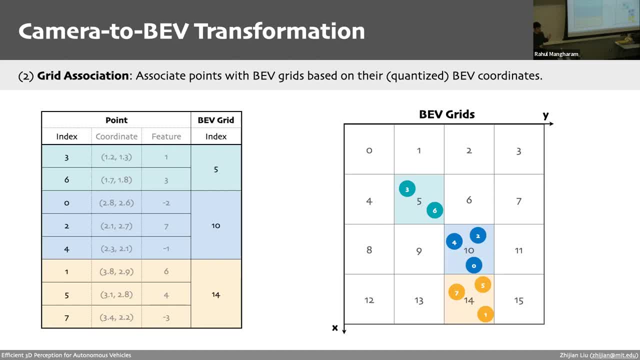 So, but there's one property we can leverage here to accelerate this process. So all the point coordinates here is actually fixed. If you think about the way it's generated, it's only based on the original camera. greeting that sorry, the original camera coordinates. 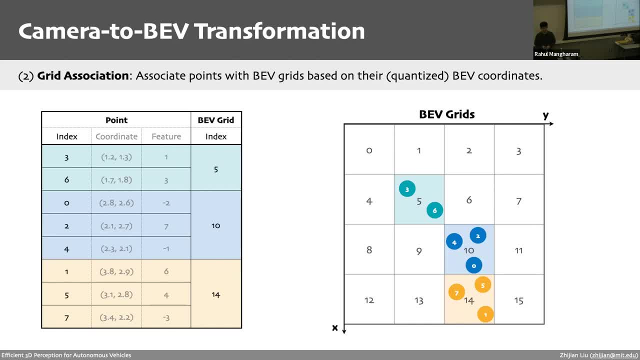 and the transformation between a camera to the LiDAR. So as long as the sensors are well calibrated, for example you have all the camera mounting known and also you have LiDAR mounting configuration known, then this is actually fixed. So the point coordinates are fixed. 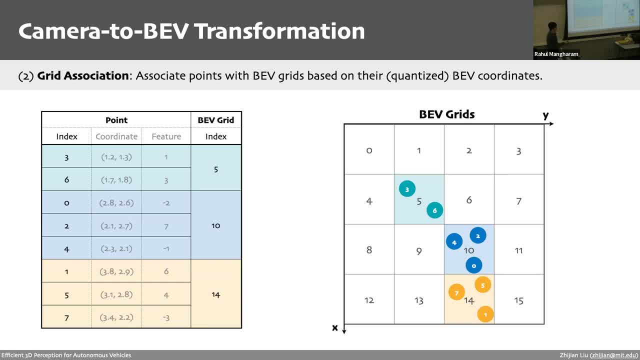 and therefore the BV grid index is also fixed And therefore the rank here is also fixed. So we don't really need to do the sorting during the inference time. We can just do that once, like beforehand, to store the pre-completed rank. 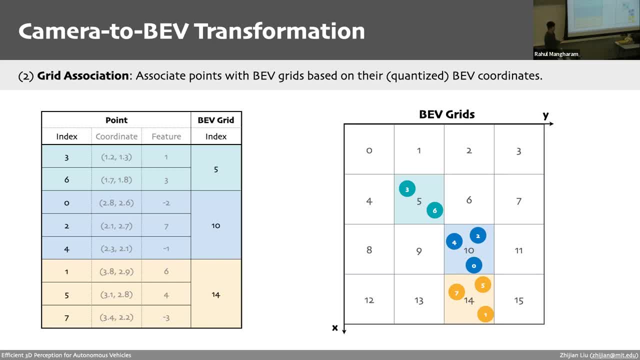 And during the inference time we can just use the rank here to reorder all the entries. I thought that the coordinate somehow derived as well from the depth of the point, Because we actually generate a very dense point. So actually for each of the taps we'll generate point. 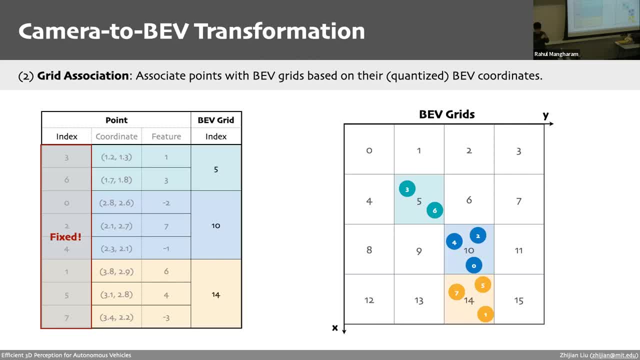 Yeah, so actually, yeah, I think you're right in some way, like if you consider the like, for example, for one pixel, the one with the largest taps is actually dynamic based on the based on the taps prediction, but we're actually generating a very dense point. 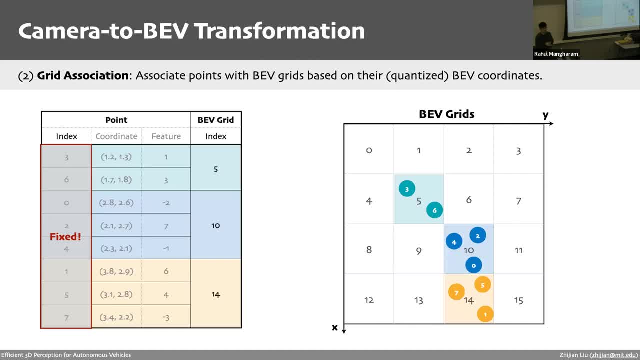 The reason for that is we want to make sure this process is differentiable. If you generate only one point, so that means we're doing some sort of arcmaps over all the taps probability. The arcmaps is not a differentiable process, So we want to use that as a proper relaxation. 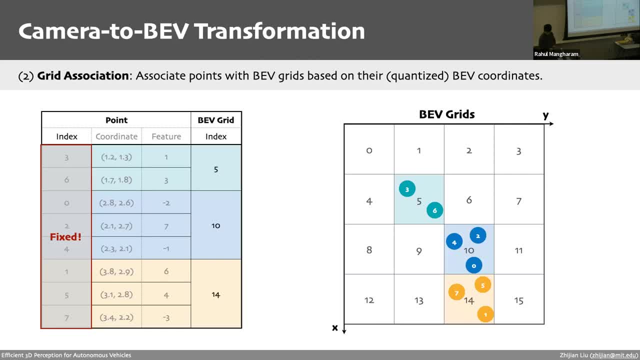 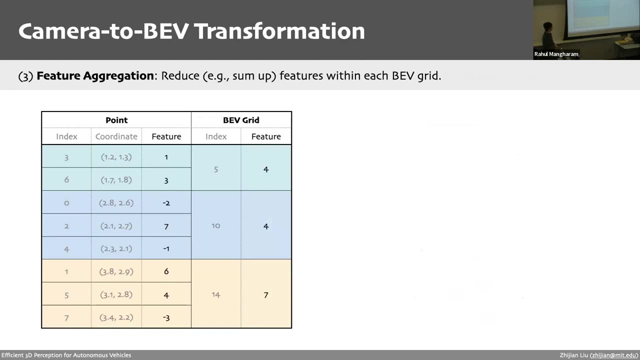 to make it differentiable. Yeah, So the computation optimization. although it's very simple, it can actually like optimize this, like the latency of this step, by a factor of four. So now all the points within the same degree will be consecutive to each other. 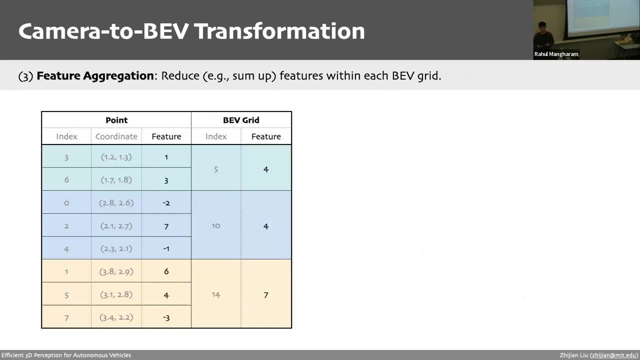 The next step is to do some reduction over all the features within the same degree here. So the reduction function we're using is just doing a summation. So for example, you can see here that for the first grade the feature is four. we can obtain it by one grade right. 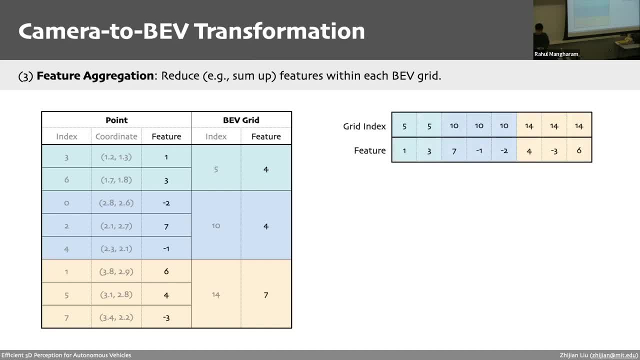 So let's take a look at how to implement this. So aggregating the features within each BV grid is actually not very straightforward because you can see that different BV grid can actually have different numbers. So the existing implementation from LSS actually uses a very ever prefix sum tree. 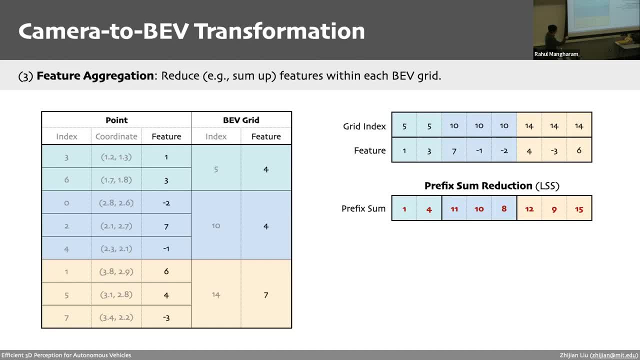 So basically the first calculus prefix sum of the feature. here you can see we got one and four is basically one plus three here and 11 is four plus seven and so on and so forth. We first got a prefix sum vector. 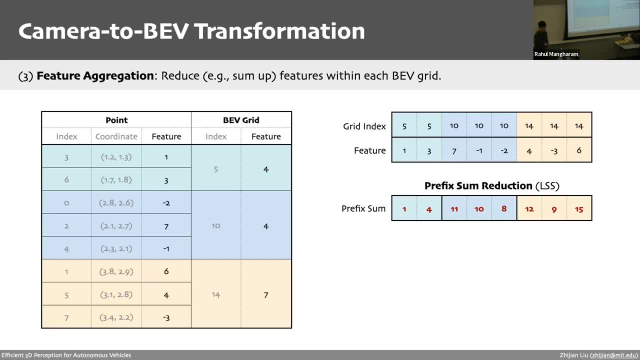 And then after that we just subtract the values at the boundaries where the indices change to obtain the reduction values within each BV. So here we can get a four. here Four is basically subtracting an imaginary zero, here by the from the four. 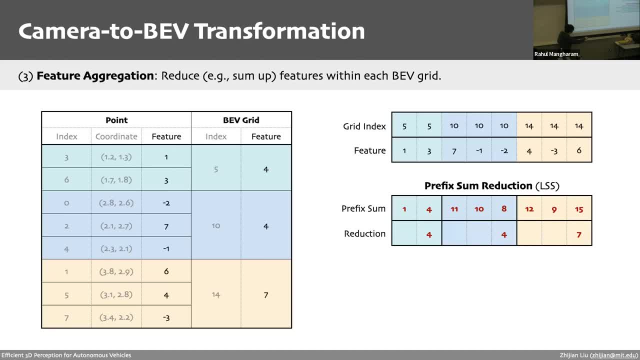 And then the four here is subtracting four from 18, and seven is 15 of eight from 15.. So we can compare the results here and here it's actually correct. So this is a very clever implementation because it reduces a lot of existing operators. 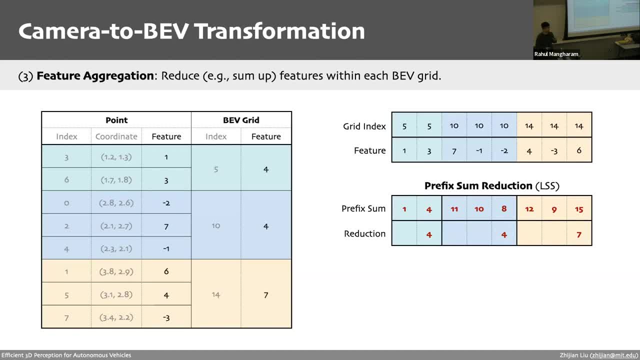 for example in the high-tour intensive flow, for example, doing the prefix sum, doing the subtraction, doing the indexing. But the issue here is the prefix sum is actually not very efficient on the GPU. It requires a multi-level tree reduction to get it. 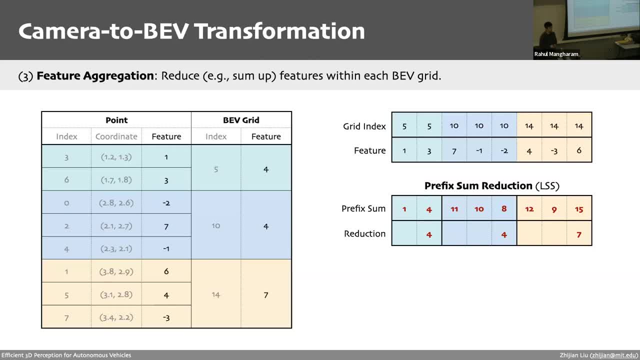 And now go ahead. I thought it's, it's quite implemented, like efficiently, this influence is efficient. but if you think about it like different outputs actually have the dependency, uh, between each other, right? yeah, if you want to get the prefix sum of the larger avenues here, you need to first get a result before, so you need to do a tree. 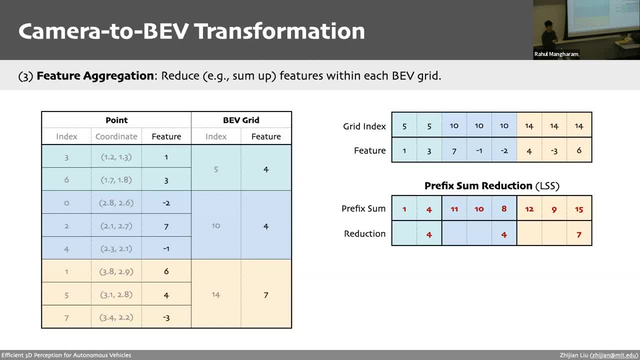 reduction. so that's actually not. so it's not as efficient as, for example, just doing a sum. that's true, yeah, and also, if you think about it, here there are a lot of unnecessary elements generated, because what we only care about here is those prefix, some values at the boundary. so 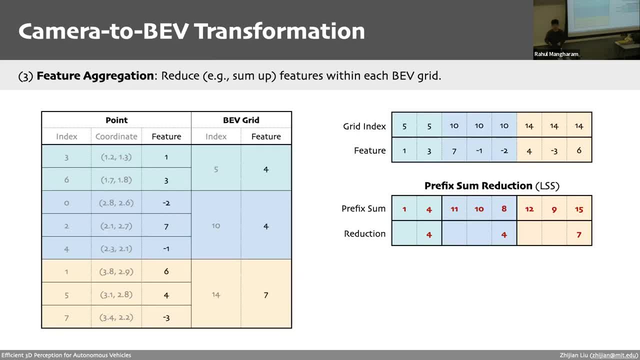 we're actually generating all of them just to support us, to get all the like the prefix sums at the boundary that we care about. so the way we accelerate it is also very simple. so we just write a specialized kernel. so the basic idea is we assign a gpu thread to each of the grid and then 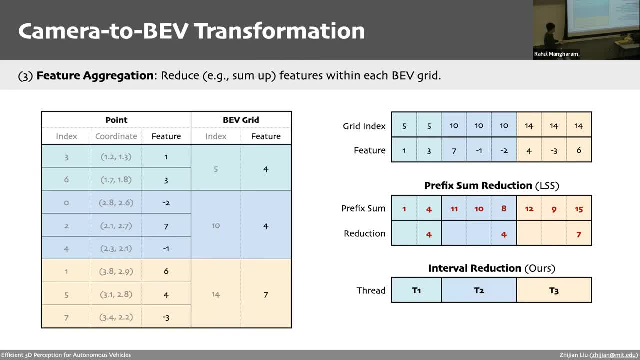 within each grid. we just do an interval reduction and then write it back to the, to the gpu. so it's very simple but turns out it's actually very effective because it removes the dependency between different output values and also it does not require these like unnecessary value computation right. 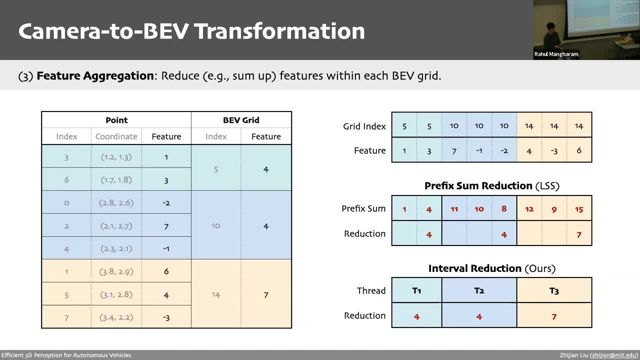 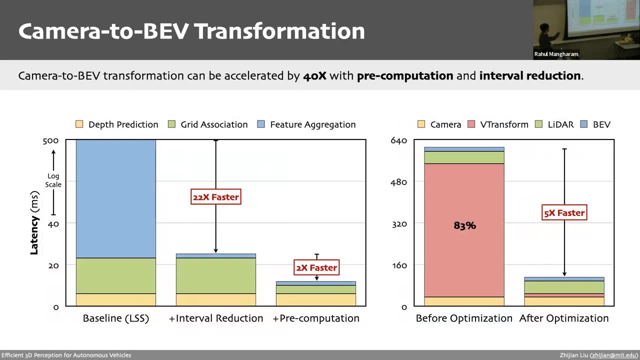 so this optimization step can accelerate the whole process by a factor of 250 meters. initial camera to bird's eye view transformation step took around like 500 milliseconds. here with the interval reduction it can be accelerated by a factor of 20, two times and then further with the pre-computation. this step is optimized by another factor of two. 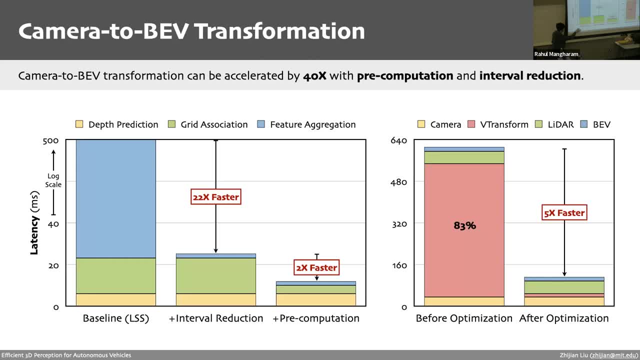 so you can see originally like for the view transformation. so the right hand side is the engine breakdown, latency breakdown of the billion fusion model. so 83 percent of the total runtime is actually spent on the view transformation process. a clear bottleneck. but with the list of optimizations we can reduce this part generally 12 percent, achieving a five times engine speed up. 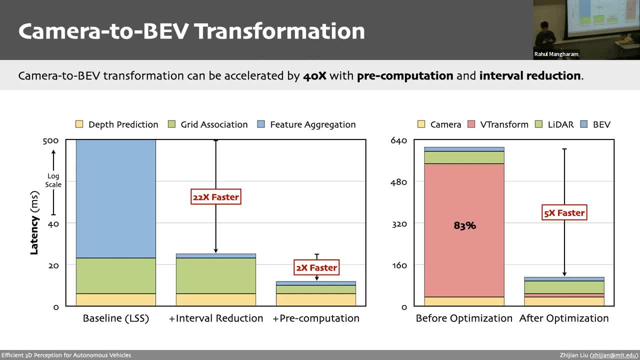 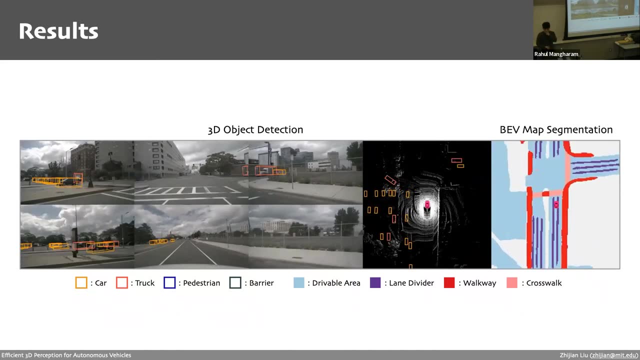 so this improvement is actually very crucial because, if you want to unify the multiple sensory into a like a unified bb space, this transformation is actually a key operator to to to achieve this. so now let's move on to the evaluation part. so here's the demo of 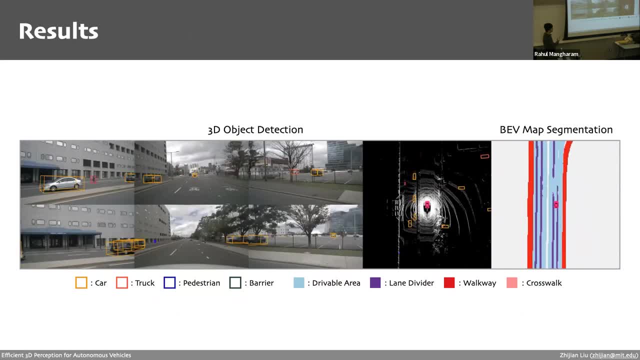 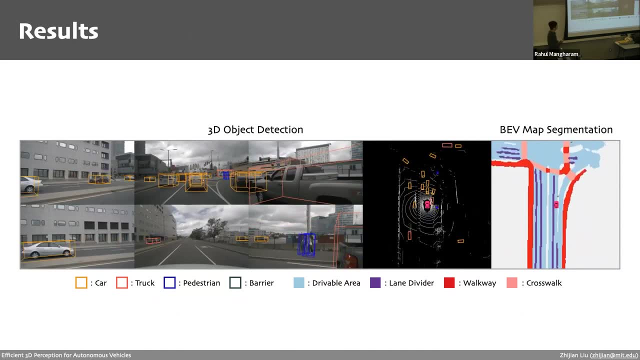 the fusion running on the new scenes for a 3d object detection for the bb max application. so you can see that, like the b, fusion is able to recognize different objects fairly accurately, even though it's like far away objects, and also the map sanitation results also clearly exist. 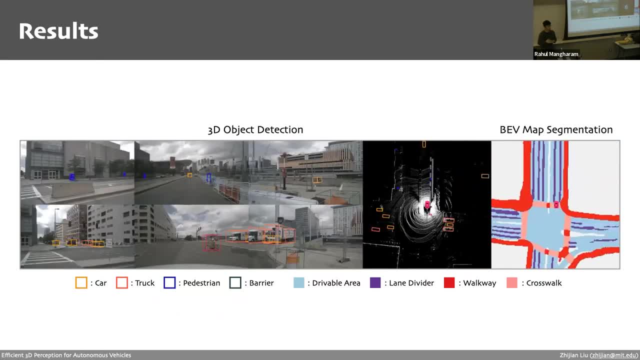 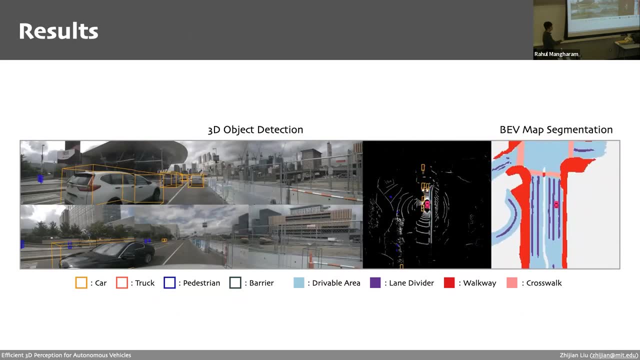 although you can see some blurry like before the intersection, but that's mostly because we don't really have the information at that region. there's some occlusion and a limited sensory coverage. uh, in some regions. for example, you can see the top right corner of this contract. 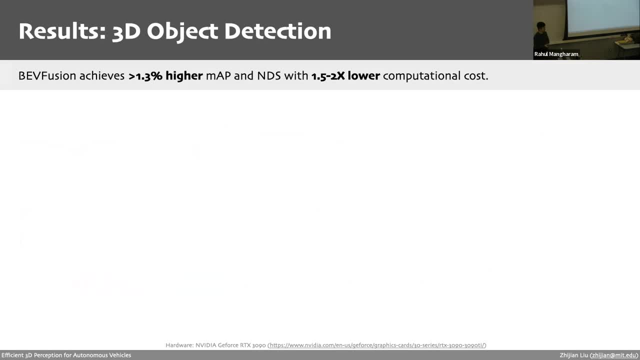 then let's take a look at the quantity of quantitative results of the 3d object detection on the new things. so there are a lot of numbers here. if we're looking at the numbers, let's first take a look at the metrics that we care about. so 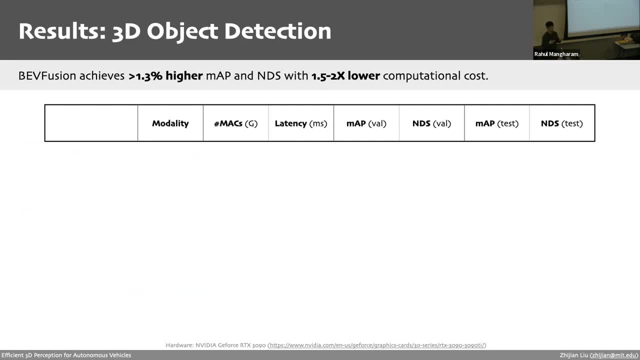 first it's the modality, basically which sensor? what are the sensory like inputs? uh, the master uses. and then the next year is the number of facts in the latency. so these two are the efficiency measures of the model. so the number of max is the power of moderate measures. basically counting the 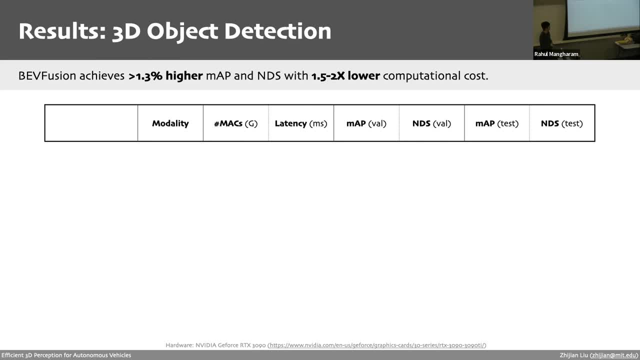 number of multiplied ads in the model and the latency is measured on rtx 390 gpu and the rest four. here is the map, nds on both validation and test that the map is the 3d object detection accuracy and nds is an aggregated detection score defined by the new things. 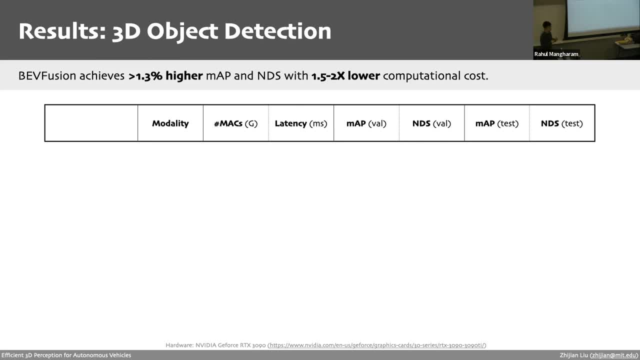 uh leaderboard. so it's kind of also uh care about curious about some other factors like attribute estimation and also the velocity estimation. so let's first take a look at the camera- only baselines and the light only. so one thing we can clearly see is that accuracy between accuracy of the lidar, only baseline detectors are much higher than the 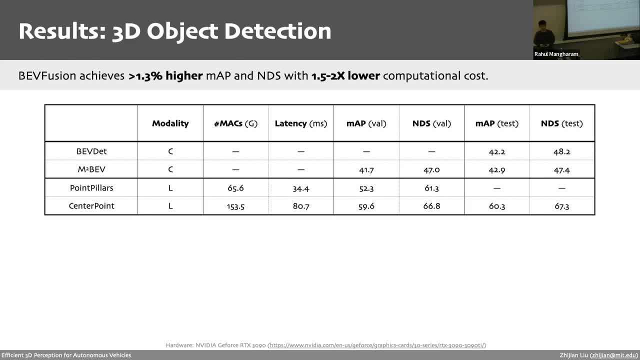 camera only presence. so the reason for that is the 3d detection is a task cares about the geometry of the scene and objects. you can directly get an accurate spatial like estimation from the lidar sensors. well, for the camera sensor it's actually very hard to get the spatial estimation. 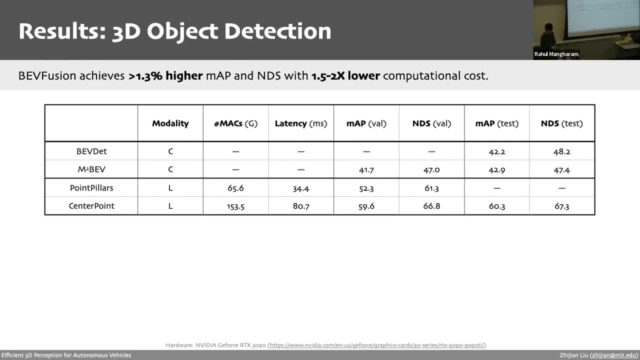 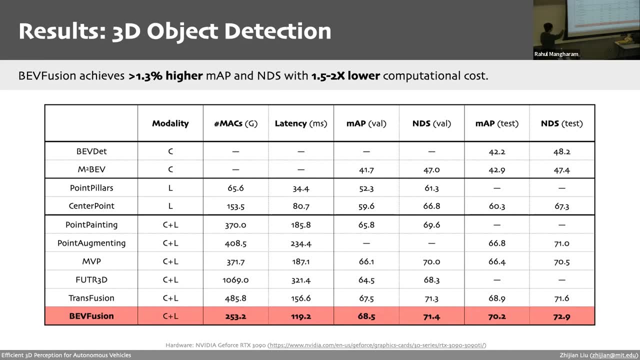 the depth estimation. so that's why there's a huge gap here. and then let's take a look at the sensor um methods. so we compare with the few representative sensor fusion lengths, with the point painting we have just introduced and some others like map filter 3d transfusion. 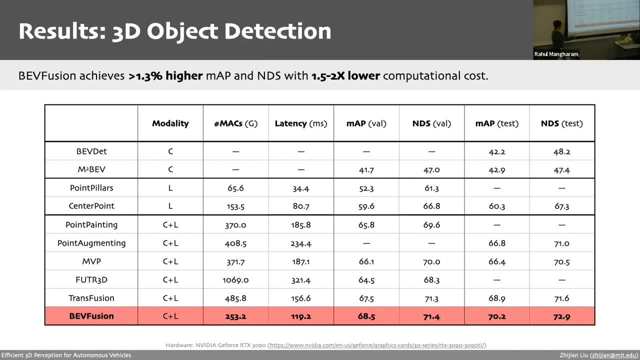 the one thing we can clearly see here is the sensor fusion method. that typically is more expensive, computationally expensive, compared with the lidar only, for example. you can see here the future 3d uses like 1t max, while for the center point the line only center point is only like 60. 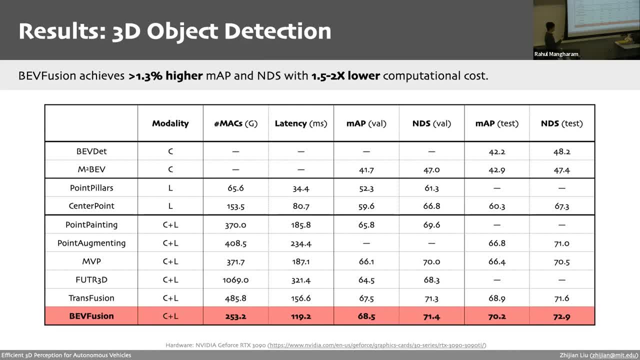 in comparison, our bb fusion is able to achieve the state-of-the-art performance while like actually being much uh, at least like 1.5 to 2 times uh more efficient than those on baselines. another another thing we can see here is compared to lidar, only baselines the fusion. 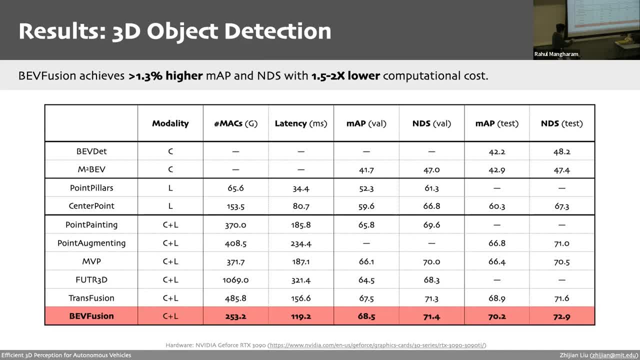 method like right that achieves a very high accuracy, uh large accuracy improvement around like 10 percent um on the validation set and more than 10 percent uh around 10 percent- on the test set as well. so i want to understand where these improvements actually come from. so here we study some like the performance of uh, our b fusion, the lidar only. 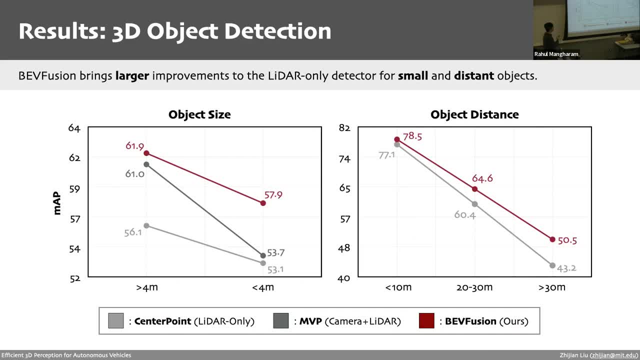 baselines, the baseline center decommasses and there are different object sizes and object distances. but one thing we can clearly see here on the left-hand side is that the bb fusion achieves a very consistent improvement over the lidar only models across different uh, across different object sizes, while for the mvp it only achieves a good 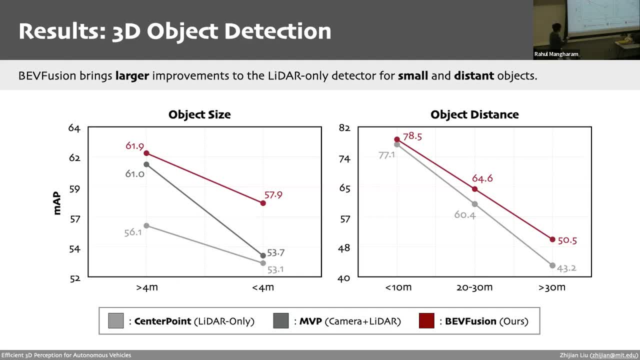 improvement for the smaller option, but for the larger objects, the, the improvement is actually very large. oh sorry, the other side, uh, the achieve a large improvement for the larger objects before the smaller object. the improvement is actually very, very marginal. and also for the right-hand side we can see, compared with the lidar only method, our bb fusion. 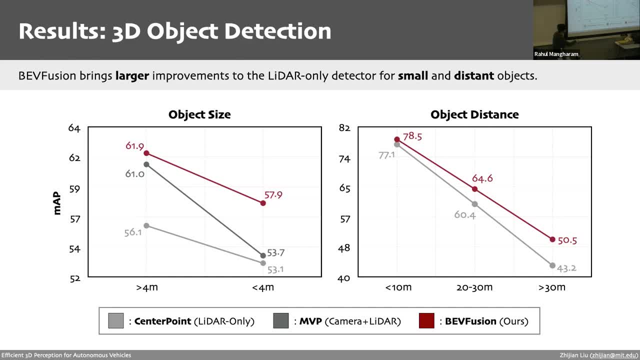 a much larger improvement for those objects, uh, that are very far away, distant away from the, from the eagle car. that actually makes sense because the lidar has a very limited coverage, range coverage. so that's something can be improved by the, by the like dense camera information, so you can actually bring a much larger purpose. and then let's take a look at the. 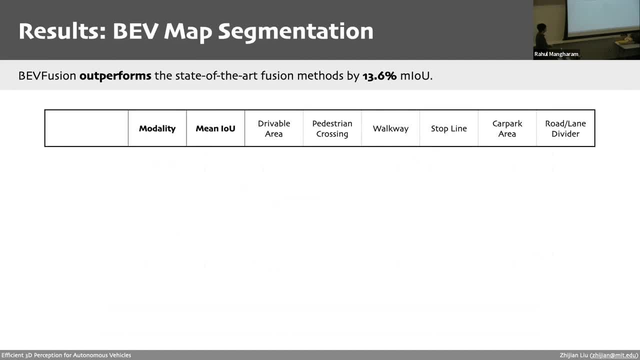 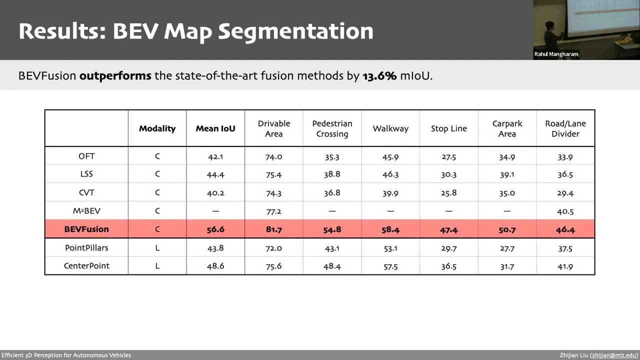 results of the bb map segmentation. so that's same. here we first take a look at the matrix. we only put about the mean IOU here and also the per class IOU scores for all these different semantic classes And the camera-only baseline, the LiDAR-only baseline. So we actually have a better camera-only. 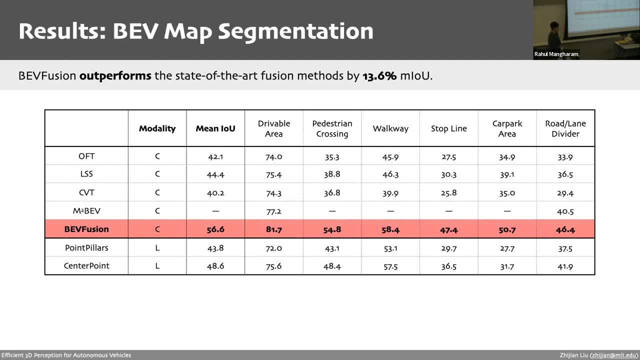 baseline already. The bbfusionc is a camera-only version of our bbfusion. It already achieves at least half percent higher MOU compared with the previous camera-only baselines. Well, one thing that's very interesting here is you can see the LiDAR-only method. 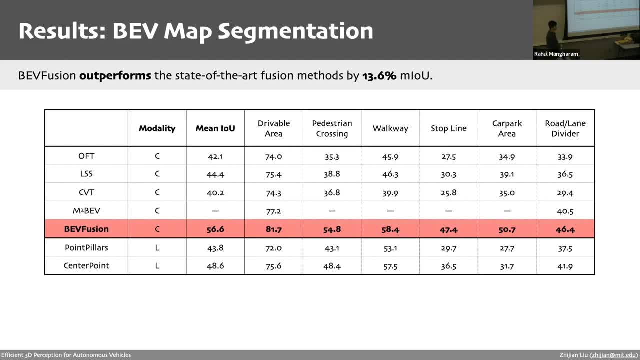 performs much worse than the camera-only model. That's directly the opposite from what we have just observed on the three objects. So the reason for this is the this task is more about the semantics rather than about geometry. So this is actually what this type of information is, what the 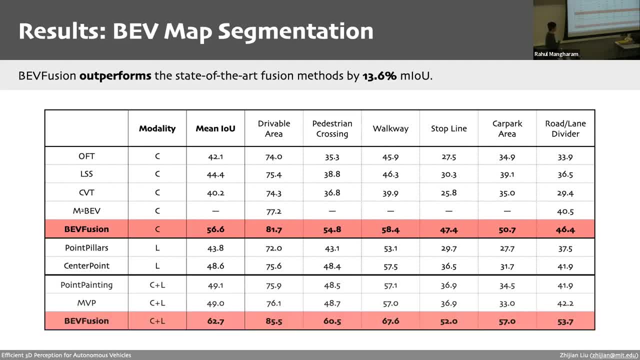 camera can help the most. And then finally the fusion results. So compared with the baseline, the point-picking and linking, they mostly just care about the objects. So that's why they don't really have much improvement compared with the LiDAR-only baseline- here Very marginal improvement. 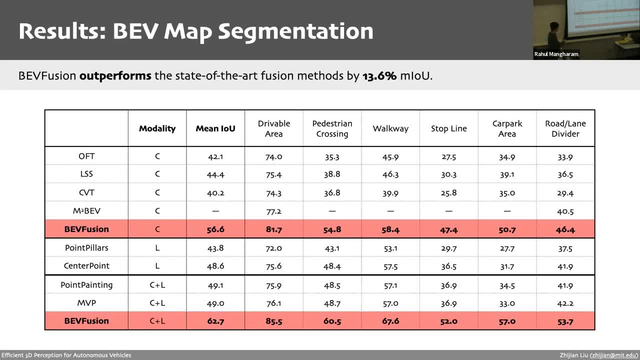 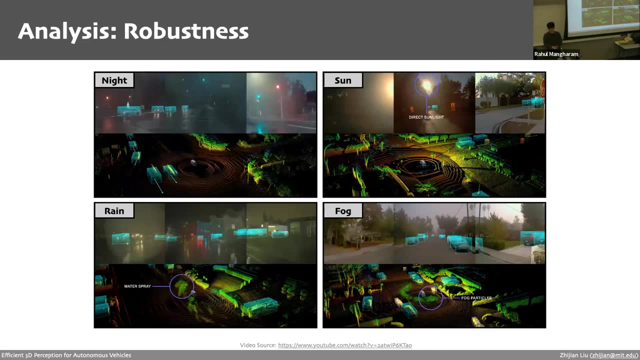 around like 0.5 percent, while bbfusion achieves a much larger improvement, around six percent, over the strong camera-only baseline. All right, so that's enough for numbers for now. So let's take a look at how robust our execution model is to different lighting and different weather conditions. So because 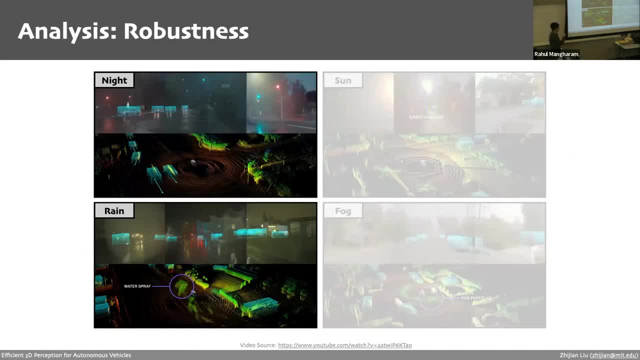 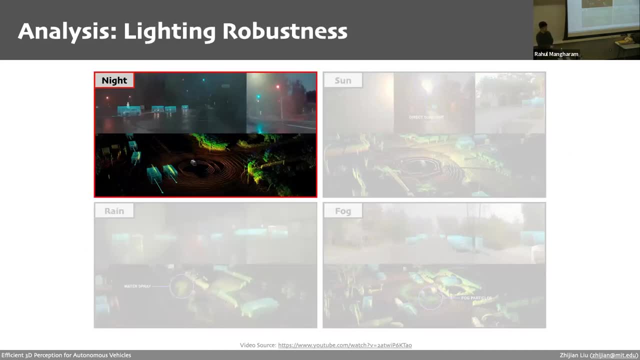 of the limitation of the NewSynX dataset, we can only test the performance under the nighttime, the daytime and the rainy days and the sunny days. Let's first take a look at the lighting robustness. The poor lighting conditions are very challenging for the camera-only models because 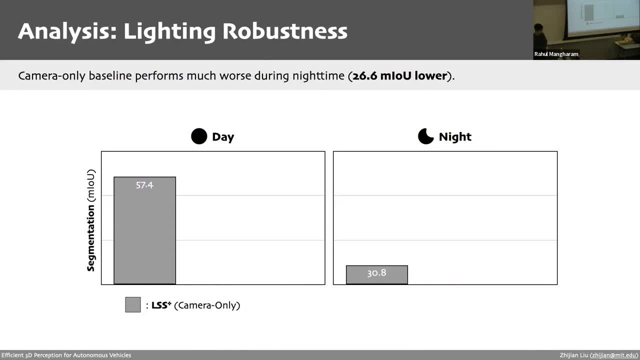 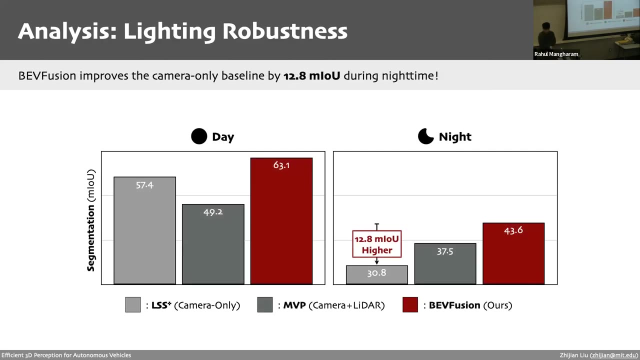 camera provides less information during the night. So the camera-only LSS, so the camera-only baseline here, performs much worse during the nighttime. It actually has a 25 percent- at least 25 percent- MLU degradation, While with the fusion, with our fusion, the bbfusion can significantly 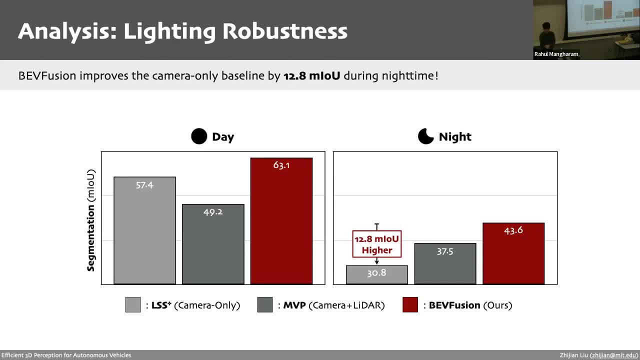 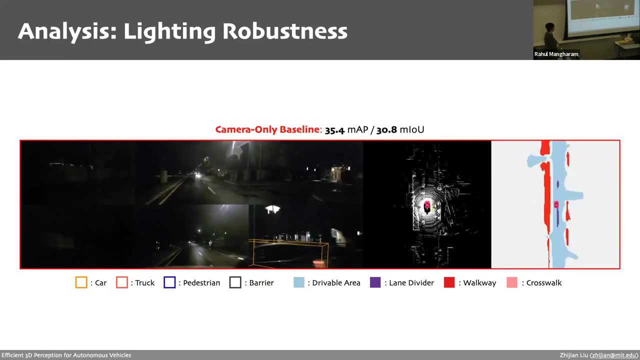 boost the performance by about 13 percent, which is the improvement is actually even larger than what we got for the daytime. So this actually demonstrates the significance of the geometric clues when the sensor, camera sensor fails, And this is the visualization of the camera-only. 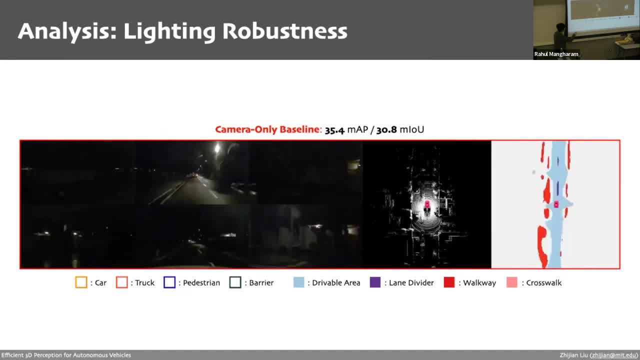 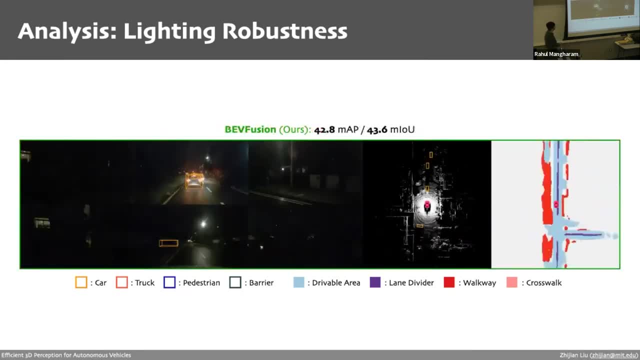 baselines during nighttime. You can see it cannot like recognize the objects, like the faraway objects here, and also the segmentation quality is fairly poor, While our bbfusion is able to recognize much more objects on the, on the data and also the segmentation quality is much. 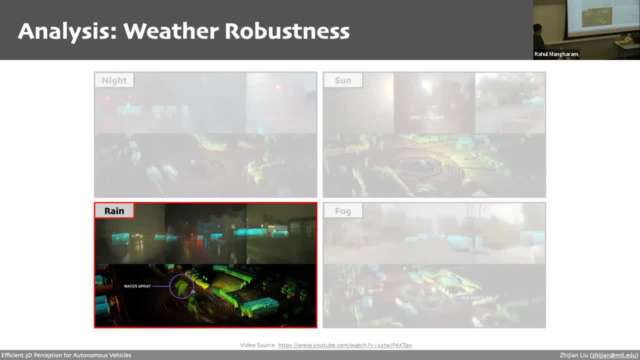 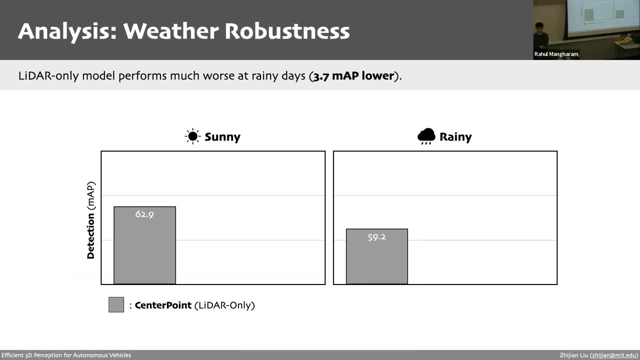 better. And then let's take a look at the results in the different weather conditions. So detecting objects in the rainy weather could be challenging for the LIDAR-only method because of the like the sensor noises during the rainy days. So the LIDAR-only detector's central point- here you can see. 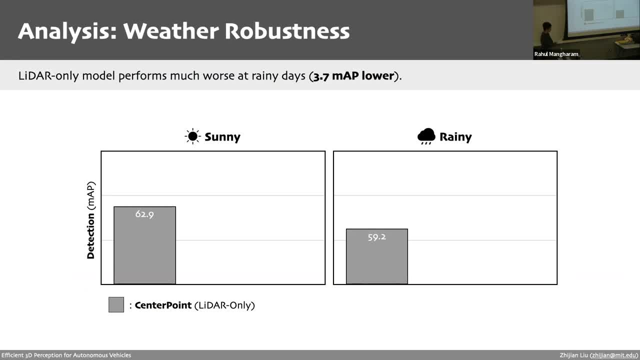 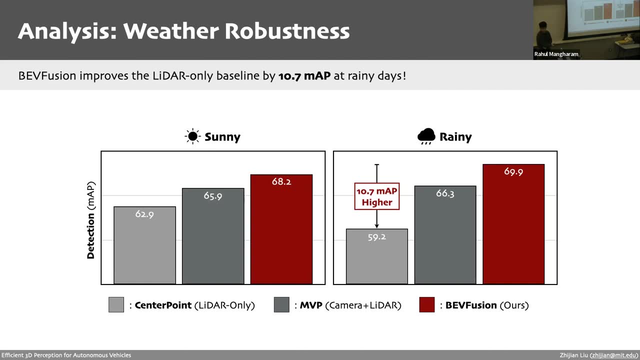 and that's the right 4 percent accuracy drop compared with the results during the sunny days, Although with the bbfusion you can see it improves the center point by 10.7 percent, actually achieving slightly better accuracy than the sunny days here. So this is because 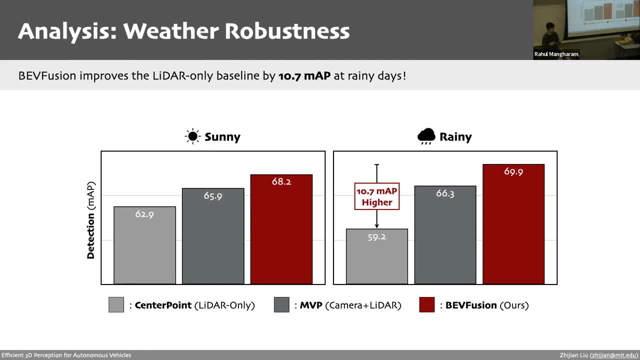 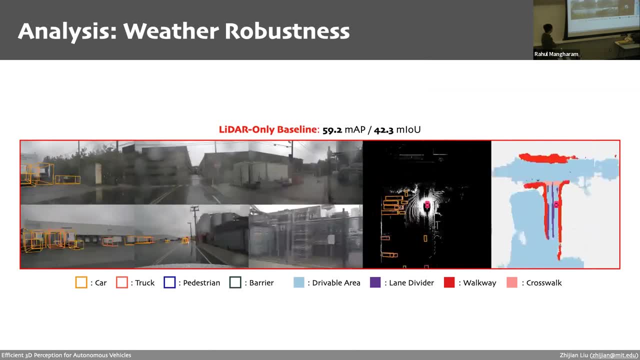 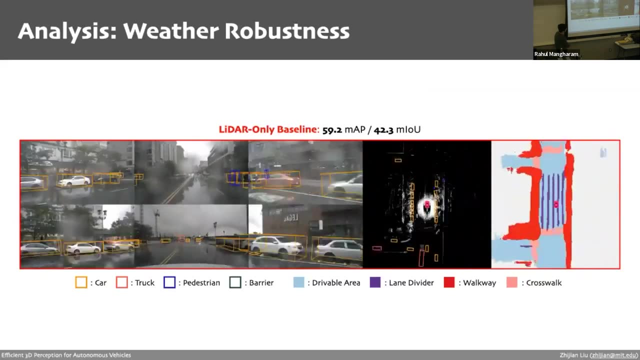 the camera is actually very robust to different lighting conditions, so adding this information to the fusion model can help a lot. So some visualizations here as well. So there's a LIDAR-only baseline. The segmentation result is clearly very blurry, and this is our result. So 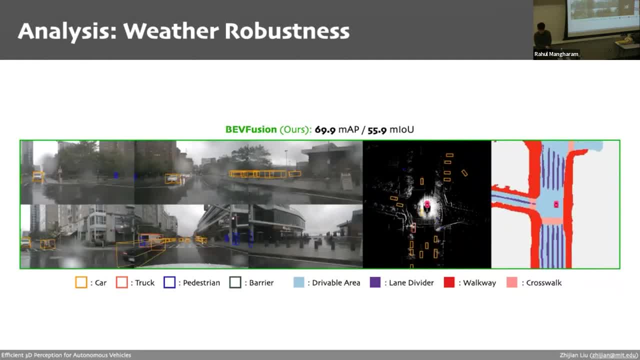 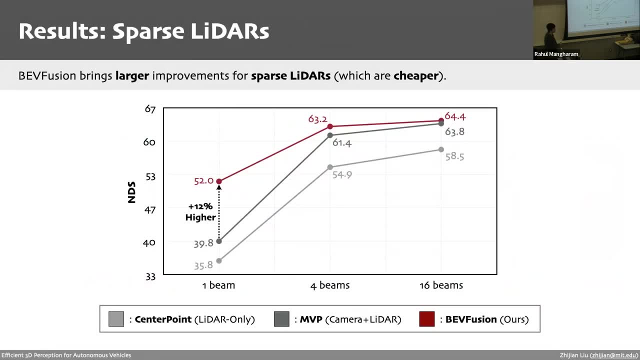 you can see the lane dividers are much clearer here And also we study some effectiveness of our bbfusion under like sparser LIDARs. So the reason why this setting is very interesting is the sparser LIDARs are usually cheaper, so it can be actually deployed like more deployable. 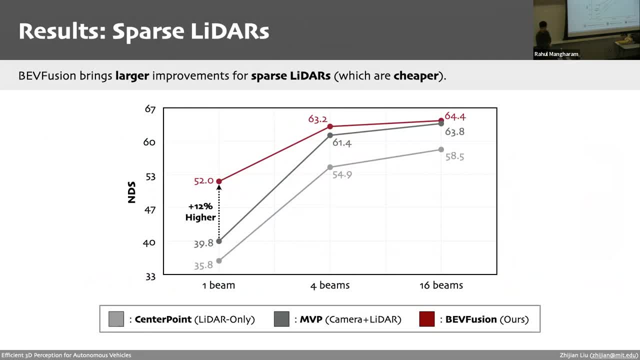 or affordable on the cars. So, for example, a four beam LIDAR consumes for around a thousand dollars, while for the higher end of like LIDARs they can be much more expensive. So bbfusion brings a much larger improvement for the sparser LIDARs, For example. 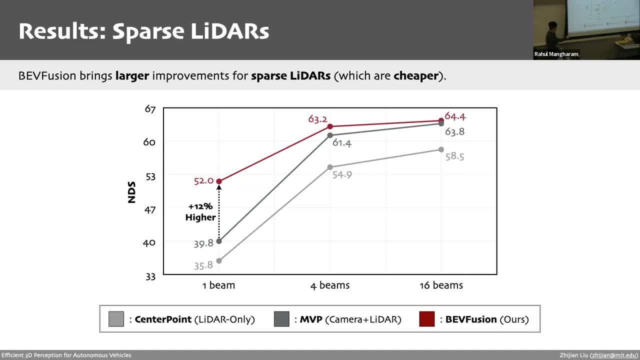 for the one beam, LIDAR. here the improvement is around 12 percent compared with MEP. It makes sense because the LIDAR is very sparse. right The point painting or point decoration will drop almost all the camera features, which is clearly not optimal. 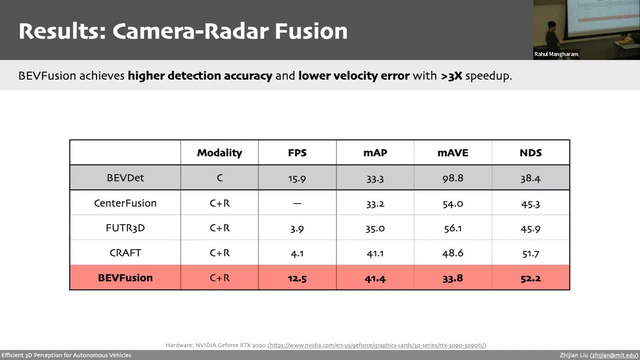 And radars can be seen as a sparser variant of the LIDARs. So we also did some analysis on the radar camera, radar fusion as well. So here the base signs are the center fusion, the filter screening and the very recently the recently talked about PRAPT. So you can see that, compared with these, 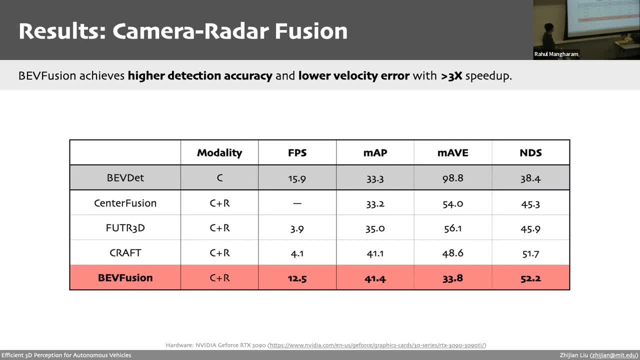 base signs. the bbfusion can at least deliver the same detection accuracy, which is the MEP here, and achieving much better velocity estimation. So here the MEP is the mean average velocity as an arrow, so it's the lower the better, and the MDS is the aggregate force. 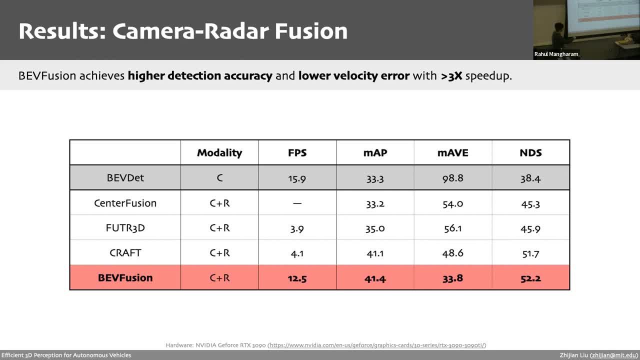 So you can see like the bbfusion can achieve this result with at least three times faster compared with the baseline, And recently we'll also try to accelerate this model using 10.0 RT. We can achieve around 40 frames per second using an existing model. 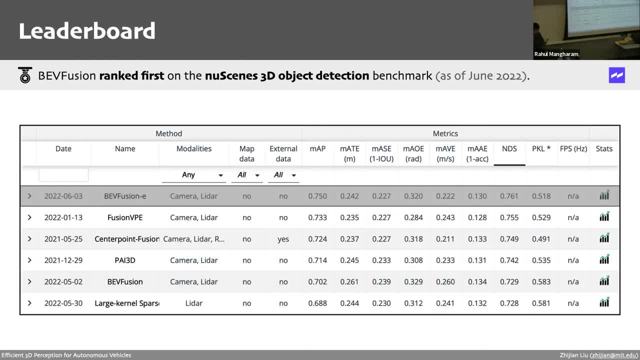 And finally, let's take a look at some critical results. so Mauritius YuSIN three-dimensional basal source, BNFusion measure, BV Fusion, ranked first on the NewSyncs 3D object detection as of last summer. So, as I mentioned earlier, 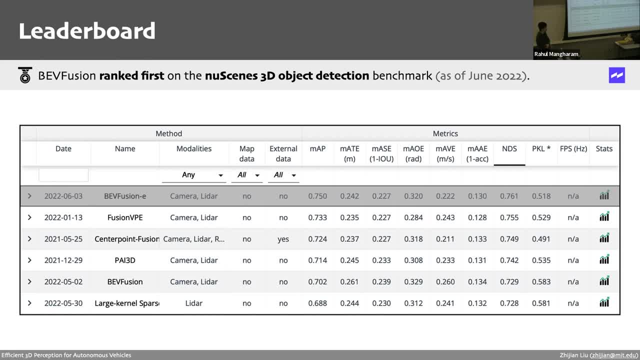 like this is a very fast evolving direction, so they're having a lot of works coming on the leaderboard in the past one year, But some of them are actually using very similar approaches as BV Fusion, some follow-up works, And BV Fusion also ranked first. 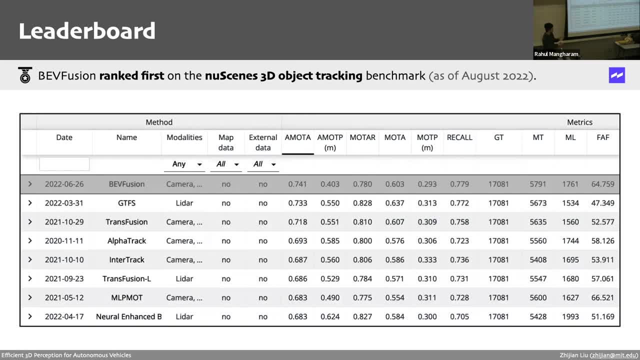 on the NewSyncs 3D object tracking benchmark. So tracking is one step further than the detection. So we not only want to detect those objects, we also want to associate the same objects across different prints. So this is actually very necessary for like doing motion prediction. 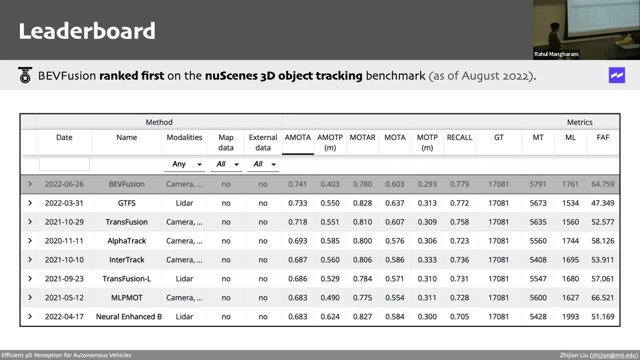 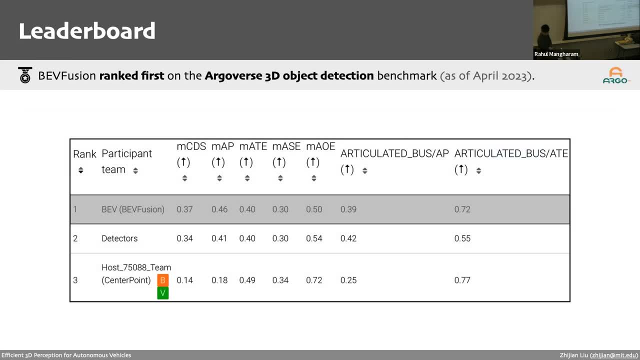 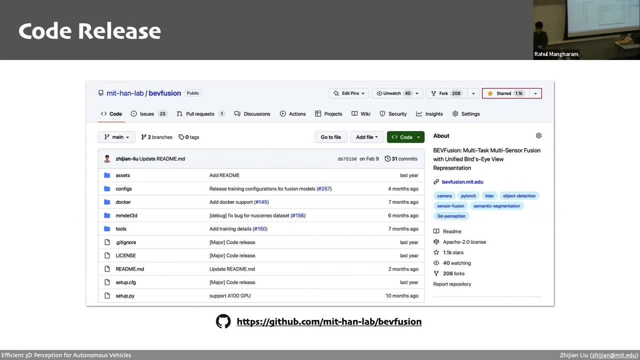 like even in the later planning series, also very crucial- And also on the WebMode 3D object detection benchmark, our global benchmark, And we have open-sourced the code of our BV Fusion on the GitHub, So it has received like 1,000 stars since its release. 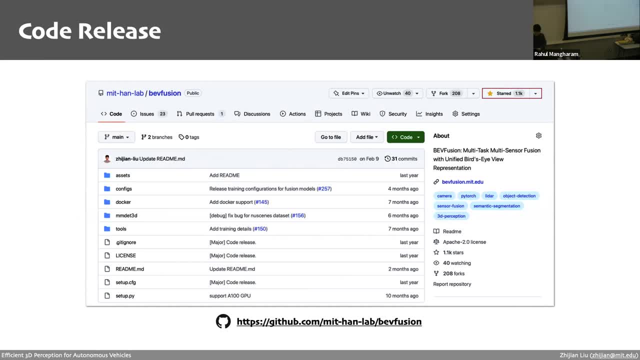 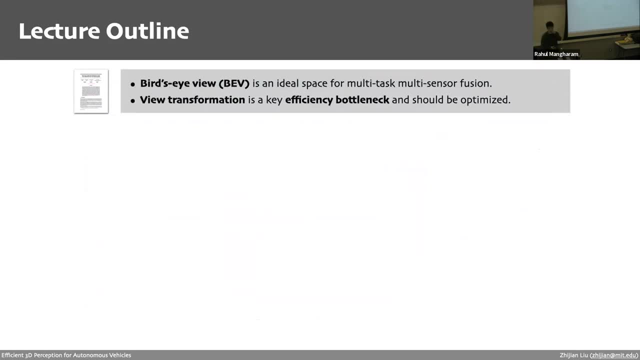 and feel free to check it out if you're interested. So that concludes the first part about the BV Fusion. So there are two main key takeaways here. First, the first ideal space is actually an ideal space for the multi-task, multi-structure fusion. 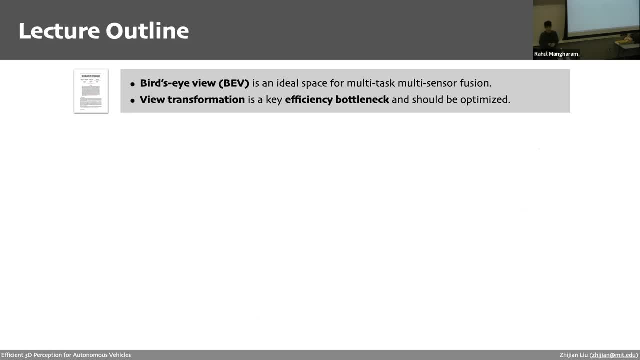 And secondly, the view transformation actually plays a crucial role in terms of the efficiency. It should be properly accelerated. And before we move on to the next part, I would like to pause a little bit to take some questions you may have. I just have a question on the prefix sum part. 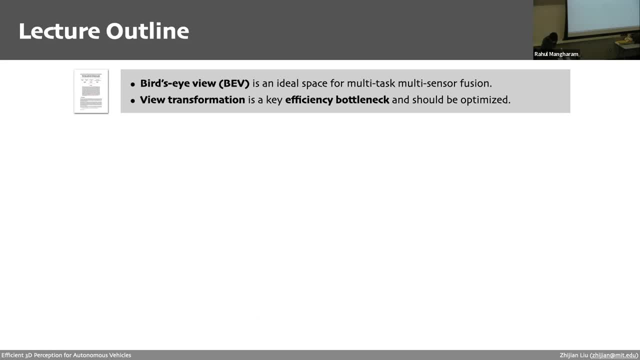 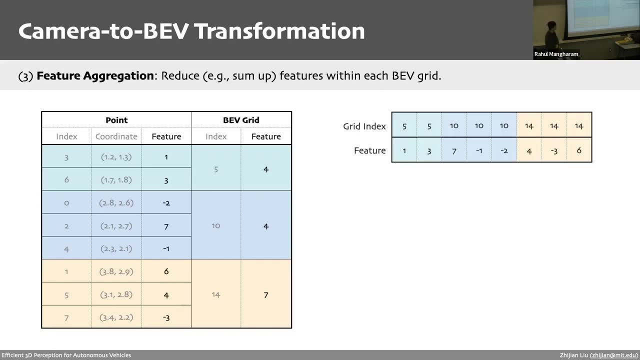 Okay, So if you write a kernel for each cell- basically right For each cell- then you have to make the cells equal length, right, All of them equal length to be able to run the purpose. It doesn't have to be. 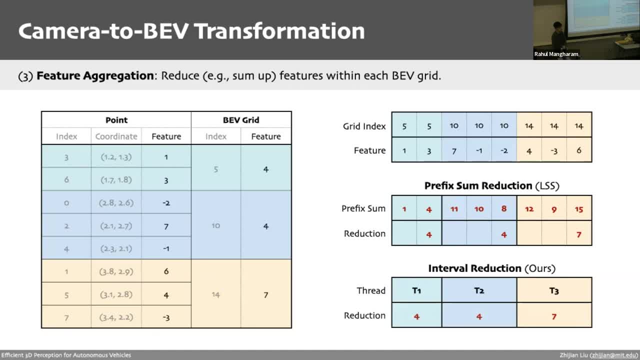 like some threads might like, finish the top of the. So you run it. if you push all of them to the GPU, you have to connect zeros when they're not equal. You don't have to. you just need to mark the starting and ending position. 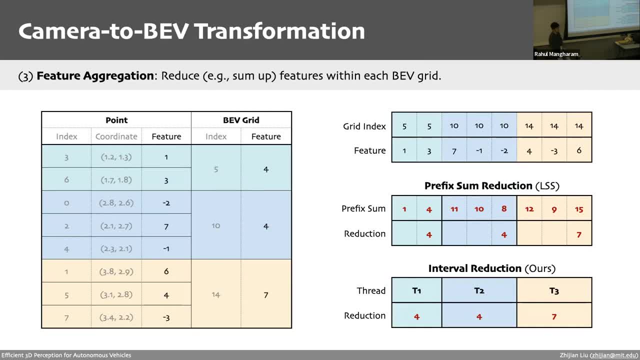 of each interval and then you can just assign the workflow to like each GPU thread. So for some GPU thread like your workflow might be lighter so it can finish like earlier. it's also fine. So it's kind of a volume effect by the interval that has the heaviest workflow. 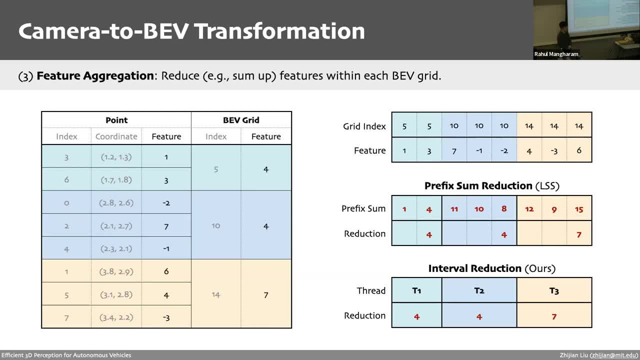 Yeah, So even if they finish earlier, they will still wait until the last one finish. That's kind of right, Like there are some other like optimizations we can do here. For example, it's highly in balance right. We can kind of move some of the 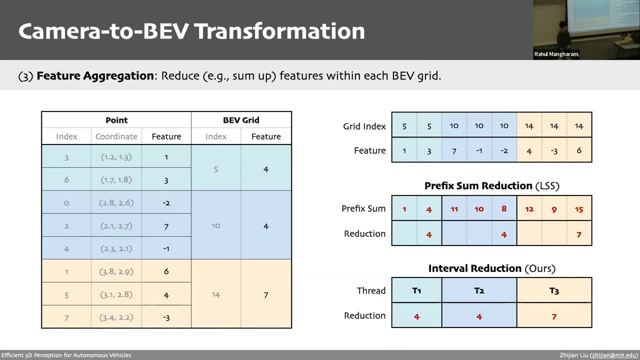 Oh, so you can push this one to this part, this one to this part, But we haven't done that because, like, in reality, like the, actually it's fairly equally distributed. yeah, So it's kind of like we don't have to do this. 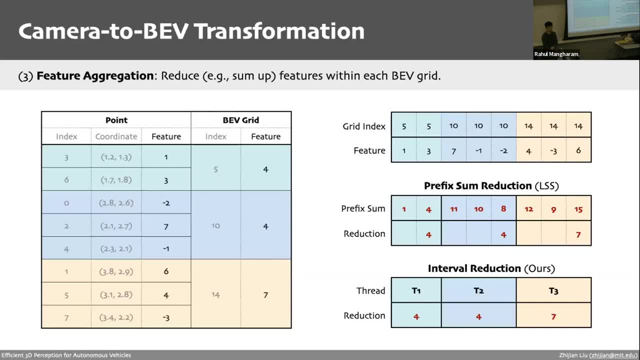 We can just do it like this, And then we can just do it like this. So it's kind of like, if you have an example of like a, let's say like a- you know you have a like a, you know. 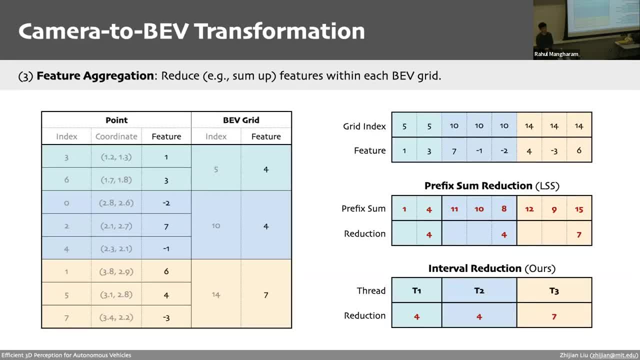 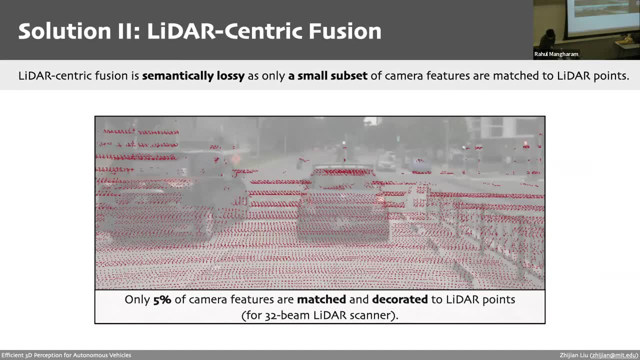 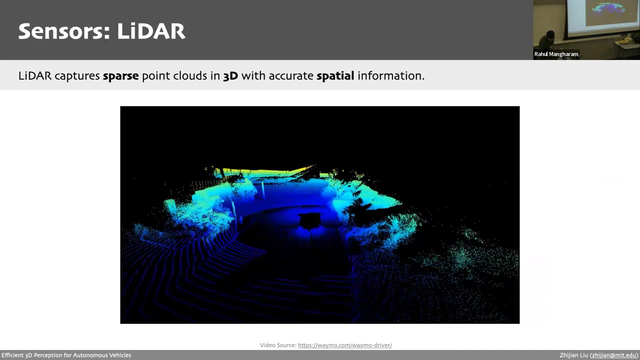 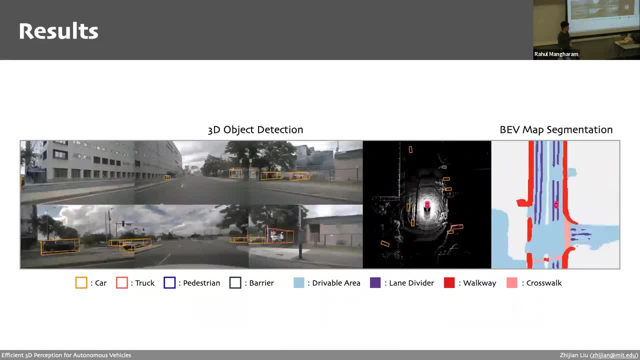 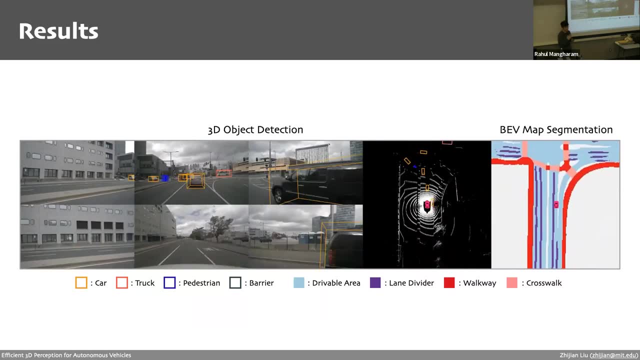 we just generate 3D boxes. So for each box you have the 3D positions XYZ, you have WHL for the 3D sizes, you have orientation, the heading orientation, and also you have the velocity prediction For the big snaps. 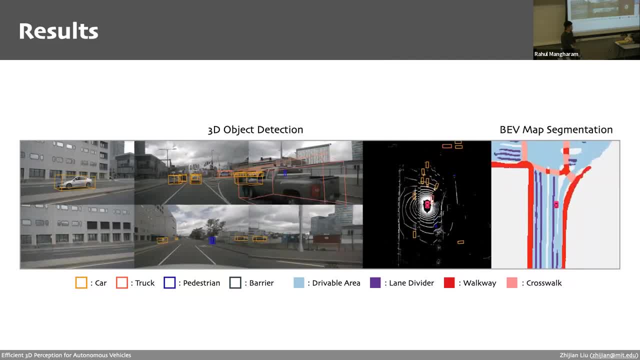 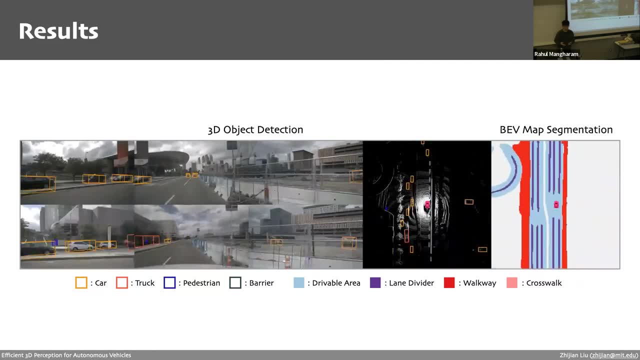 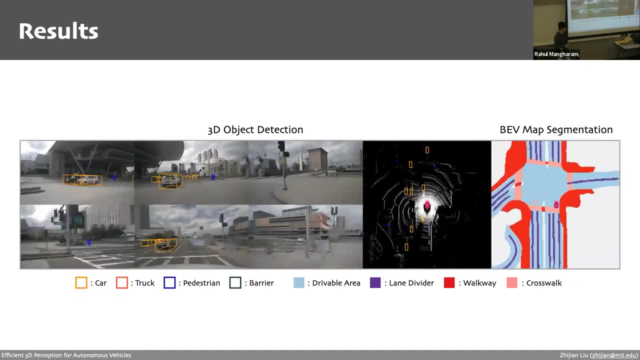 orientation is basically generating multi tasks, like prediction for each of the pixels here, For example, for each pixel. here we'll generate a probability vector over like, let's say, different classes, and one for each semantic class. how, how do you know the, the velocity of the? 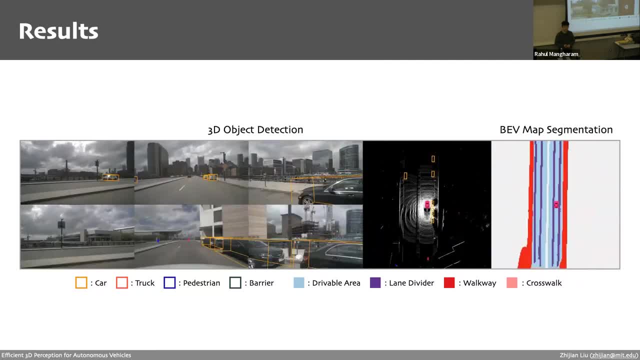 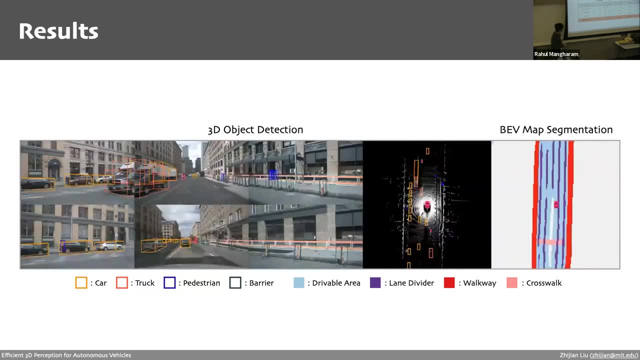 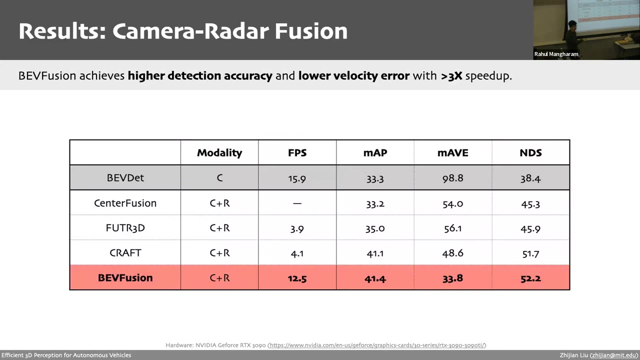 objects. are you combining multiple frames together from from the sensors or is that fusion happening and it's separate? yeah, that's a very good question because you can see here it's a camera, so you can see it's because obviously activation average is very large, so the fusion here is like 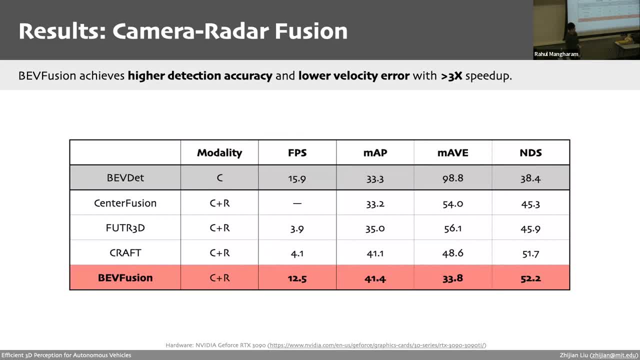 a centimeter per second, so it's like one meter per second error, like it's a very large um error because it's a single frame model so you cannot really estimate the velocity uh from the single frame camera model. it's basically guessing uh the velocity based on the task uh the radar can. 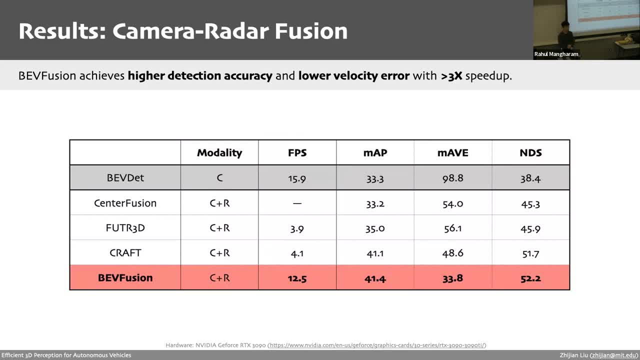 directly provide the velocity estimation. but for the camera, lidar, camera line of fusion models, because we usually use like a 10 frame light on aggregation, so we'll map the light out of an previous frames and transform it into a current warning system and just like use them together. 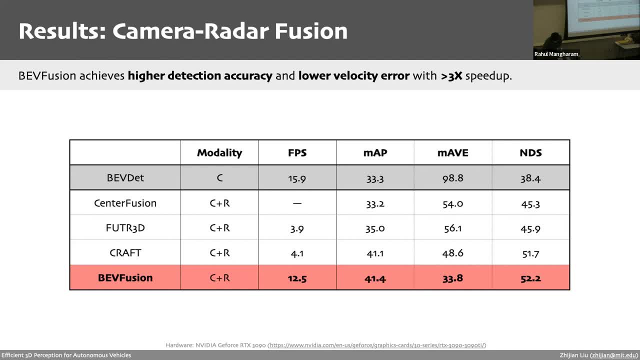 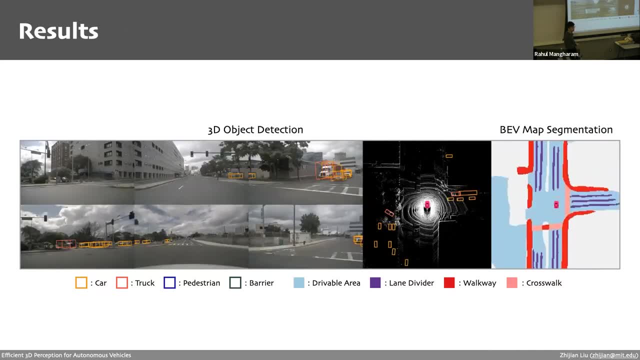 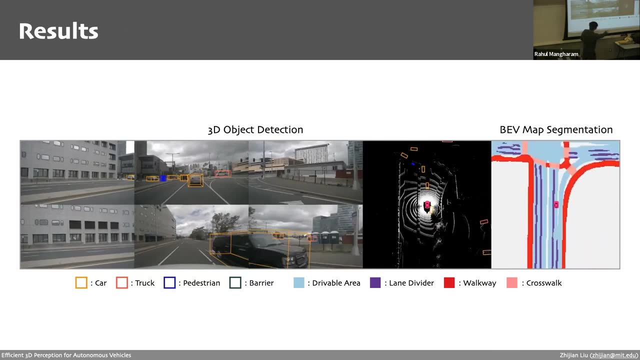 so we'll also have the information. so one thing we can see here. oh, that's okay, that was the reason why you have this carved image with the red dots. there are multiple red dots for each beam. yeah, yeah, that's right, you can also see here. there's a trace here, like behind the top. 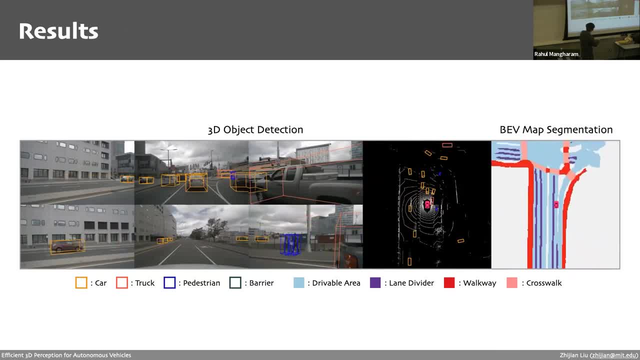 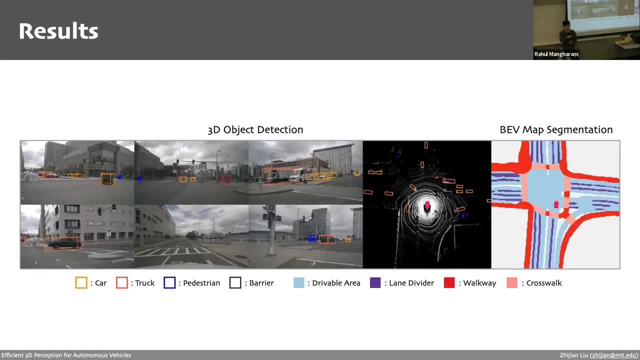 when it's not moving, you cannot see it right. but as long as it's moving, you can see the translation. yeah, i see it. yeah, because there's a trace here. that's because we're aggregating the data point cloud from modeling the french, you get it, but if it's not moving, 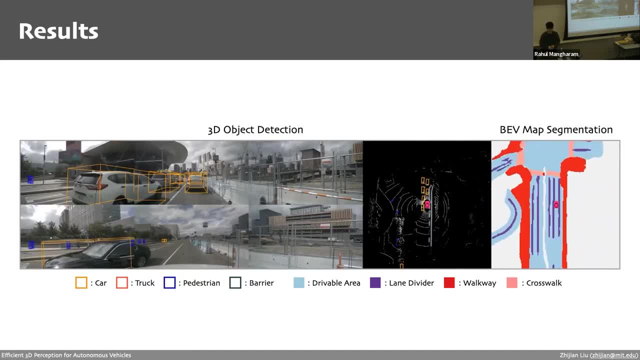 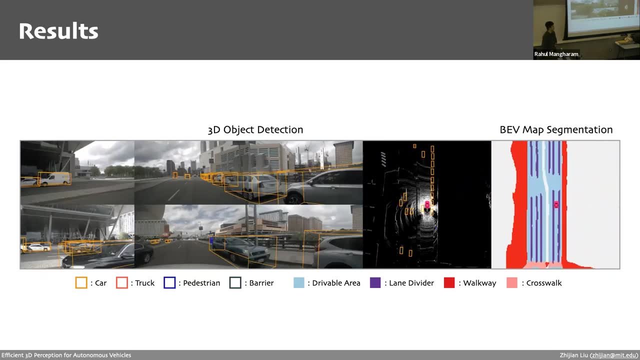 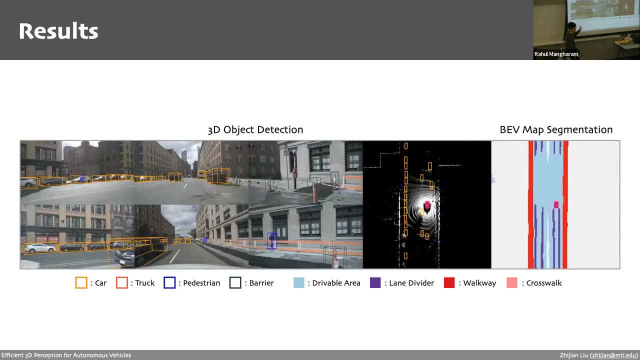 then you're actually stacking the same point out over and over right. are there any other questions? how long does it train from android? uh, the training pipeline is actually a little bit complicated. we need to first uh portray the camera encoders and then we could portray the light on the model and then, like, use them together. so the camera model is also. 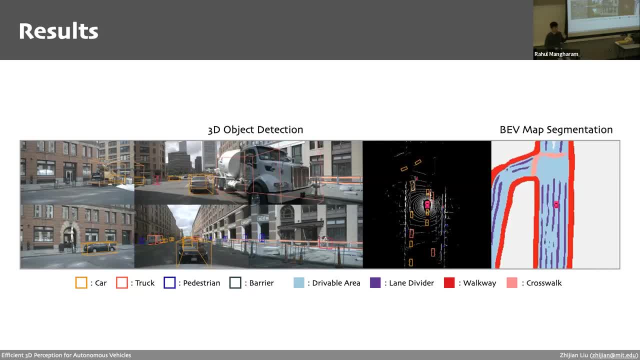 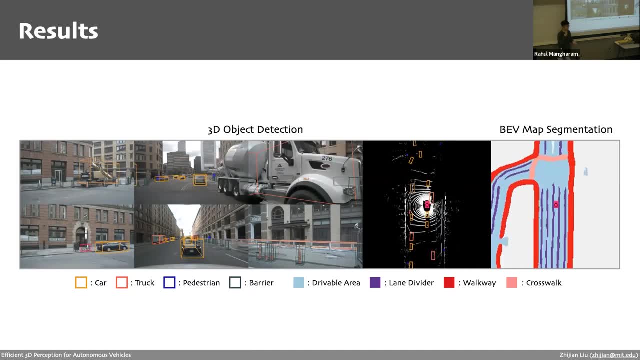 like these are like a few steps of your training, because if you want to get a good result and read it, what you do into like this, there's a lot of like complicated training, things like first portraying on the image net and on the cocoa and on the new images. yeah, a lot of steps in. 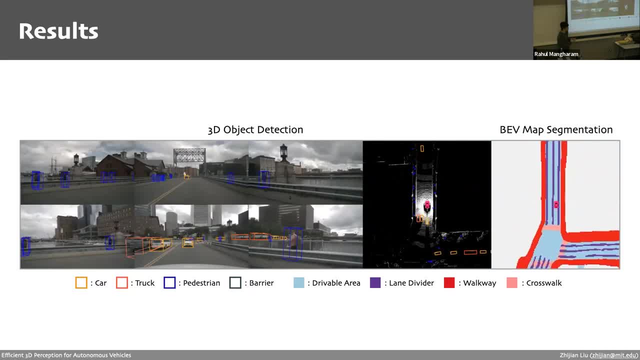 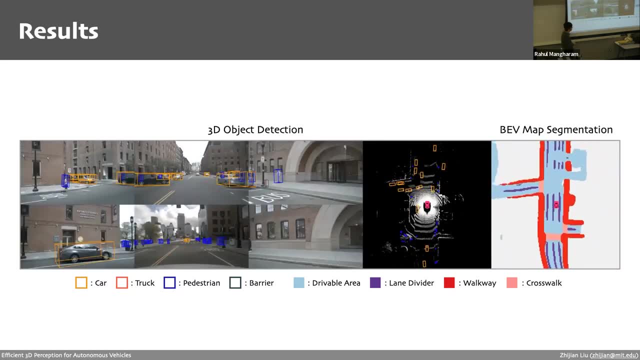 order to get a good result, but like i don't think this actually matters if you have a larger data set. so i would say, like in general, i mean this new scenes is already really large, because i mean i guess it's not that large, it's it's. 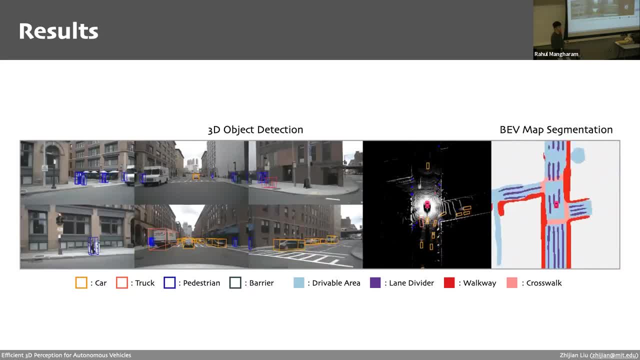 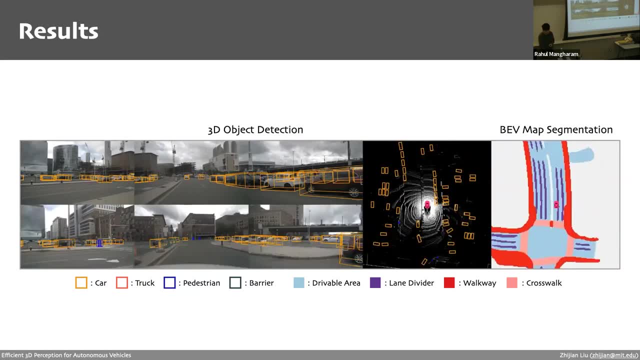 larger than some like data so, but like, for example, it's definitely smaller than yeah, so we have to go through all these between exchanges, but, like, in theory, i don't think these actually matter as much as long as you have a larger data set. i know, i know, but like, 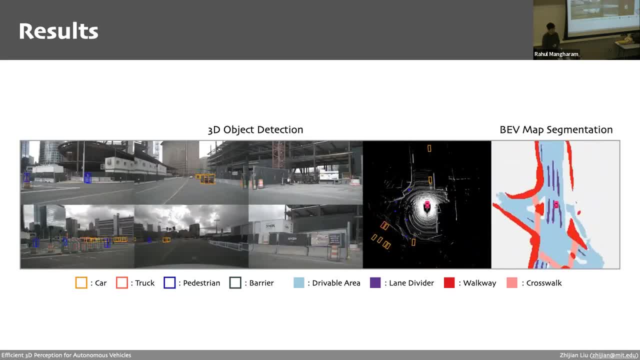 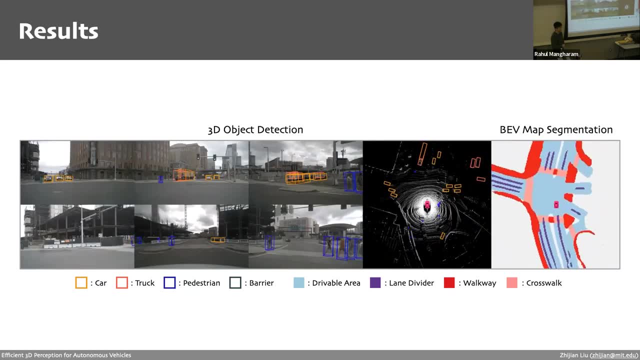 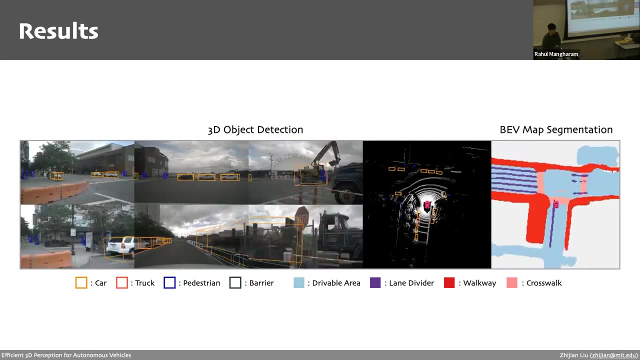 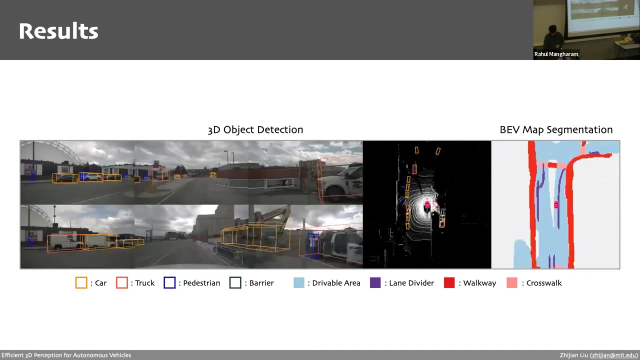 from a researcher point of view, i, i need to. we need to know how long to train, because so in total, it's only two to three days on the hgb. yeah, okay, are all the intermediate models fully convolutional, or are there model parts of the models? are they? do they have other architectures in them? let's go back to this. 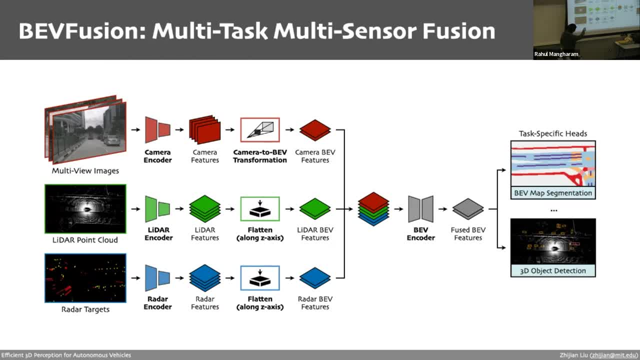 yeah, so so for the for the camera encoder, here we are using mainly using extreme transformers, but for the camera, radar fusion, because that will be targeted deployment, so we're using rest of the three transformers are harder to deploy. and for the line encoder, here we're using a box on it. i 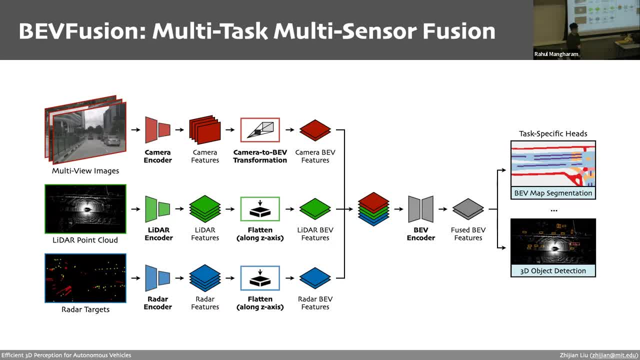 will explain what this box in the input. so it's basically a model composing of, composed with like sparse commutations and then the radar encoder. here is the point pillar, so basically a few mlps on each point top. oh, i'm sorry. and the bb encoder is just a convolutional neural network. 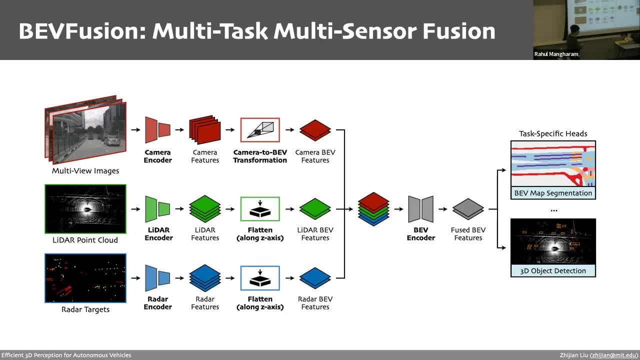 the other parts, i don't think. yeah, they're mostly, mostly like non-prime derived, so so, in principle, nobody. if someone wanted to retrain your bb, they wouldn't have to retrain a new model from scratch. they could use your weights exactly. it's better to have accurate. 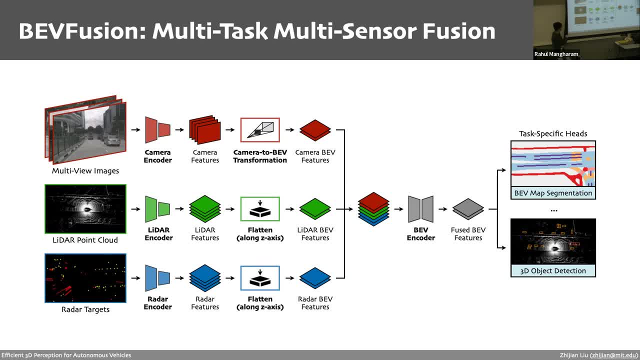 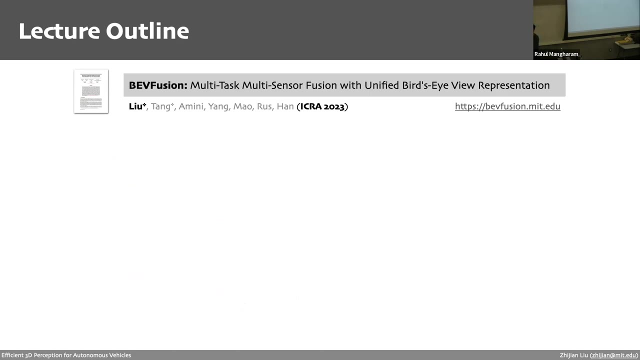 and lose the camera between the weights and portraying ways and also the line of the tools so you can directly reuse. all right, and let's move forward to the second. sorry, so i have a kind of amateur question, which is for this bird's eye view fusion. what about? 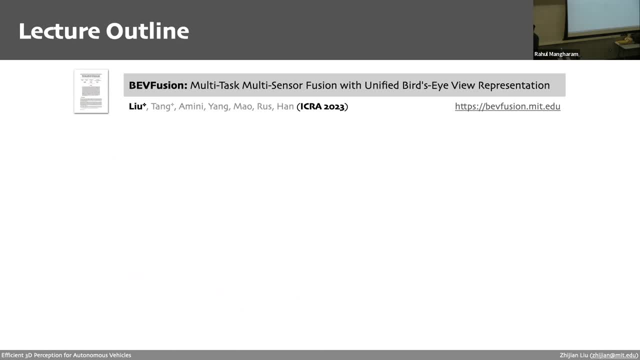 thinking about the case that the car is driving on the road, which is have a drastic change of raw and each channel is. this also works in your algorithms, because most of the intenses you're using in the slides are just the city cases where cars but actually the rock, the road, is just a plane. yes, it's really. 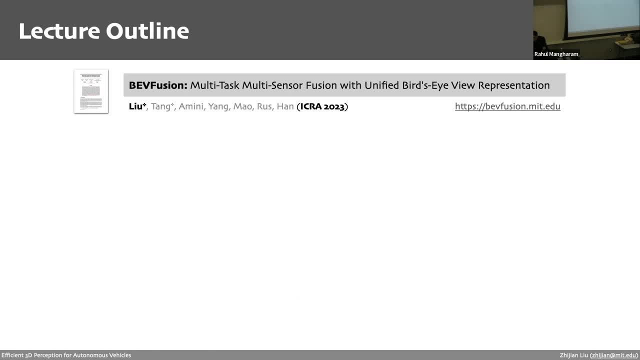 kind of right. there's the other things. yes, like that right. yeah, that's a good.